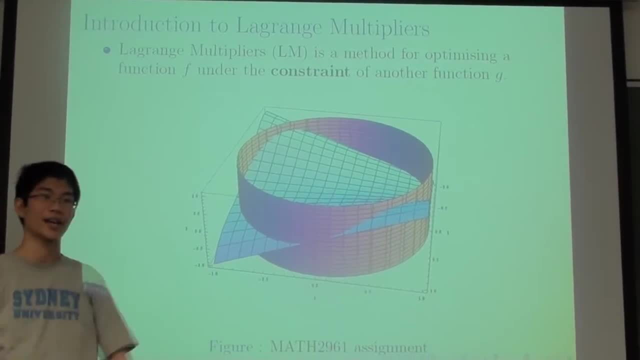 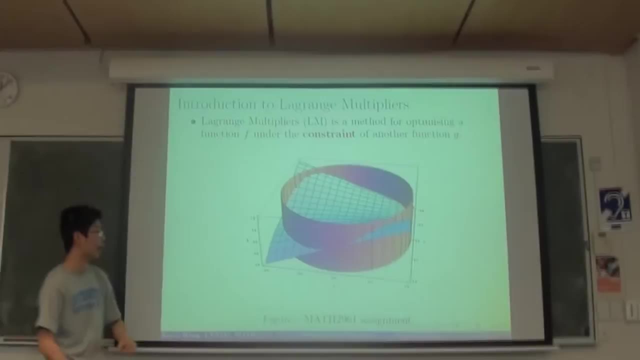 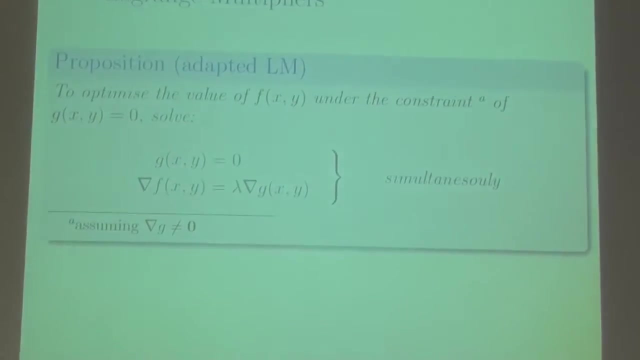 to find is the maximum or minimum point within a domain. That domain you have is the constraint. The function you're trying to maximize is, of course, the surface, And we'll actually look at how to solve this problem in the watch multipliers. 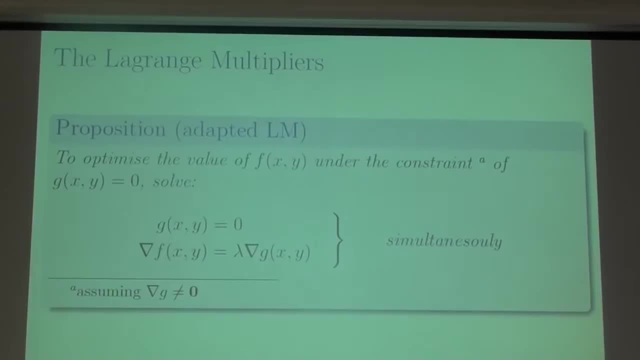 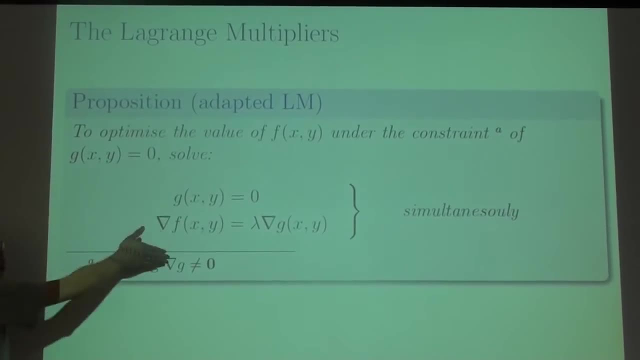 So here's actually the statement of the theorem itself, And the theorem simply says that well, if you want to optimize f on a constraint of a g of x equal to zero, then you have to solve these two equations simultaneously to find the optimized or the constraint of optimization points. 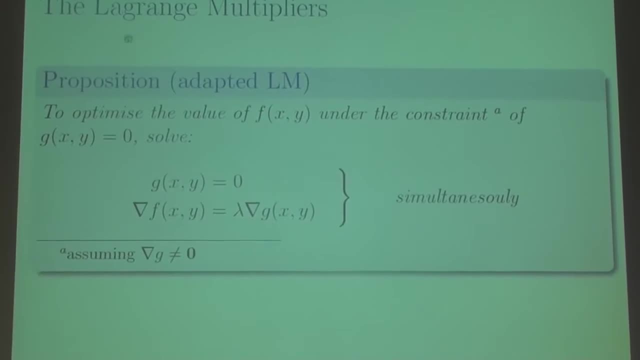 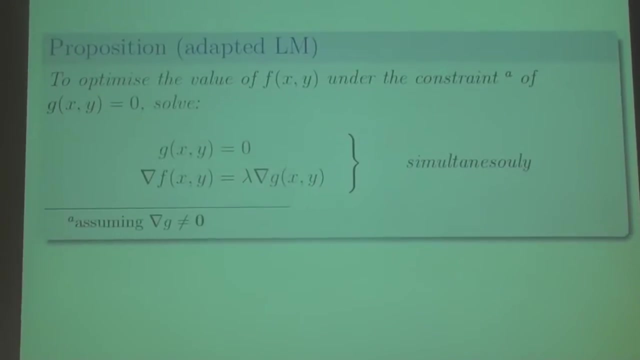 So the first: you can think of these two, two equations as being criteria for the, for constraint optimals. And the first criteria is not surprising at all, because that's our constraint. You know you always come back with a constraint, No surprise there. But 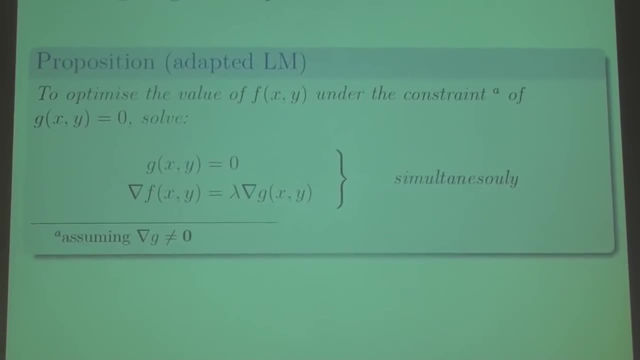 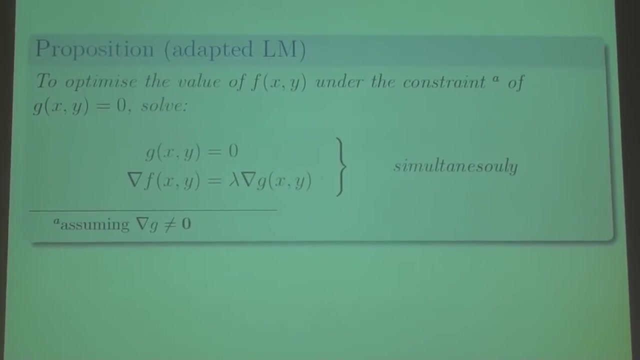 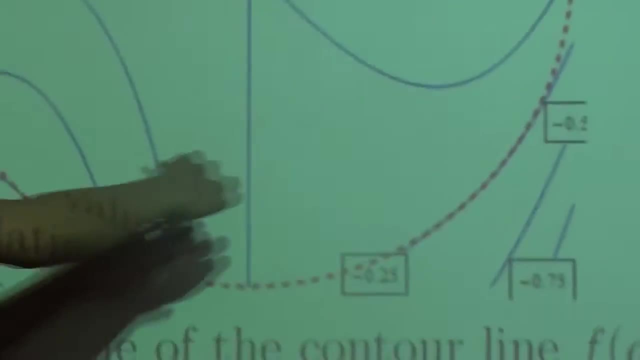 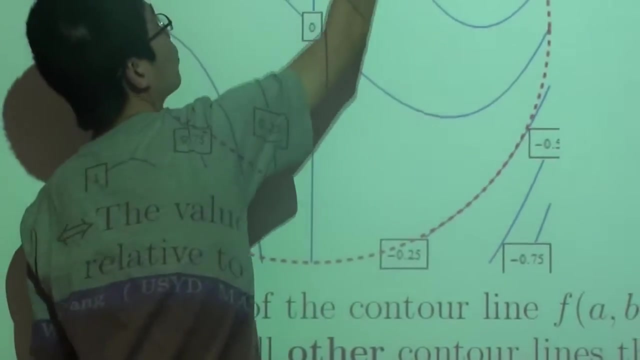 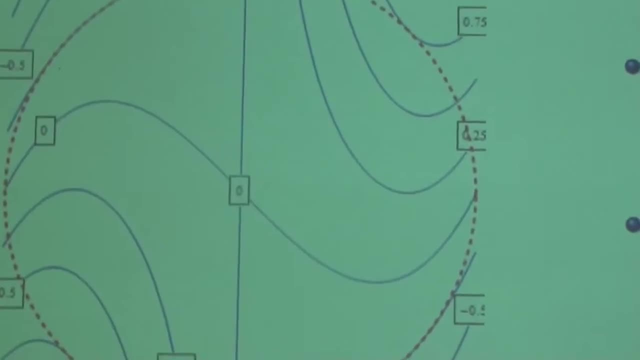 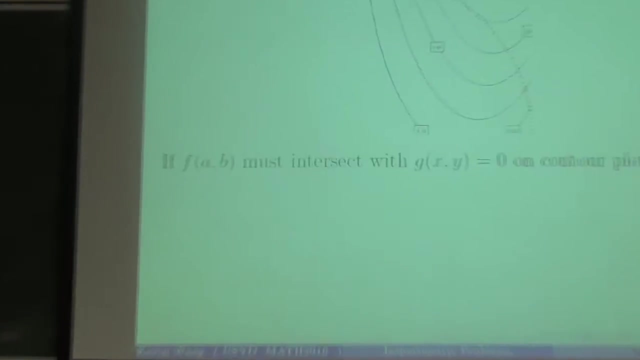 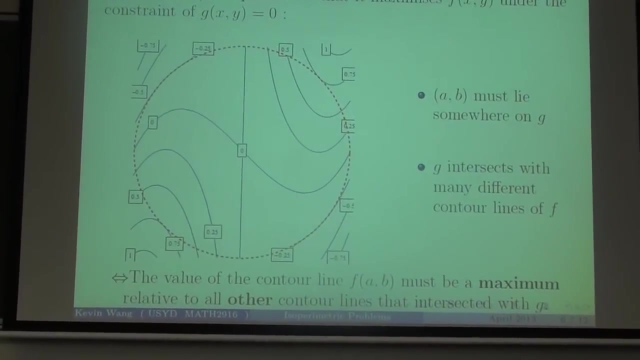 but that was intersect with g, but that would be a little bit higher than that. so we probably suspect something funny is going on here and this will probably be our maximum um. actually, is there any question about how i come to that equivalent in terms of control plot? any questions about this part? 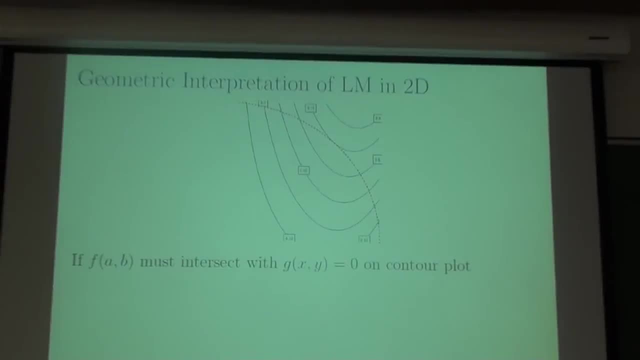 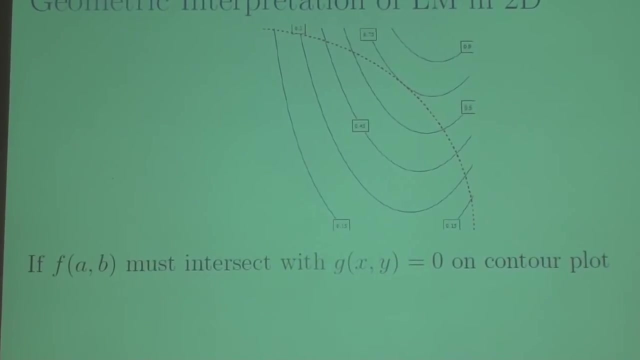 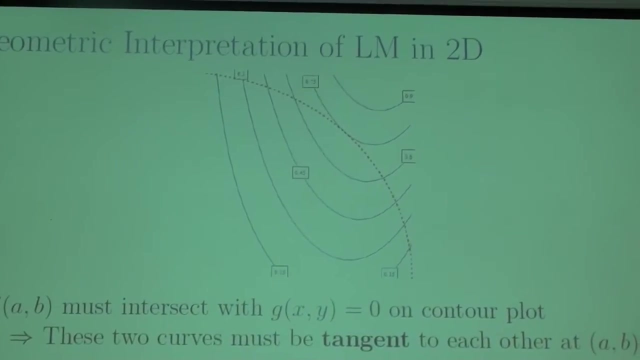 okay, so now this is assuming picture of that region I was talking about referring to, and here you can probably have a guess that if there is actually a maximum point, then must intersect tangentially. now how about make that claim? in fact, that's the extraordinary claim. how? 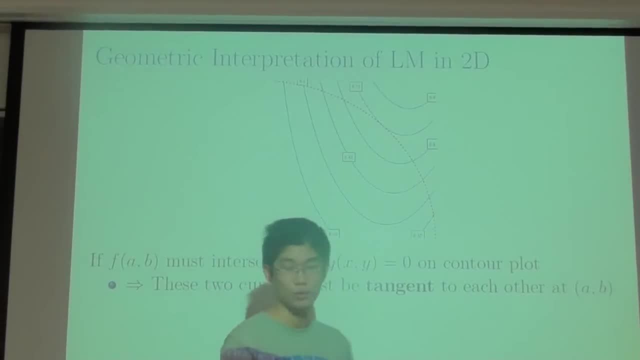 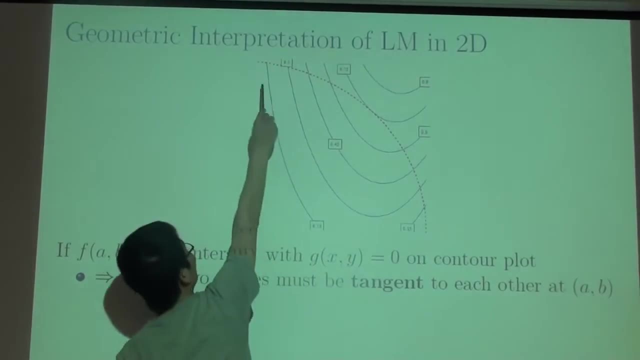 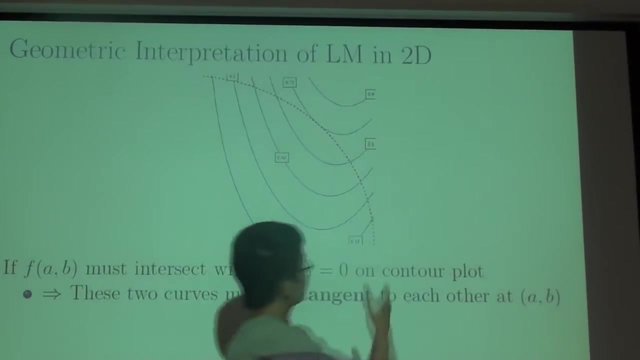 have to make this claim. well, to justify this claim, you have to use geometric intuition. now, suppose that you are walking along this. you're walking along this street, you're walking along that. now, as you walk along, you know that the g intersected with u as you're changing its value. but what happens when you 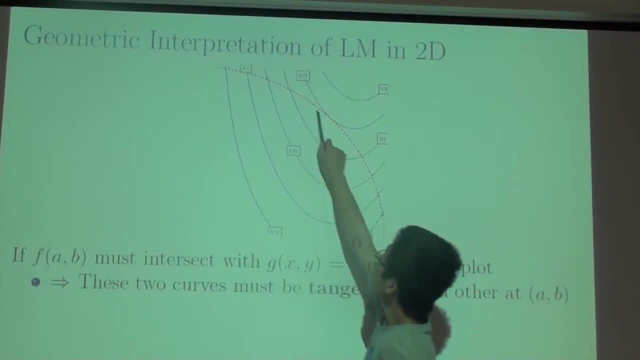 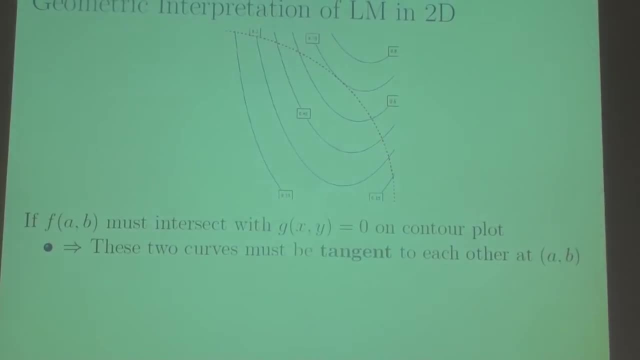 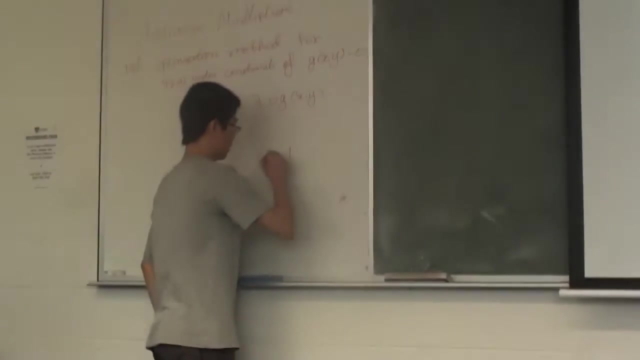 intersect tangentially. well, if they intersect tangentially, the value of f does not change locally and that corresponds to uh in ordinary calculus. if i can find my chalk, it's not here. you know that in ordinary calculus you have x and f of x and locally if you have a maximum around here. 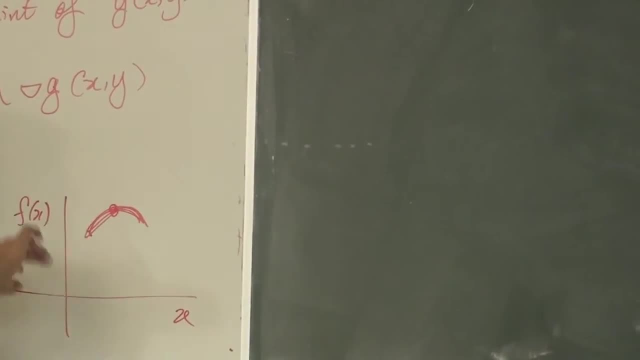 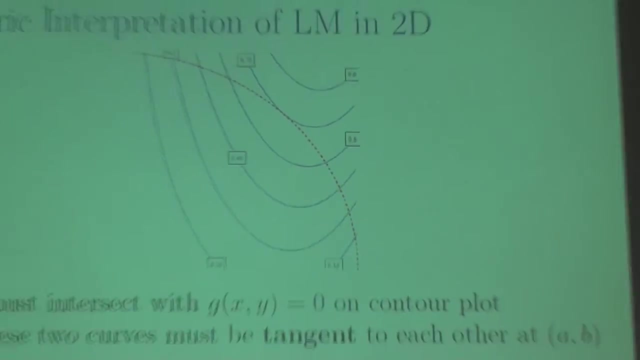 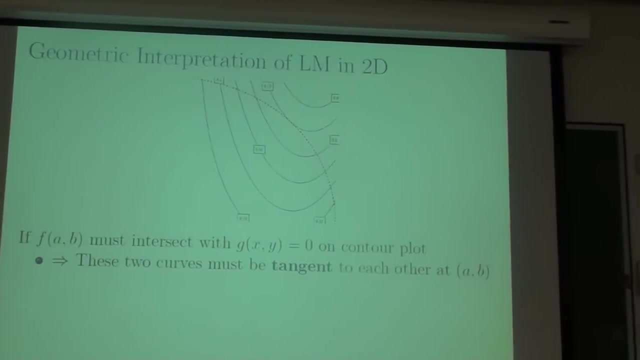 as you vary along x locally, the value for f does not change, and this is basically the same idea. the only difference is that you're walking along g rather than from x-axis. so that's a claim that if there is an optimization point, the two curves must intersect tangentially. 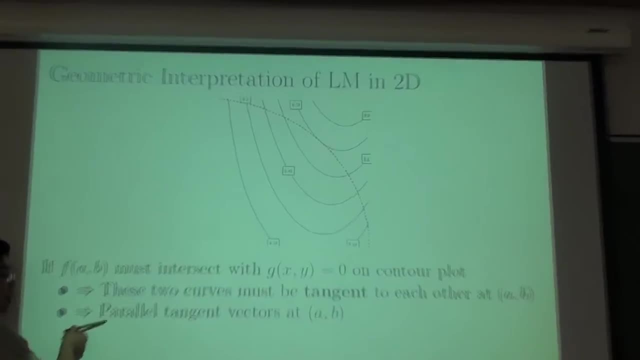 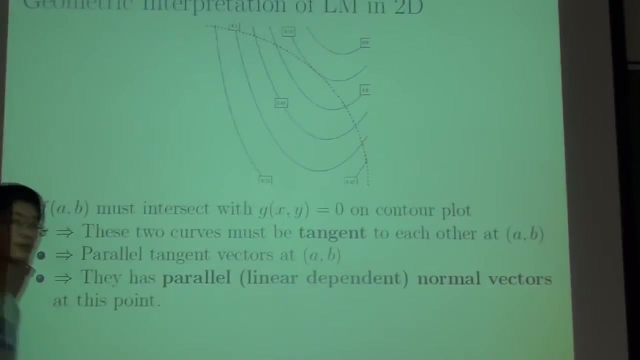 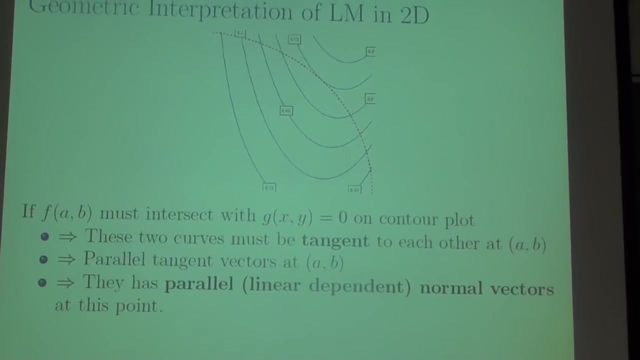 and that's equivalent, definitely equivalent to say they have parallel tangent vector and that's of course equivalent to saying they have parallel normal vectors. you can think about parallel tangentially, then no one must be parallel and of course, in other words, for parallels they were linear dependent. 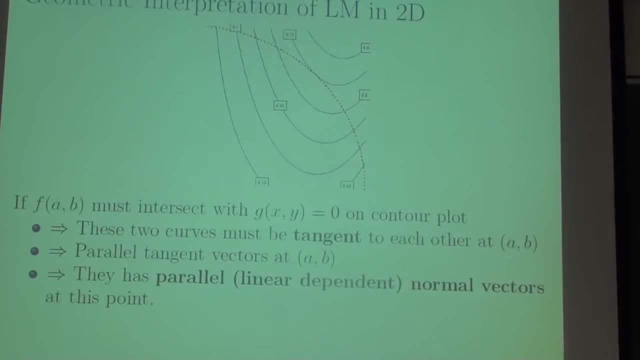 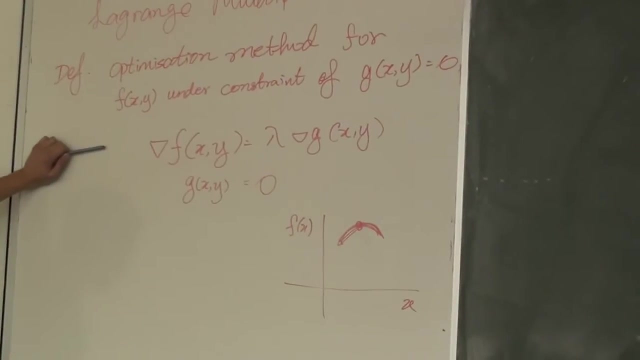 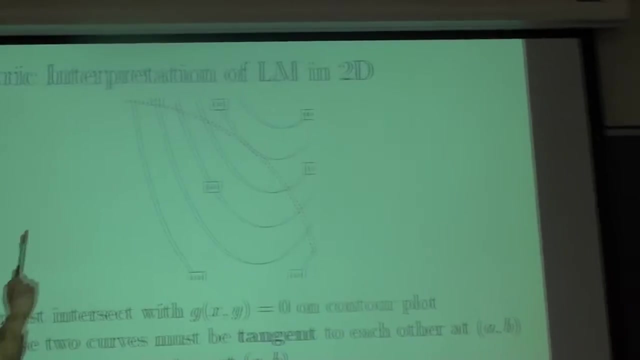 so just about this line. here we justified our first criteria. oh sorry, you're supposed to be sick anyway, we just have this criteria. that which is why i've written here, because no vector for the counter plot of f is right f and it's linear dependent. that's why i have the vector there. 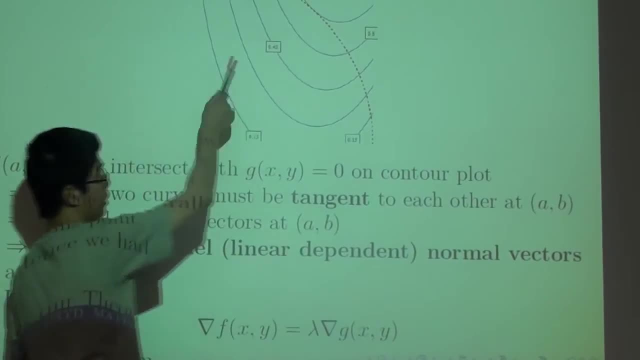 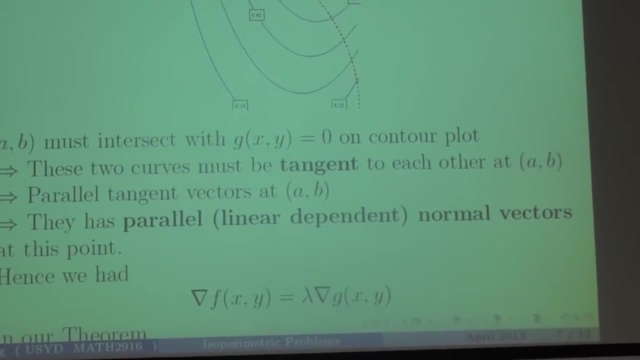 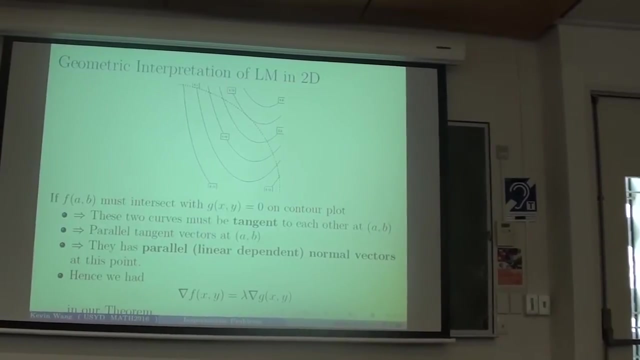 it's the constant there, and right gb is definitely the normal vector for the counter for the contour plot of G at every point. So are we in question, or do you want to clarify this in an alternate point? Are we all good? OK, great. 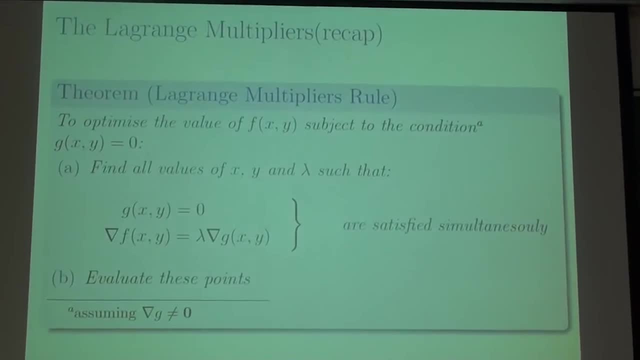 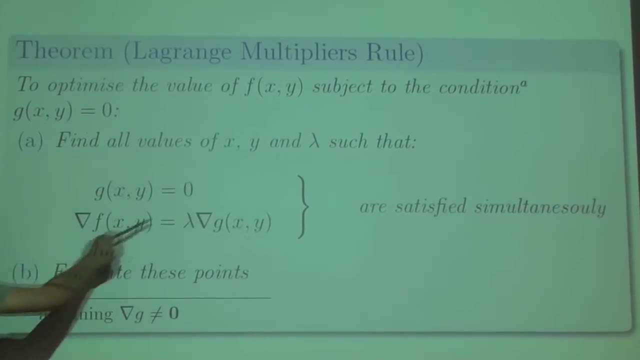 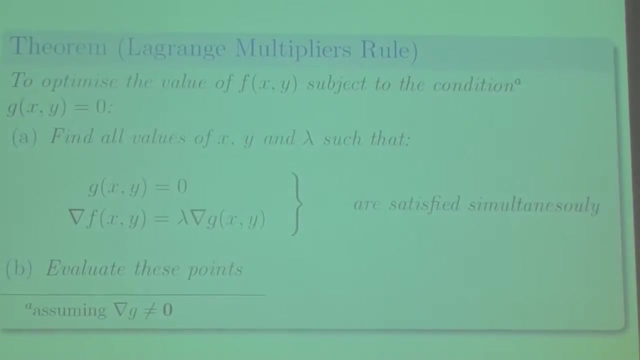 So here's actually the large multipliers equation itself, And it's nothing more than I just showed you. You have to solve this regression simultaneously, And once you get a bunch of points there, you will evaluate these points. So how do we know this thing will work? 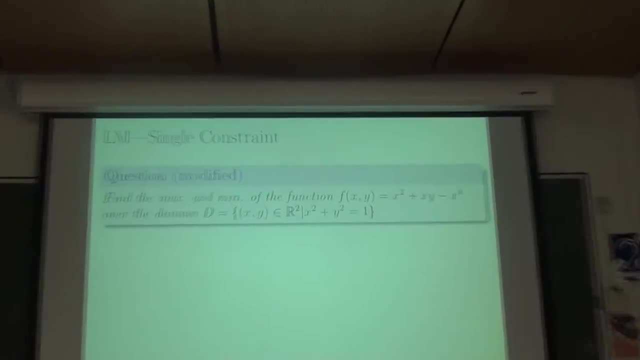 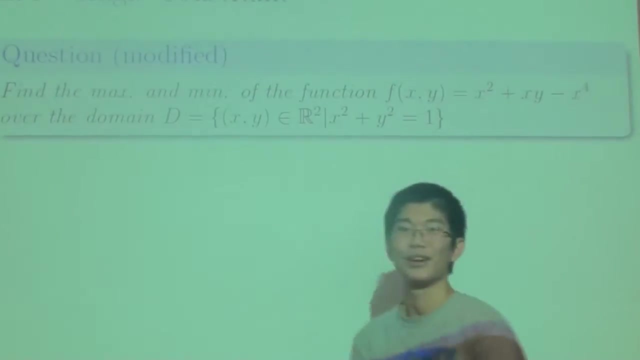 Well, it's simple. We'll do an example. So this is actually question three in the effective calculus assignment, And this is the function you have. And now I'm going to try to equate. All right, Have you handed this already? 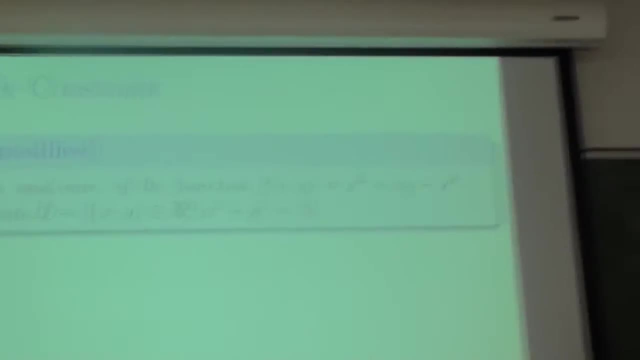 Yes, We already gave it back. We'll return it- I mean, everybody's got it right- Because I don't want to cause any trouble, Otherwise I just leave out a solution. I just call a solution if you don't have it with you. 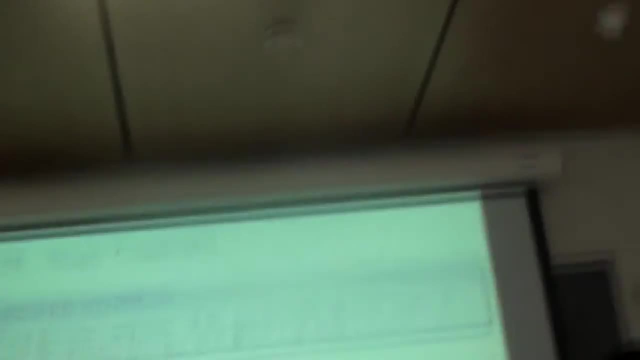 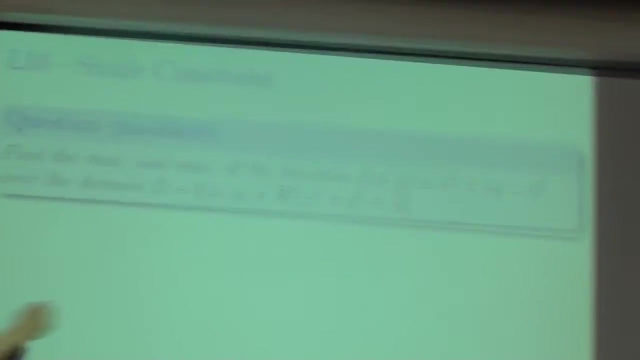 But a domain. actually, we don't care about what's the interior, Because if you don't have a question, you don't have an interior. it's simple. Or if you really care about the boundary, project it upwards. So that's why we have an equality sign. 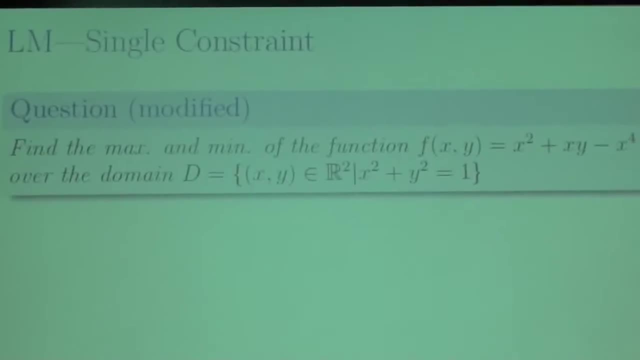 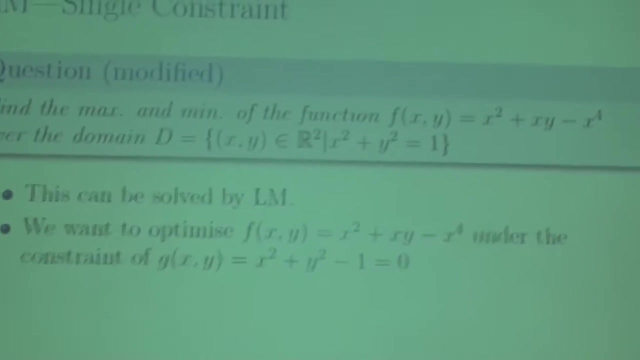 rather than the inequality sign, Because we only care about boundary points And, of course, so far, the large multipliers. And it's definitely saying that we want to optimize f under the constraint of g. So this is trying to switch the visualizer. 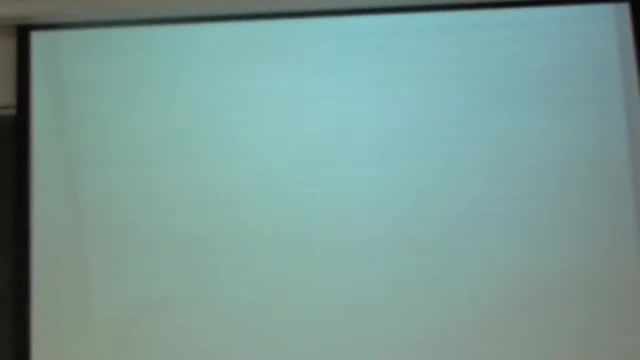 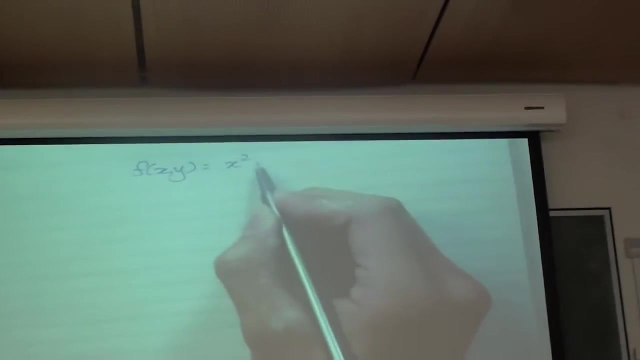 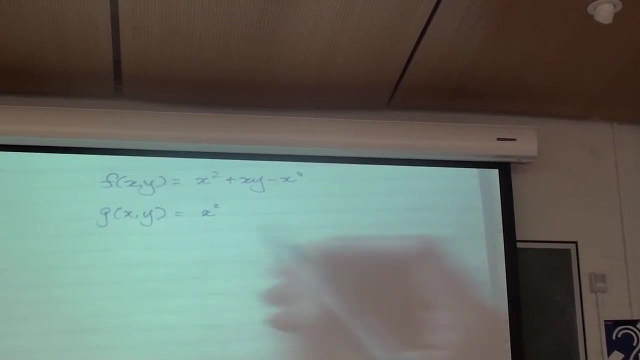 And let's see. Can you write the equation out first? f of xy equals to x squared plus xy minus x1.. g of xy equals to x squared plus y, squared minus 1 equals 0.. OK, that's our question. I want to optimize it. 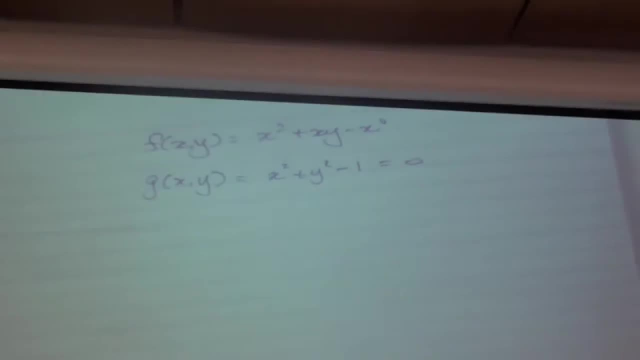 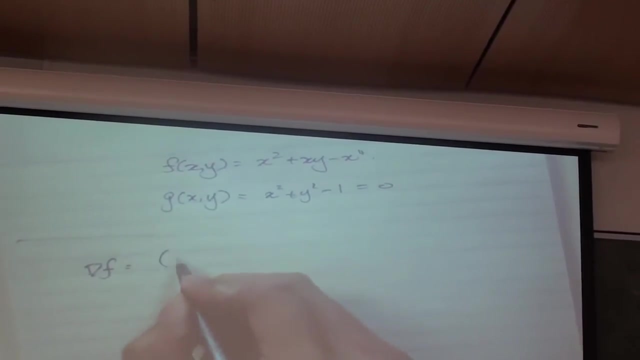 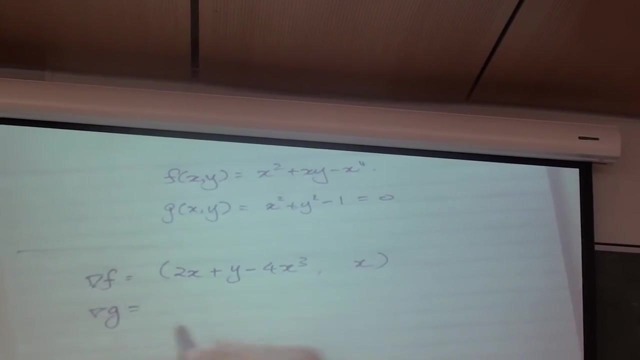 So firstly we'll form this, We'll actually count the gradient of each function. So the gradient of the graph f- Actually it goes to 2x plus y minus 4x cubed and x Rather f over g, is simply 2x 2y. 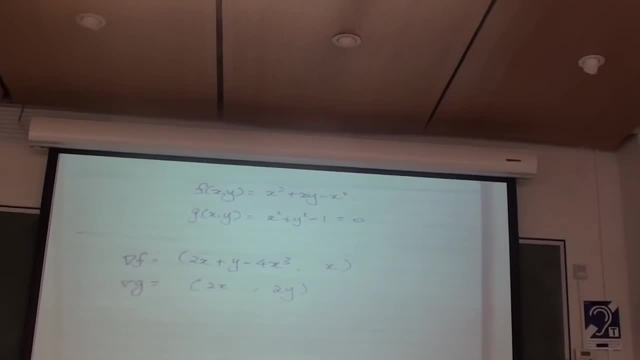 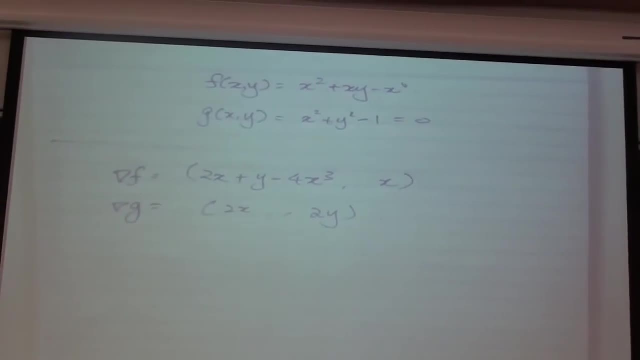 Ah, this is too difficult, Sorry about that. So what we're going to do now is equate the partial f, partial x, with the partial g, partial with the partial of g. So that's 2x plus y minus 4x. 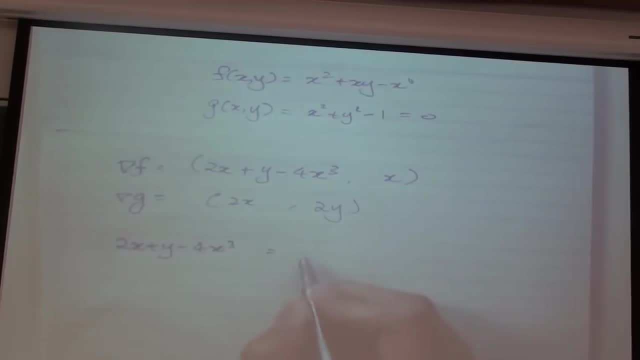 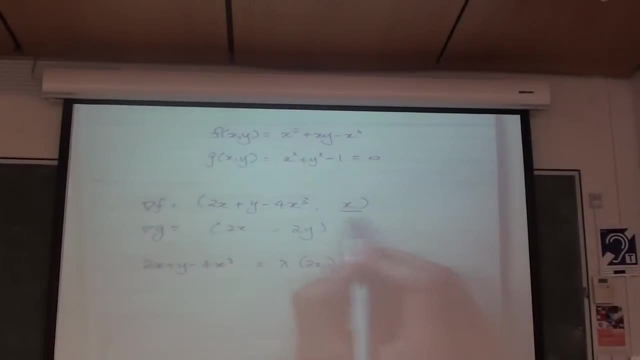 Sorry about that, OK, OK, OK, OK. So that's 2x plus 4x cubed equals to some constant lambda. OK, that's what we have there, times 2x, And at the same time we'll have x, and equate that with this. 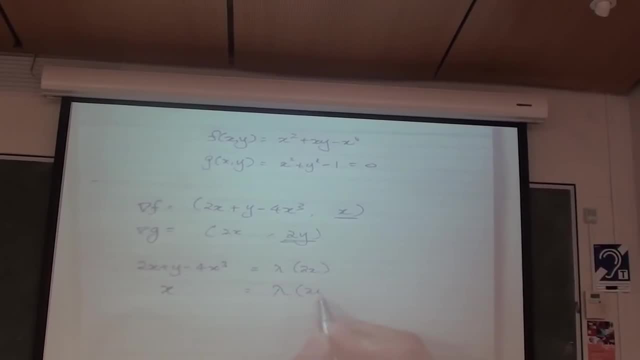 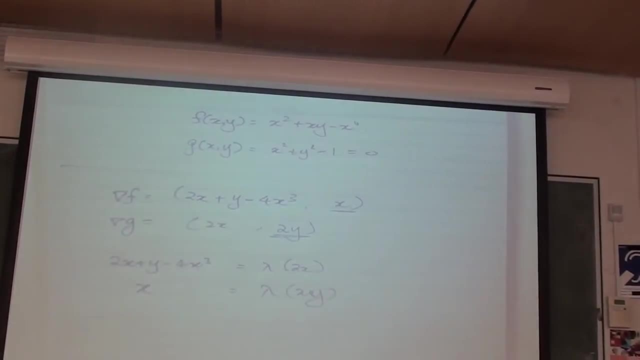 So that's: x equals 2, lambda, 2y. And our third equation: notice that we have x, y and lambda, So we need three equations. Our third equation comes from the fact that we have the original constraint, So let's put the constraint out. 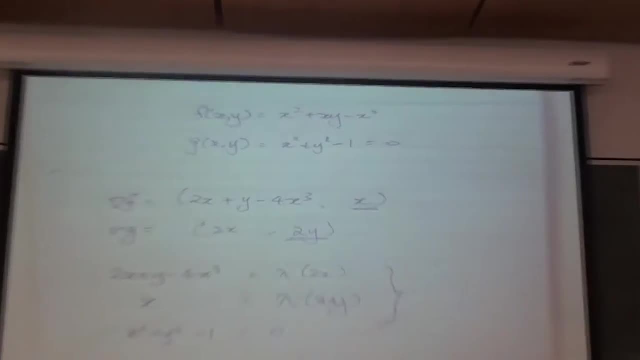 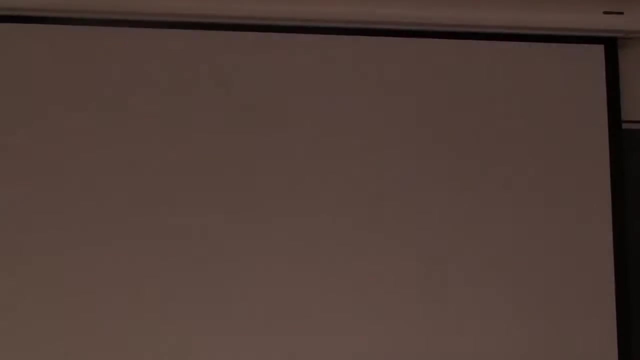 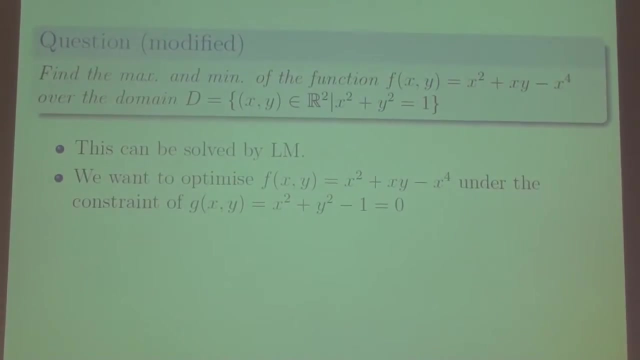 So what we have to do now is to solve this equation simultaneously. Now, to do that it's not always possible because, as you know, as the power goes on, the solution becomes more and more difficult. There is a factorization for this. 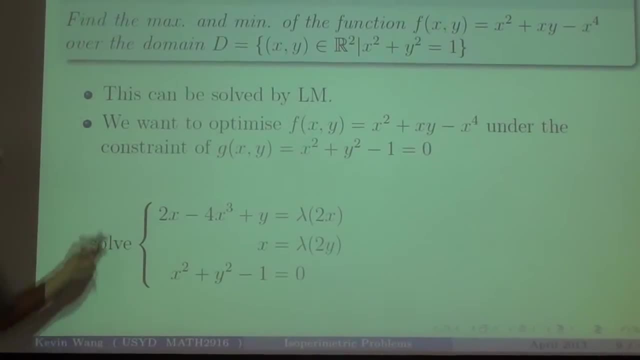 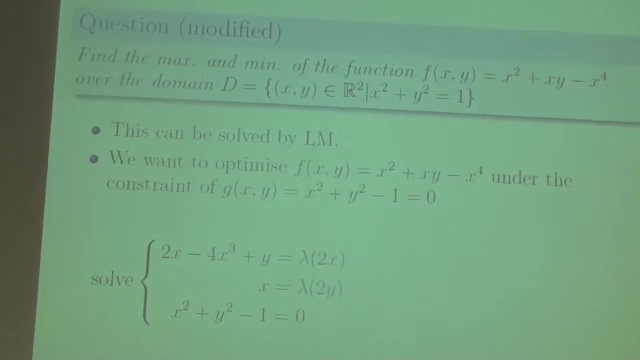 These three equations. there's a factorization which takes a bit of time, but I will skip that. What you can do now is do what I always do: put that into Mathematica, And I'm sorry. I just really hope you go ahead and finish your assignment. 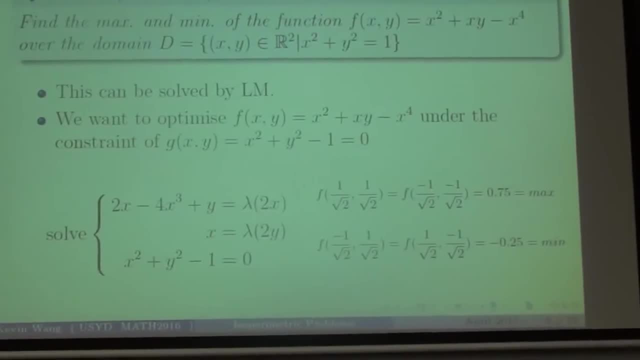 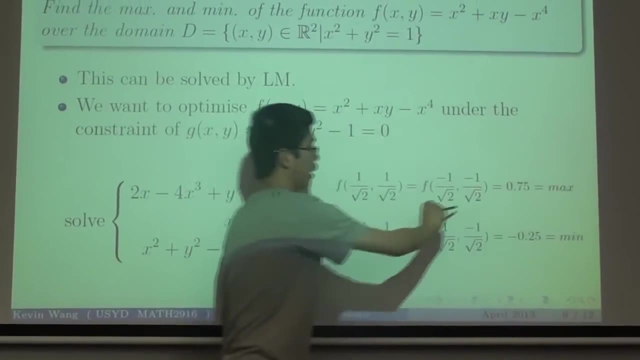 because here's the answer. And of course you get a bunch of points, That's 1 over 2, and those are 10 designs And evaluate them at points, The first line gives you 0.75, the other one is minus 2.5.. 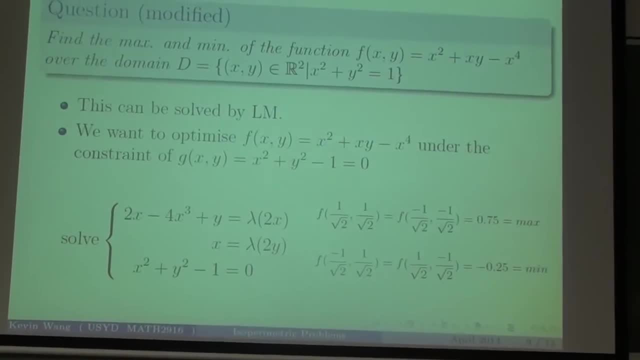 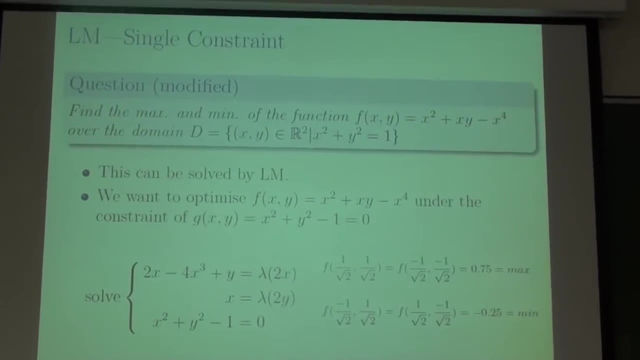 But minus 0.25, the top line's maximum, the bottom line's minimum, and that should be pretty clear. And that's exactly what you get in your parameterized equations When you do that assignment a few weeks ago. So that's the one-multiply method. 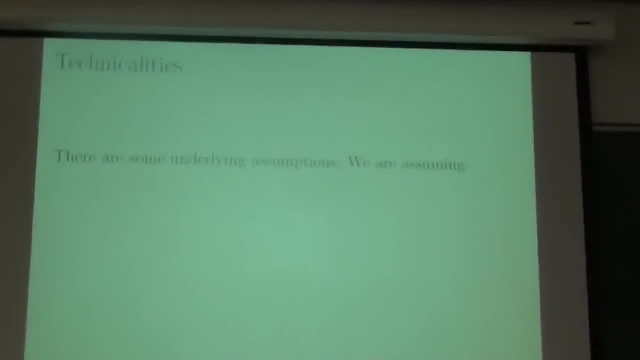 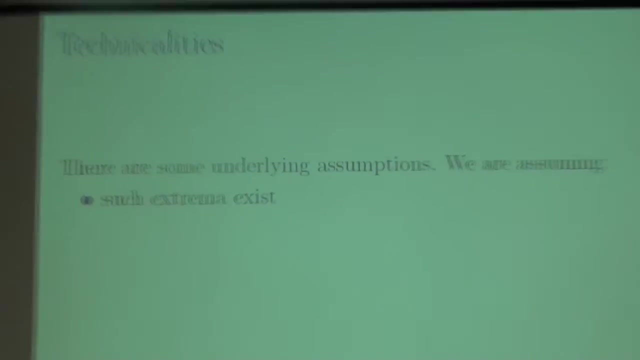 It's fantastic, But there's something we have to think about this. right, There's some technicalities. Well, first thing, we'll assume there is actually extreme odds, Extreme odds, OK. Now secondly, we have to make sure. 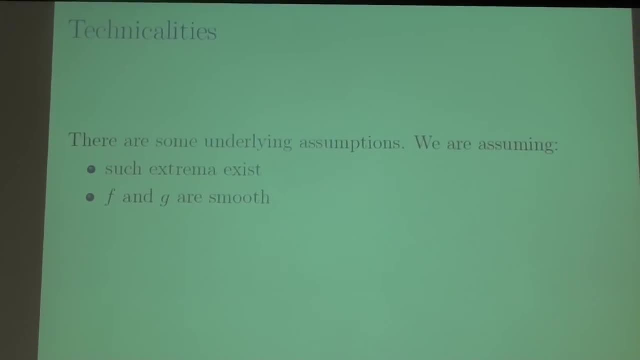 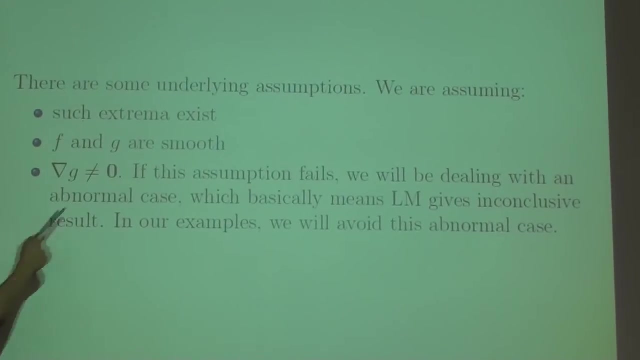 they're both smooth functions. Now what's that mean? Well, if this condition does not hold, what happens is that we cannot make it. We cannot make that geometric argument we made about the intersang tangentially, In particular, if the gradient of G is equal to 0, OK, if that. 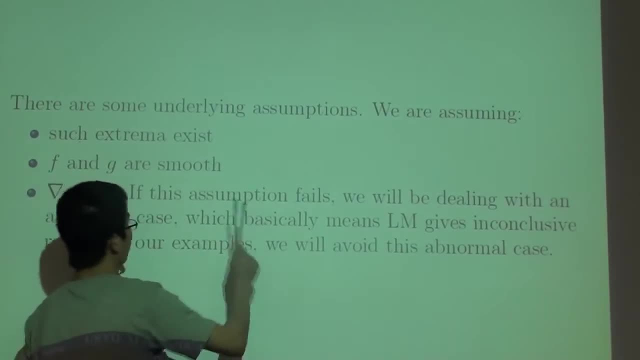 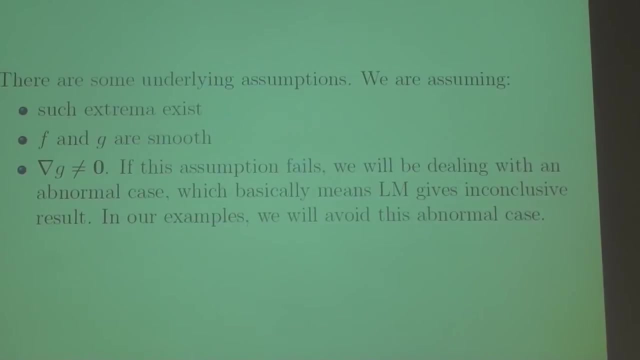 is something else, or it is equal to 0, then we'll be dealing with something called abnormal case, Or, if you think about it, it's a little bit degenerate case, And in that case you don't know what happens. 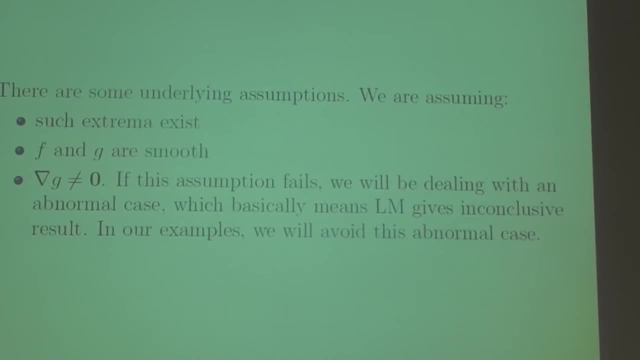 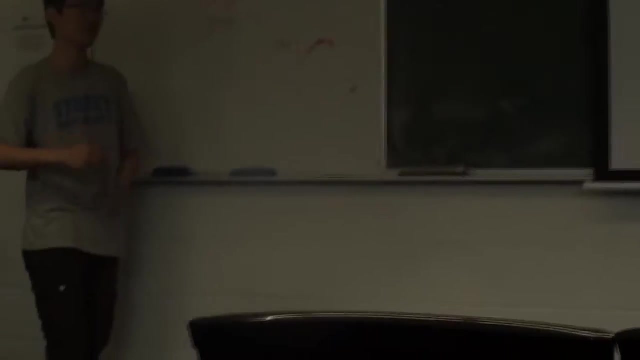 The large multiplier gives you an answer, but that answer probably doesn't necessarily satisfy the gradient, The F or the G or things like that. It could be a maximum, it could be a minimum or it could be neither. So you cannot draw a real conclusion from that. 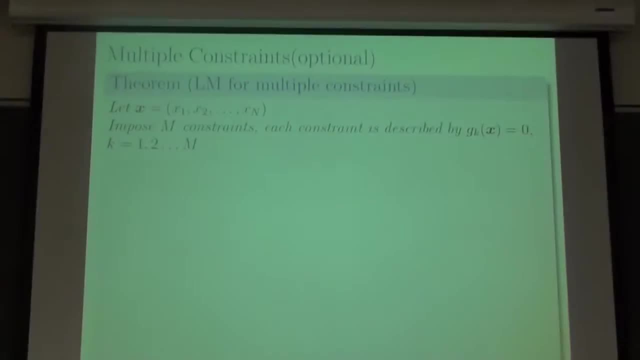 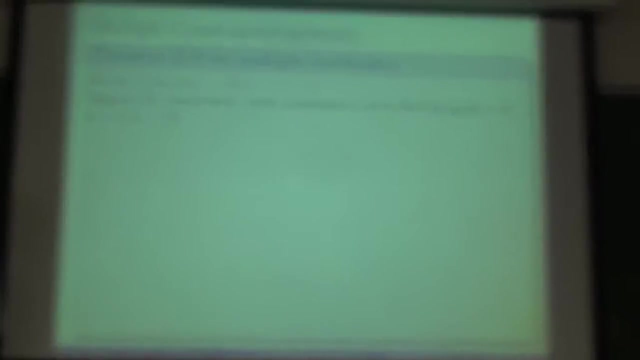 And of course this is a little bit optional, but I should quickly mention this- is that the large multipliers can be used for multiple constraint problems, And this is where the large multipliers really shines. For the large multipliers of multiple constraints, they 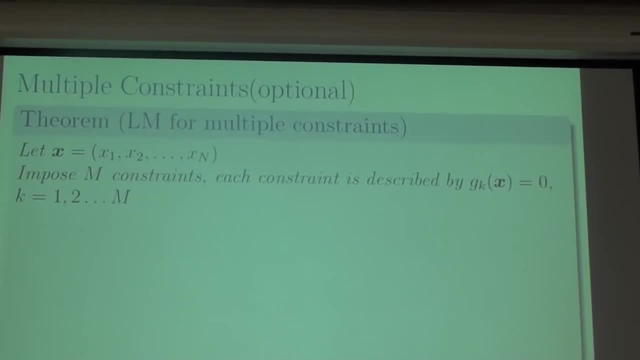 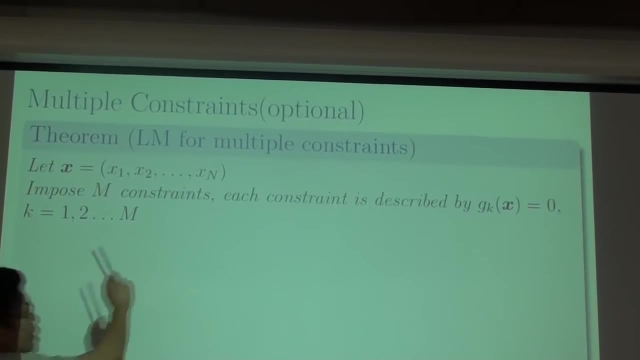 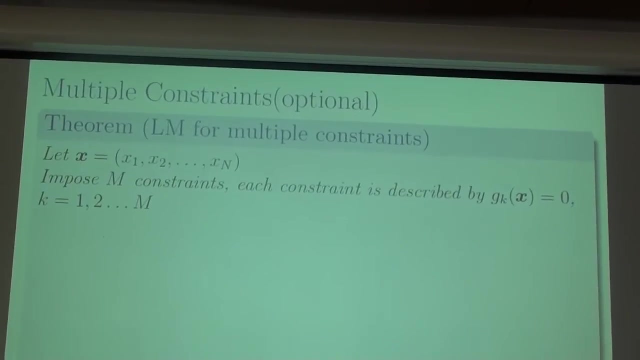 obviously have to consider higher dimensions, And now we have m constraints, whereas before in the assignment we had one, Now we have m constraints And each of those constraints is a function, And that is exactly the formulation. like that, only in higher dimension. 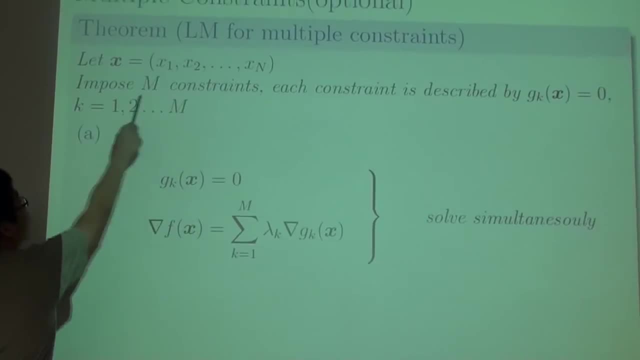 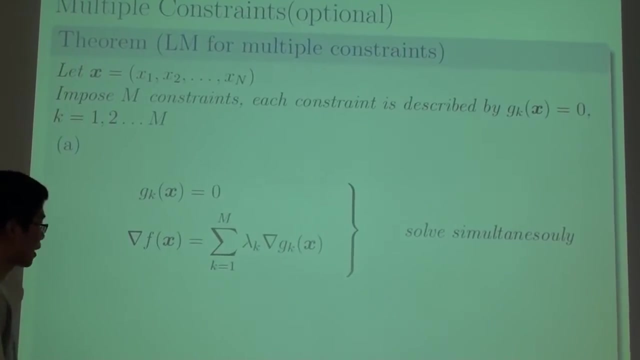 Then we'll still have two criteria. The first criteria is the constraint itself. It should be natural enough, because it's always going to satisfy constraints. Our second criteria comes from the constraint itself. It should be natural enough because it's always going to. 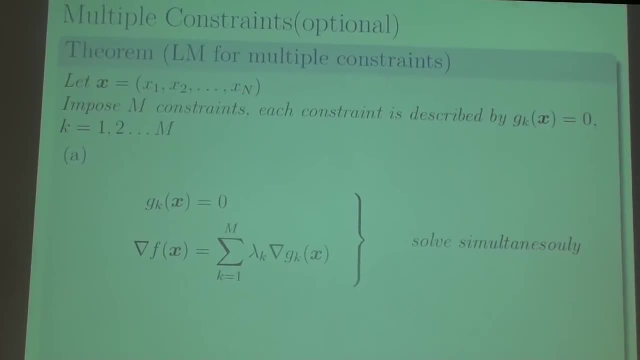 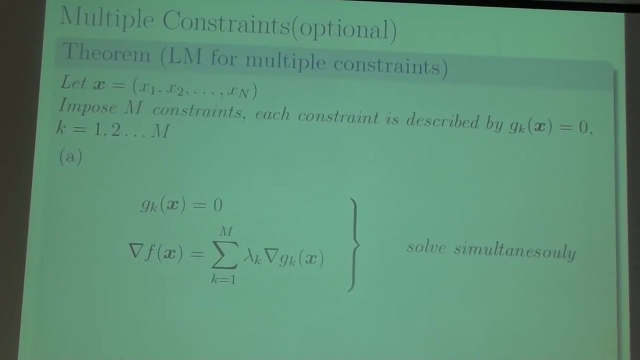 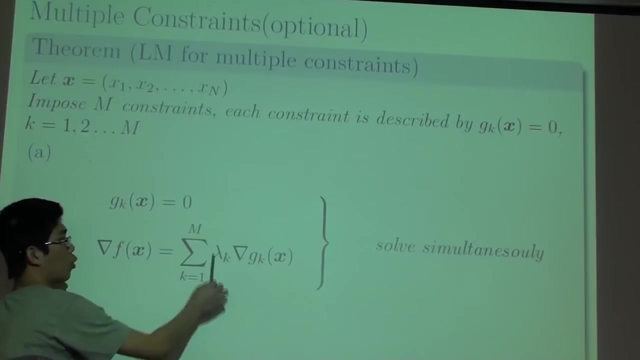 satisfy constraints. And that comes from the fact that, well, that's the generalized result from our single constraint problem Because, remember, when we talk about single constraint we mean the second tangentially. We make that claim of linear dependency. Now, this is a linear dependency, provided that all the letter k 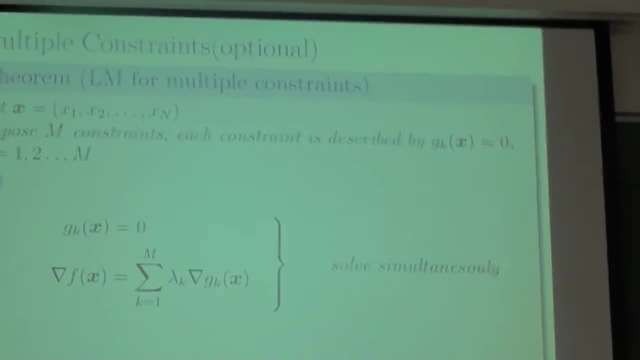 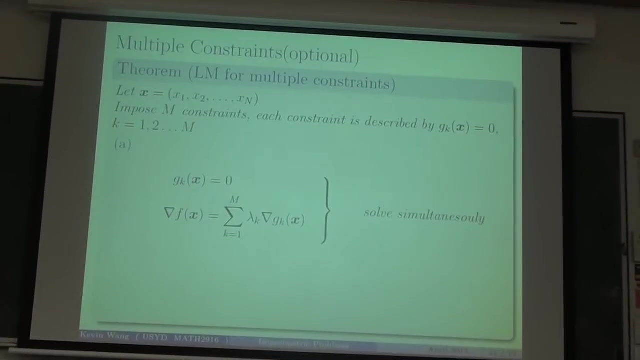 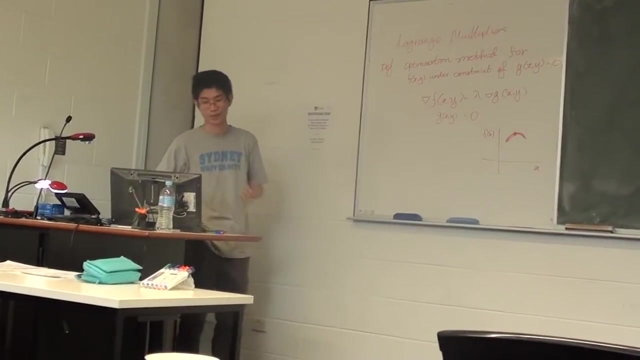 are non-zero. So here's a generalization of the lower dimensional case. The precise formulation of this is very simple: It's a linear dependency. It's probably beyond what I could do today, because there's always a constraint for that Constraint, constraint. 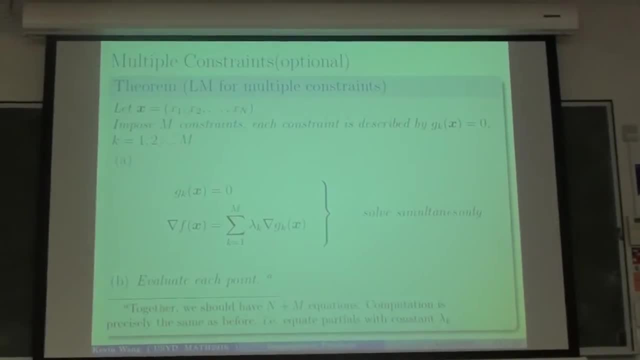 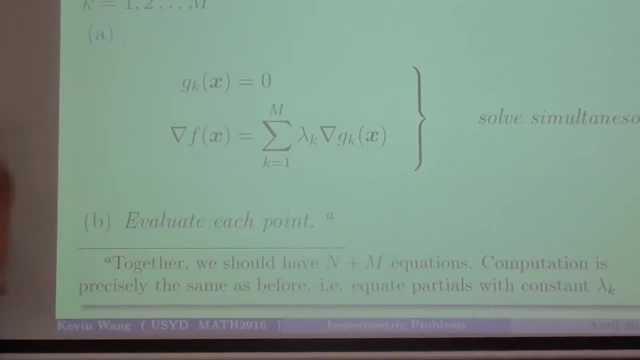 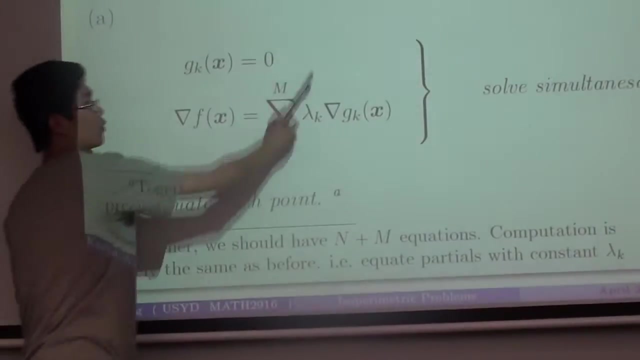 Oh, That's funny. OK, And of course you calculate the value at each point. You calculate all the points from here And together you should realize that we have m plus m equations out of all of this. Now that quickly becomes very difficult to solve because it could be nonlinear. 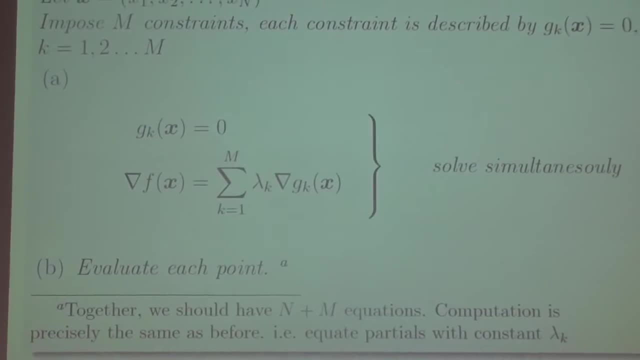 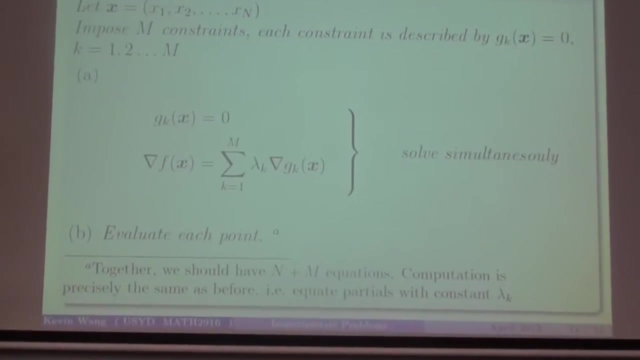 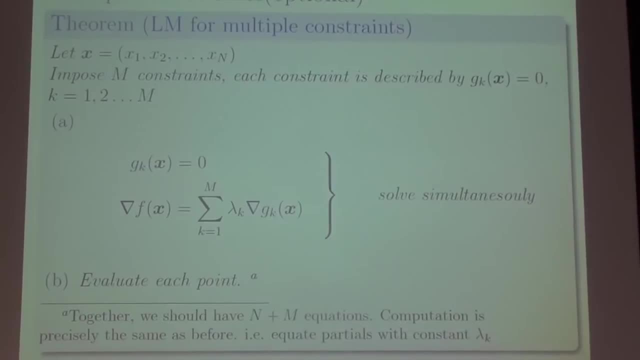 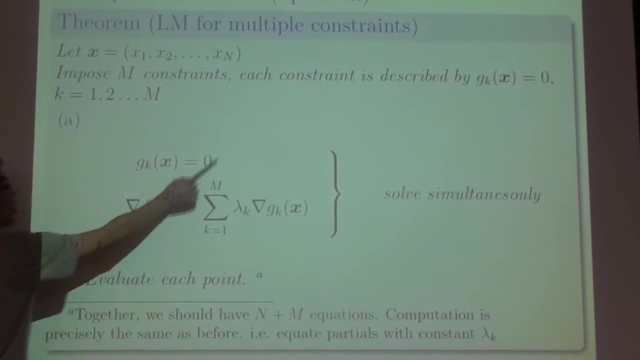 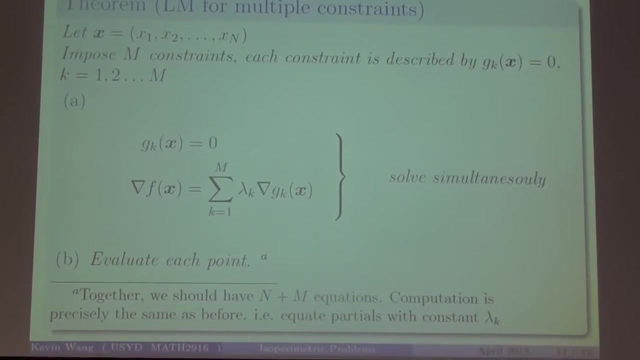 the fact that computational solution is absolutely fine. But the formulation of those equations are precisely the same, right on the constraint and right on as a linear dependent of vectors, And you solve them simultaneously. So here we actually conclude our first section on Lagrange multipliers. 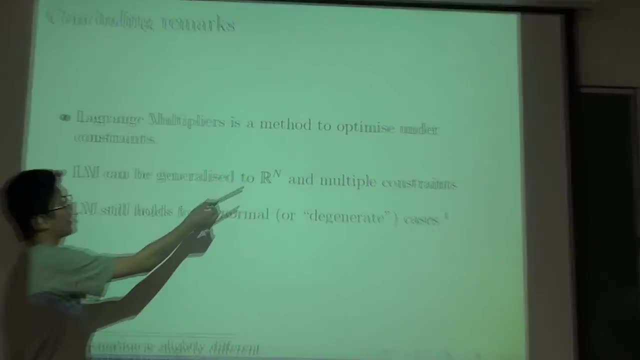 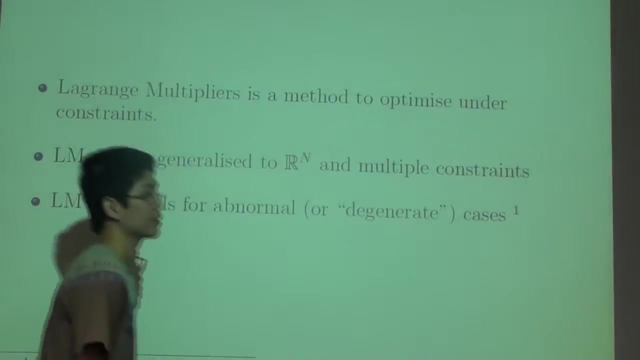 So let's summarize that Well, we know that Lagrange multipliers are a method of optimization, nonlinear constraints And Lagrange multipliers can be generalized into very high dimensions and multiple constraints, And this is where Lagrange multipliers really becomes the most powerful technique I know. 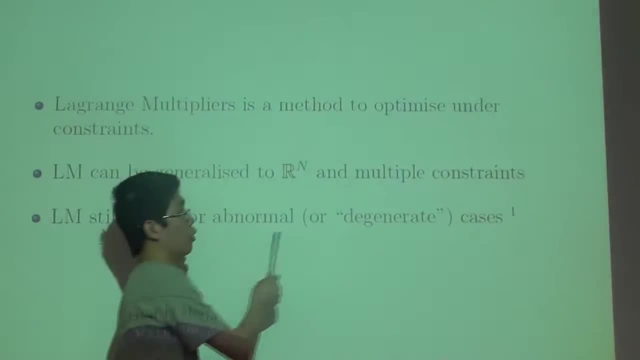 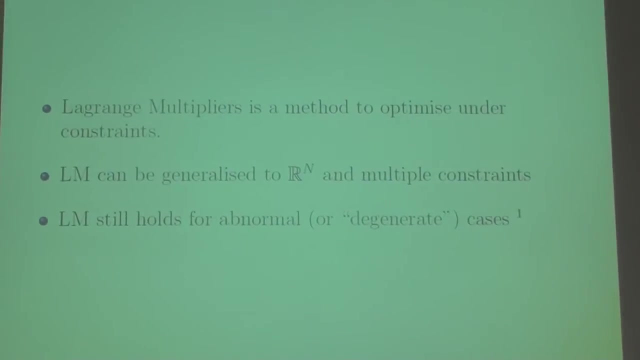 so far, And Lagrange multipliers of course actually still holds for the degenerate cases. But it's in the slotted formulation, formulation which, if you're interested, you can read about it. But essentially what that is: you just put a non-constant in front of graph G so that you avoid that zero case. 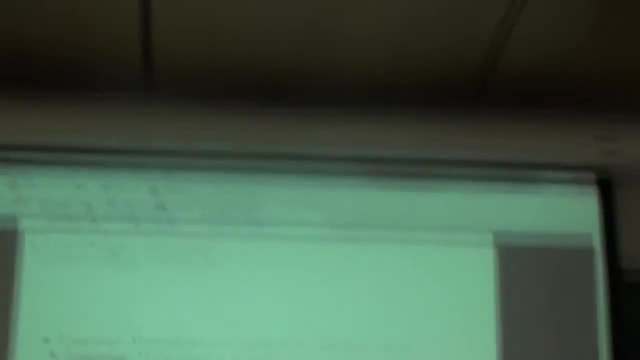 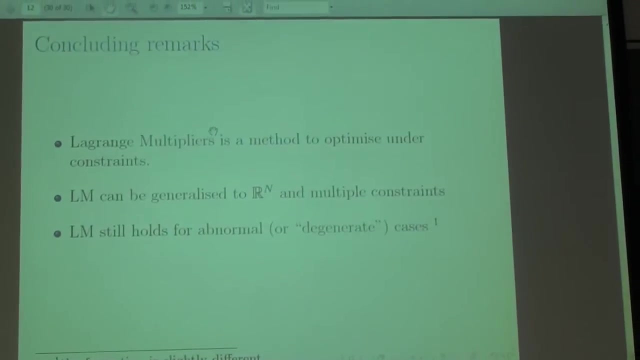 So this ends my first section. So any questions you want me to ask. Yeah, just a question about one of the assumptions. You said that we're assuming that solutions exist. If you can't solve Lagrange multiplier equations, is that sufficient to tell you that there aren't solutions? 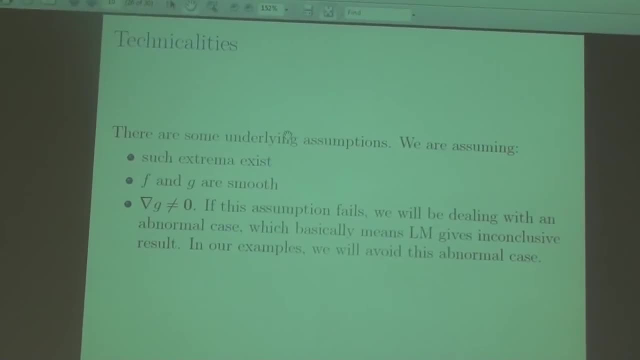 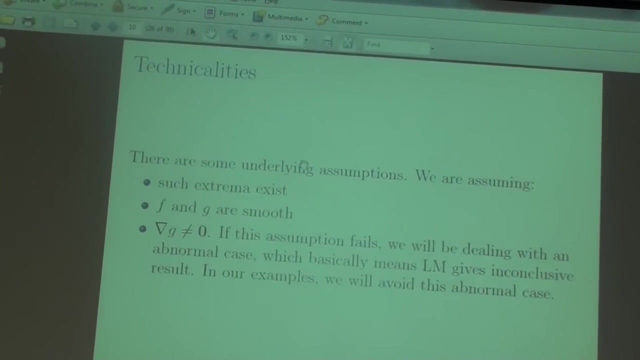 Yeah, that could be the case, Because if you cannot solve them, perhaps there's something wrong with the equation, Because maybe your solution, your two graphs, f and g, probably don't exist in the same domain and you could have a problem there. 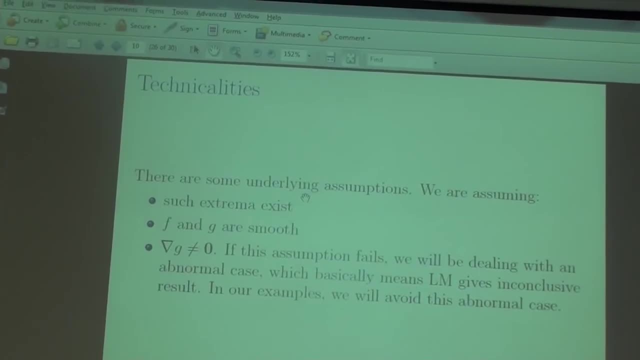 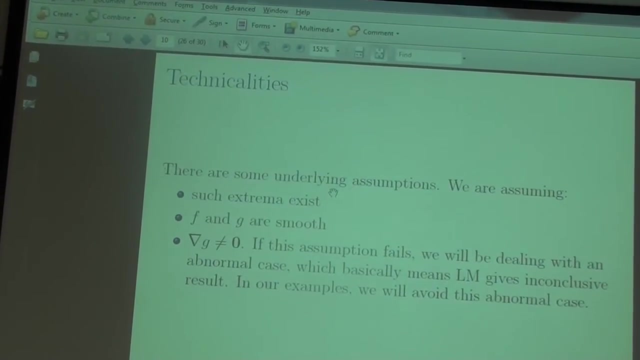 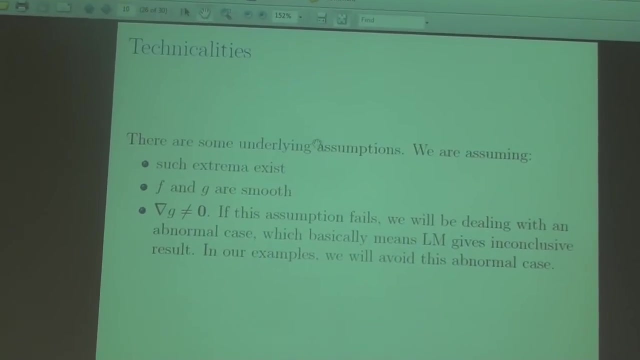 And I'm not just saying a problem. I should give you a solution. but that solution is not even the maximum or minimum, because the whole curve is continuous and diverse from infinity and the minus infinity And there's no maximum or minimum. Let me figure out how to do this. 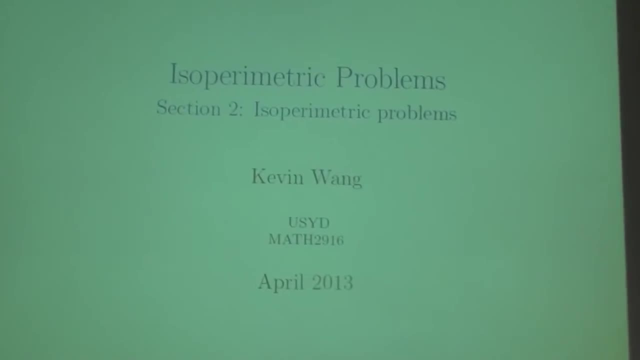 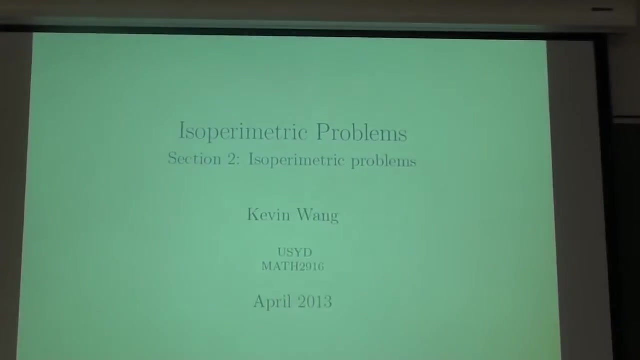 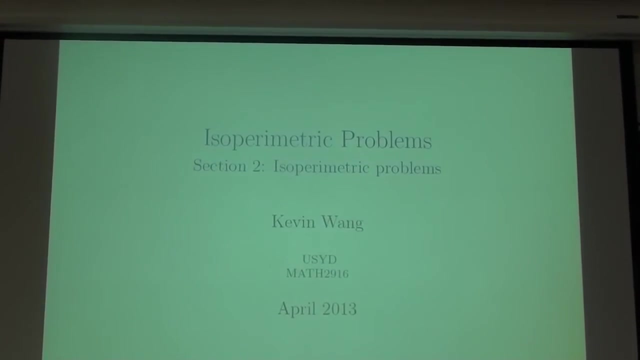 So now we'll come to the isoparametric problems themselves. As I mentioned before, we're representing a theorem here which uses the Watt-Mobil factors, So what I want to do now is to keep this equation over here, because we'll refer back to it, But in fact we're going to write it smaller. 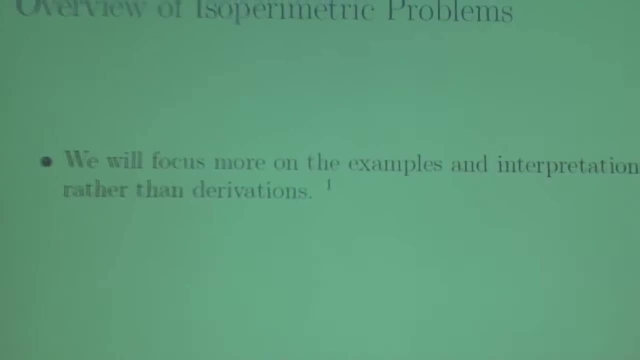 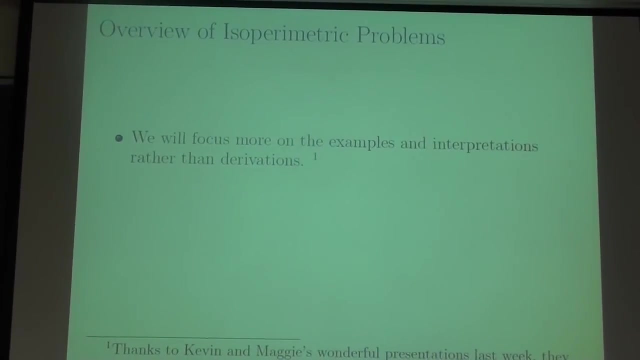 So here we've given an overview of what isoparametric problems And, in particular, we'll actually focus on more examples and applications rather than proofs and derivation, because thanks to Maggie and Kevin, my life is much easier. Thanks, guys. 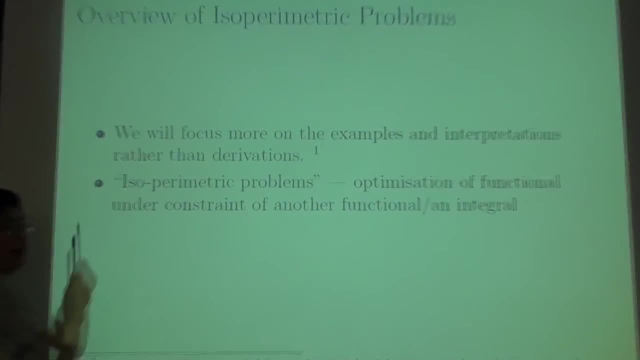 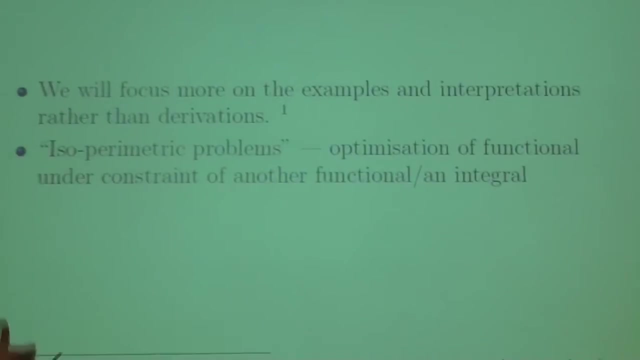 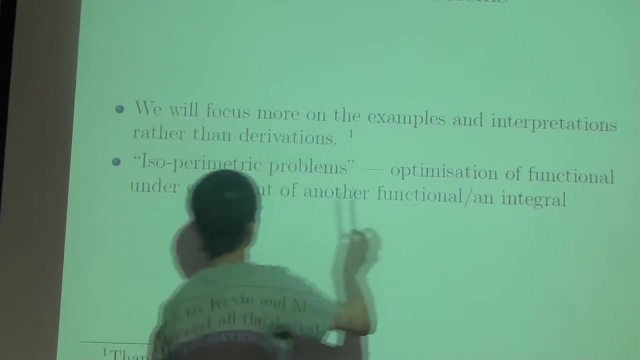 Okay, so isoparametric problems. The prefix iso comes from the word the same and parametric comes from the word perimeter or up-left. Therefore, in the whole topic you can think of this problem, this IP problem in optimization of functional under the constraints. 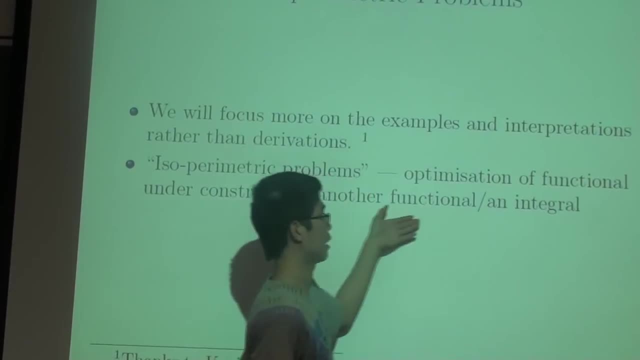 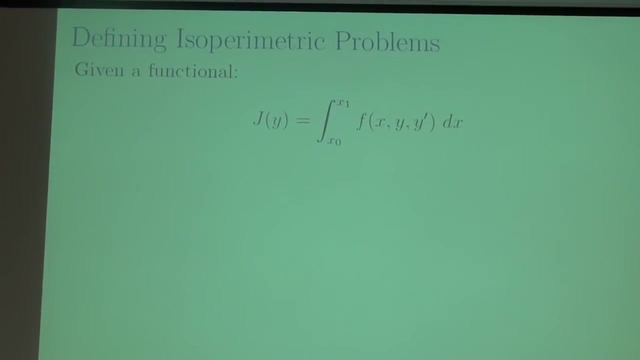 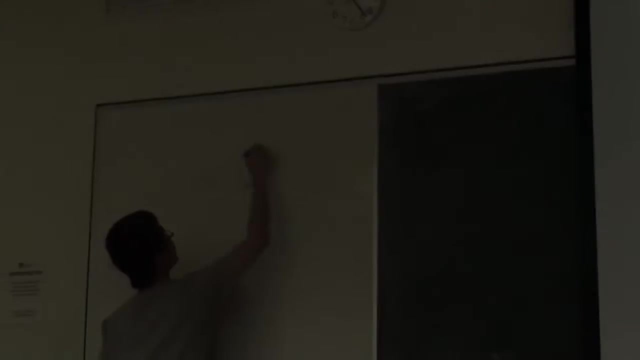 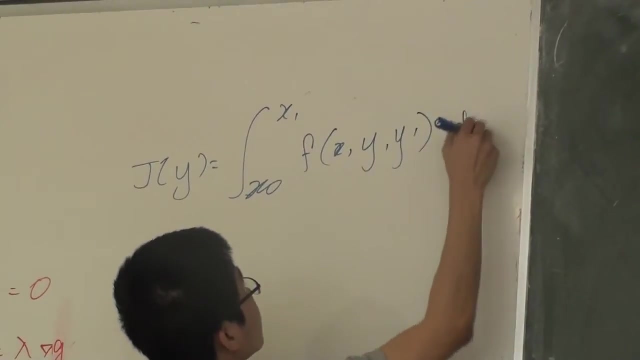 of another functional which, almost equivalently, you can say, is under the constraint of another interval. So let's define that more precisely. So probably this is good time to export. So, given a function of this form, j of y equals to the interval of x0, x1, integration of some function, f, yy-dx, We know how to optimize. 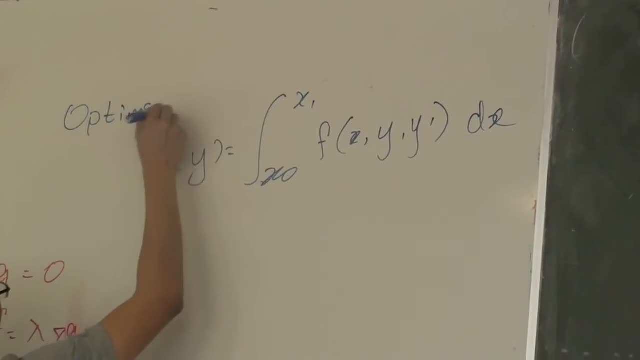 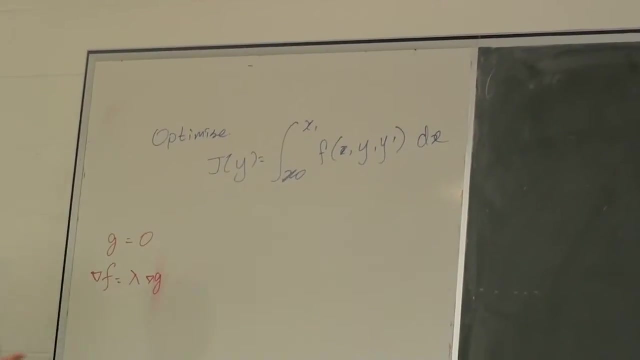 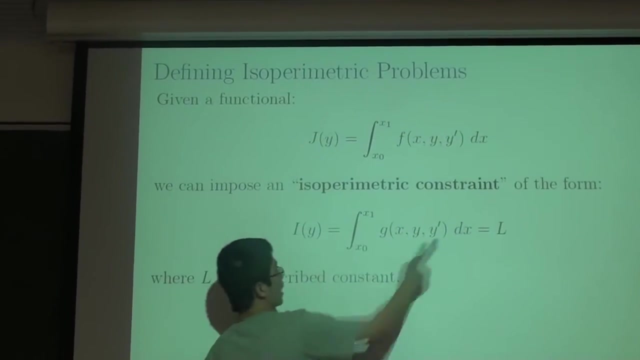 this Last week from Kevin. we just simply used the Euler-Lagrange equation on this thing and find the extreme over that. Now, once we have this, we can put what we call an isoparametric constraint, And this constraint is in the form of a functional or integral, and that integral must deliver to L. 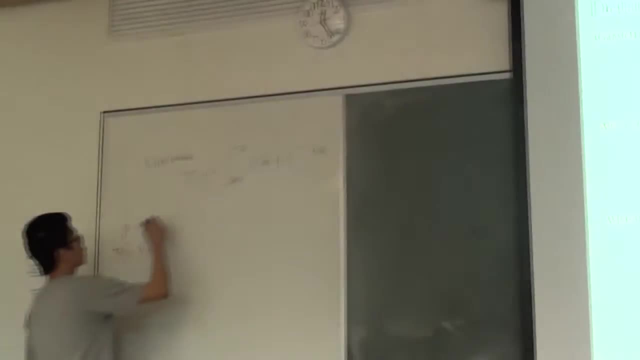 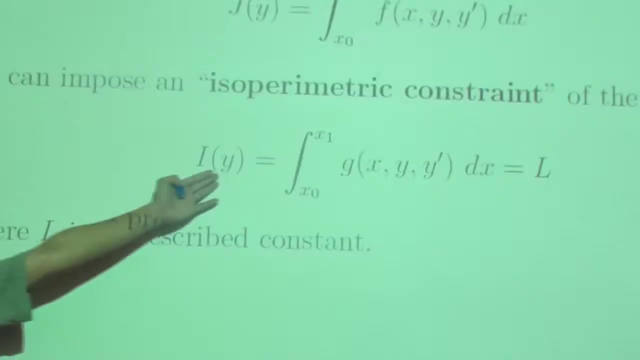 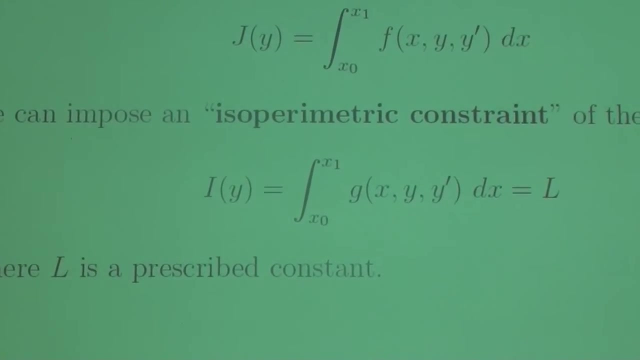 so, to put that into context, you can think of the constraint as being non-negotiable. Okay, Because whatever function I have, whatever we have, why you must give L at the end of the day? If it doesn't, you just throw that function. I don't even need that function. So this constraint, 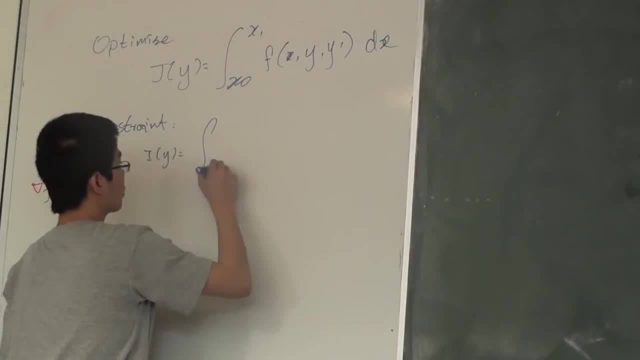 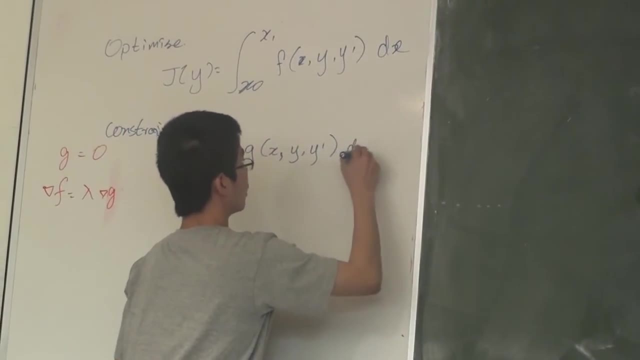 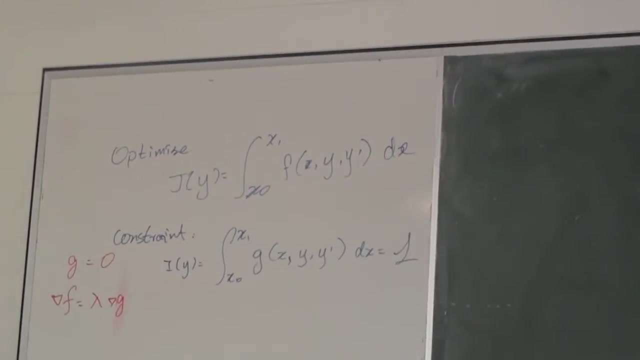 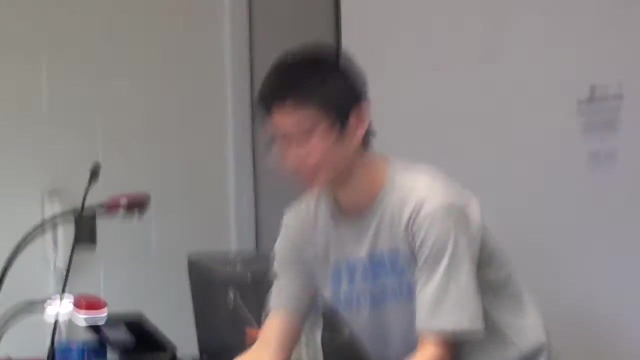 say, is that I of Y between X naught X1 and G of X, Y, Y dash dx, And that always is valid to some constant L, Always. So our problem arises, naturally, is that: how do we actually find, how do we actually find, the extreme of J under this constraint? 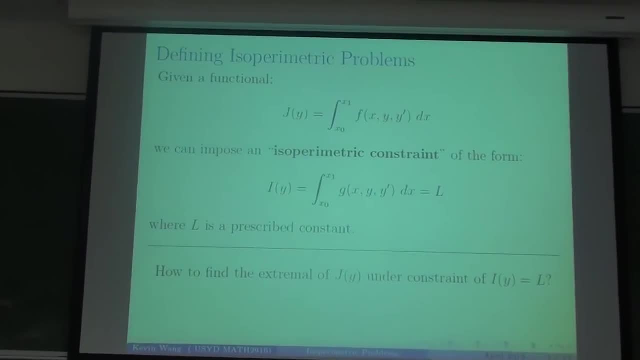 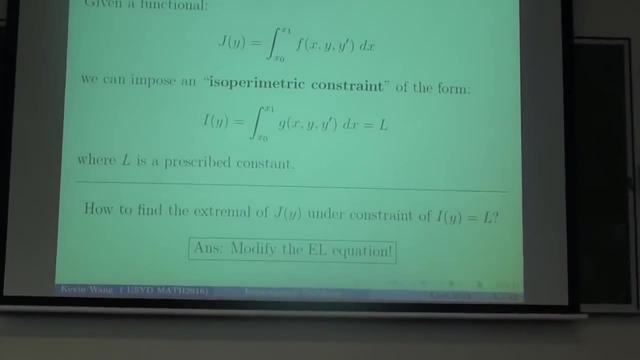 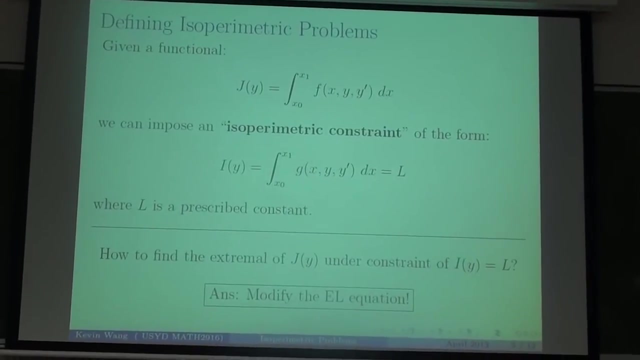 Can you guess this? You actually just modified one of the Lagrangian equations, And there's nothing wrong with doing that. I should do the proof of this now. Now, even though I say proof, even though I actually say the word proof. 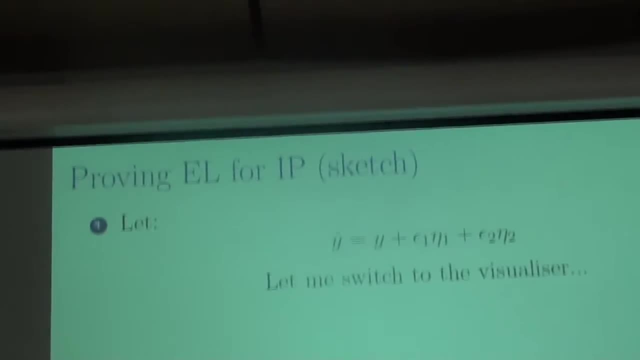 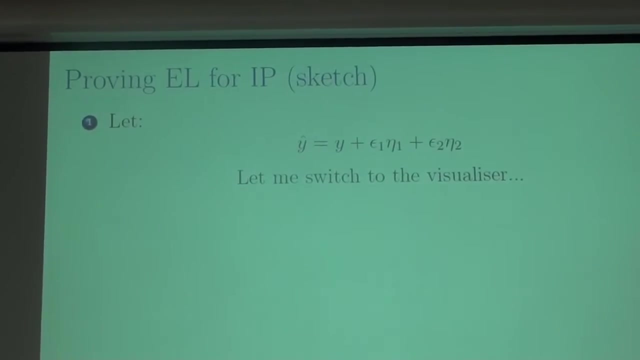 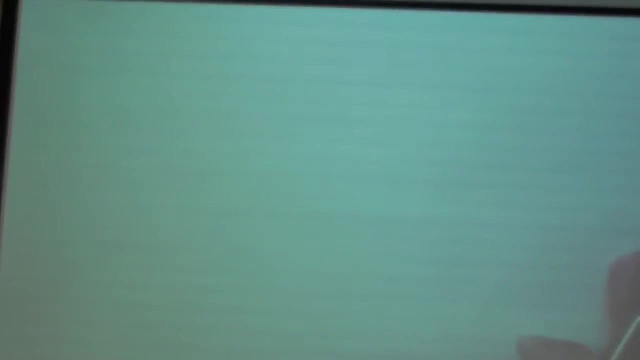 it's not exactly a proof, Because the actual proof is really technical and Kevin already proved that last week. Many of our results were proven last week, So switch. So at this point I will actually switch back, then I will switch back. Let me make sure that line is correct. 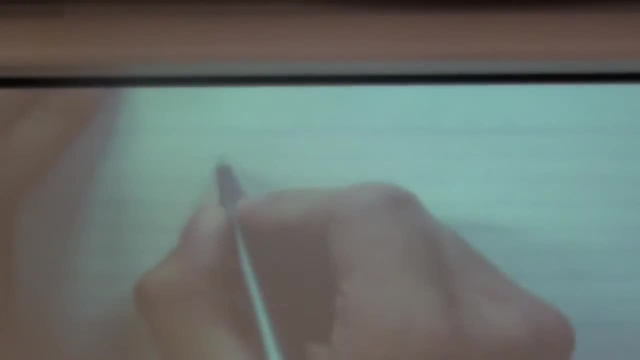 Oh good, So our first step of working towards modifying the solution- sorry, the one in the block- is to modify the solution. So our first step of working towards modifying the solution- sorry, the one in the block- is to modify the solution. 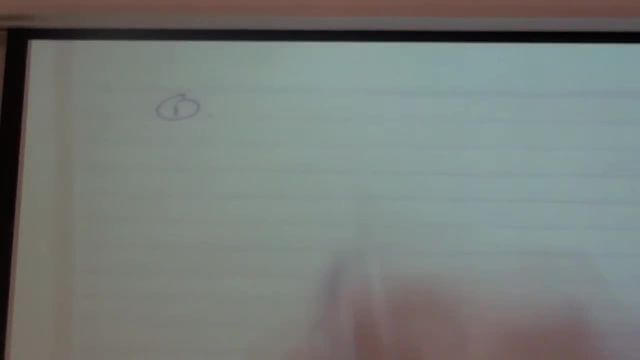 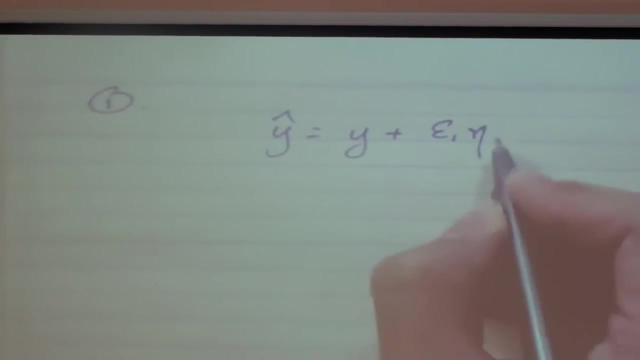 Sorry, the one in the block is to modify the solution, So it will double the operation. First step: we are going to write Y hat. You can see our Y has a three variables and it is made up of Y plus epsilon 1, eta, 1.. 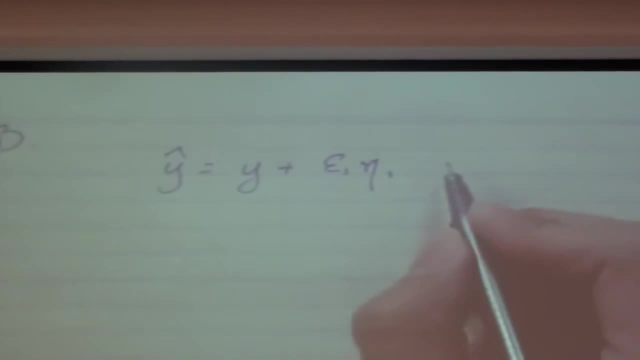 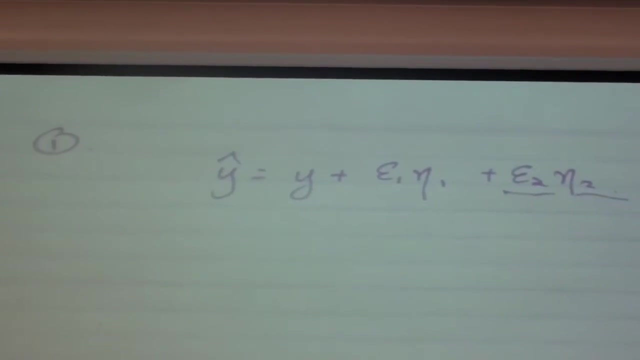 That's what we had last week. but now we have anfia term here: epsilon 2, eta 2.. Why do we have the simply? Well, the reason for that is simple. Later we will substitute Y hat into this constraint here. 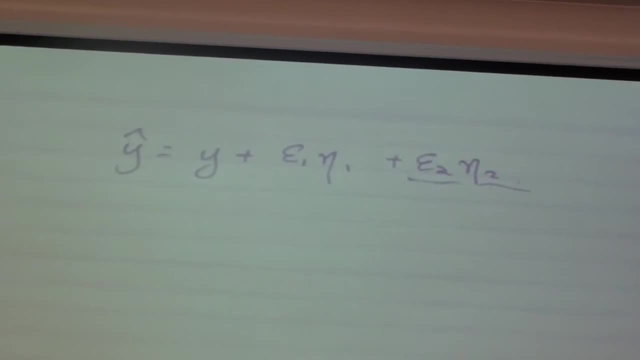 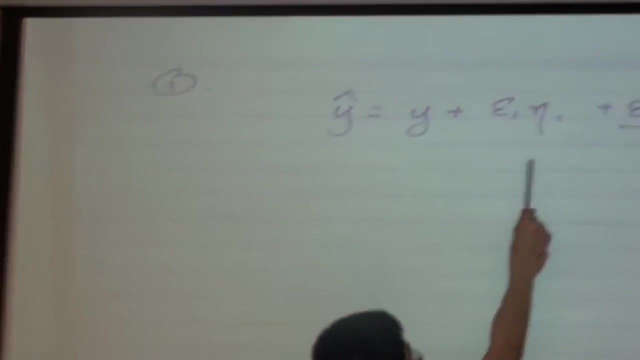 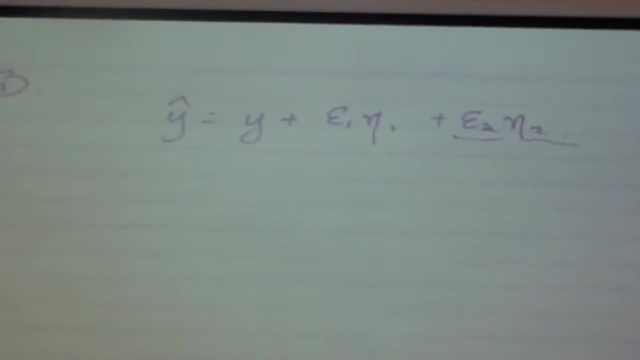 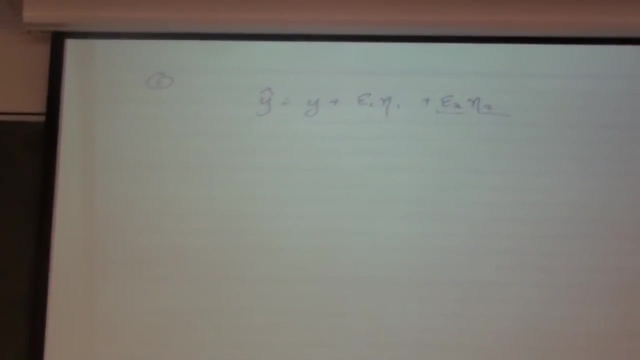 Later we will substitute Y hat into this constraint here. But if we actually do that, we're actually making an assumption that those two functions- eta2 and eta1, they both satisfy the constraint. Now that's not the case because, as we see very soon, we'll actually apply the fundamental lemma of first variation. 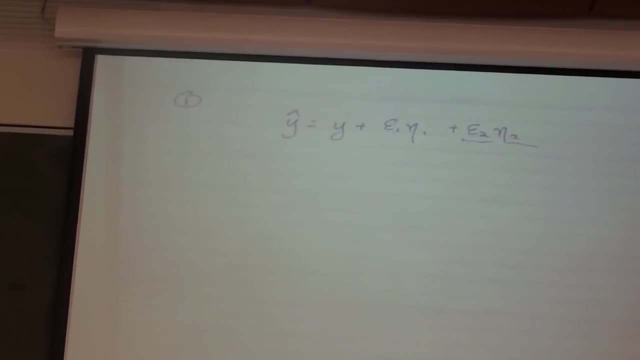 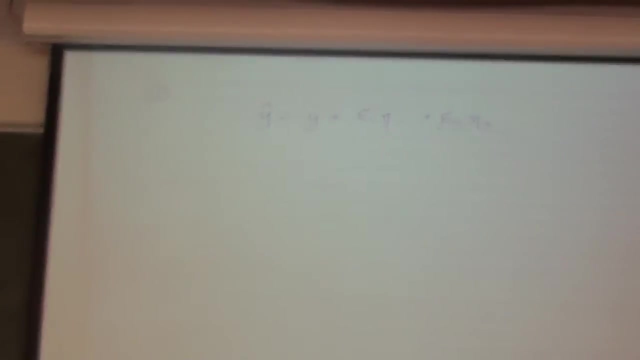 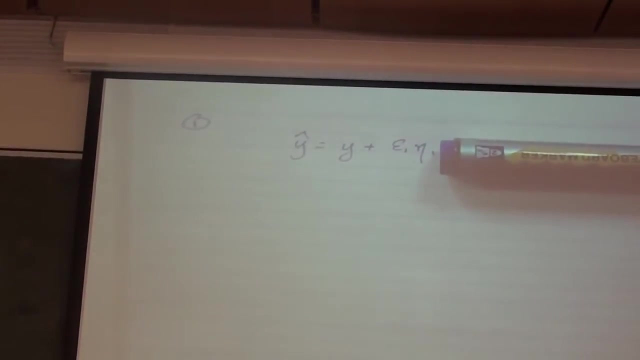 If we want to apply the fundamental lemma, we'll run into a problem, because the fundamental lemma assumes the arbitrary nature of eta1. So if we don't actually have the eta2 and epsilon2, if we just have that, well, the y? hat must satisfy this constraint. 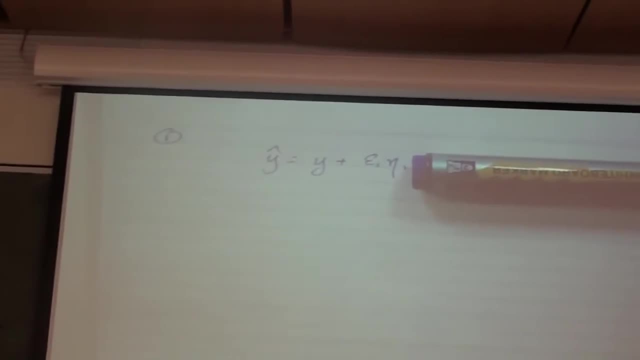 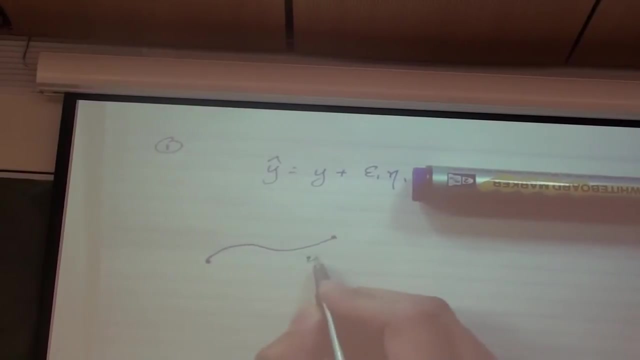 So eta1 cannot longer be an arbitrary function and the fundamental lemma is not a constraint. So perhaps I can do a little diagram to illustrate what's going on. So imagine there's two points of space. Okay, that's our optimized function y and it has to live out. 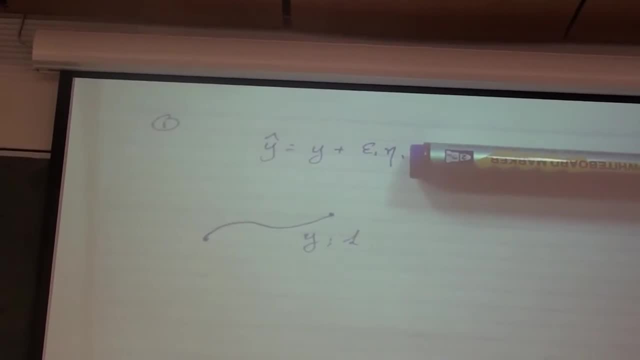 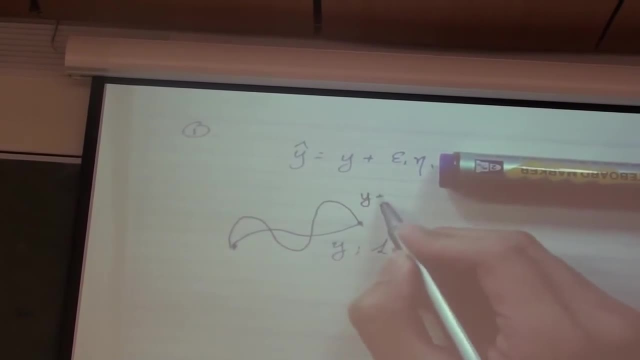 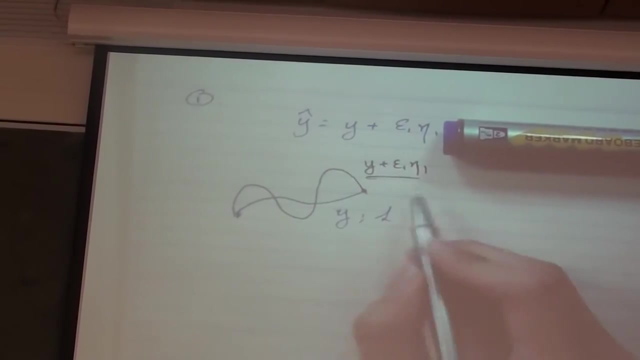 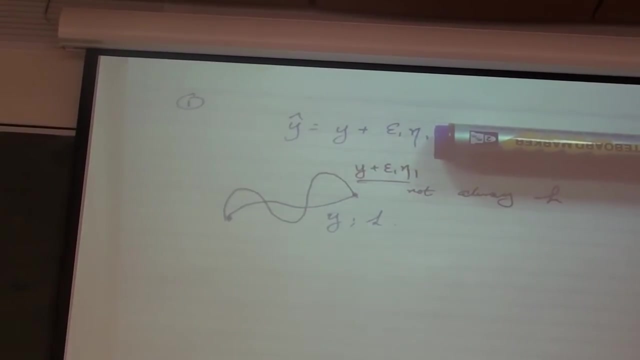 And that's great. that satisfies the constraint. But now if we just consider y plus epsilon1, eta1.. Now this, This function here, does not always give you l, That's not always satisfied the constraint, Because, as you can see, even though they have the same endpoints, the length of that is much lower than the extremal. 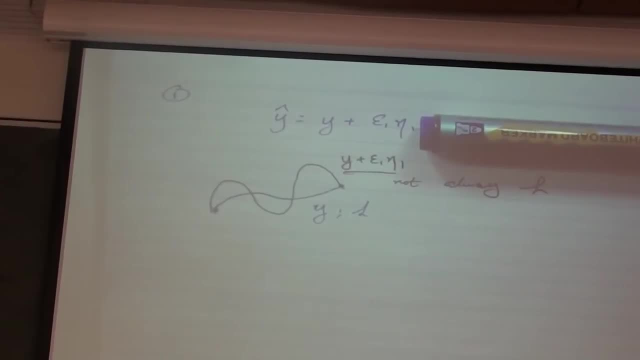 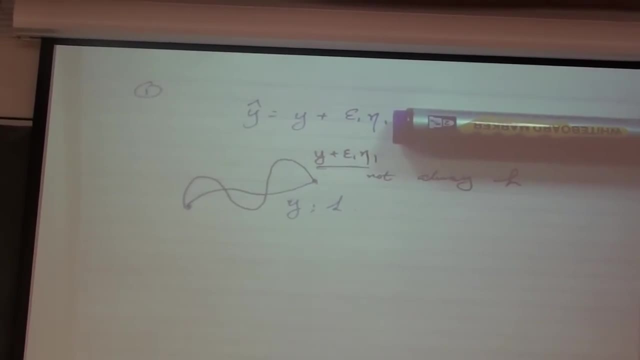 And since the extremal equals l, the new function you have here cannot be equal to that length. So to counteract that problem, we give that- We introduce epsilon2 eta2.. What it does is this: It's that it corrects. 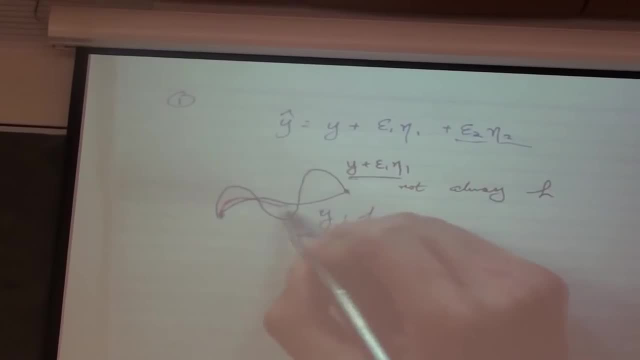 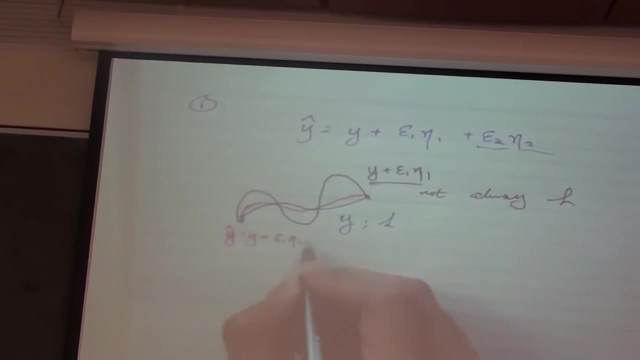 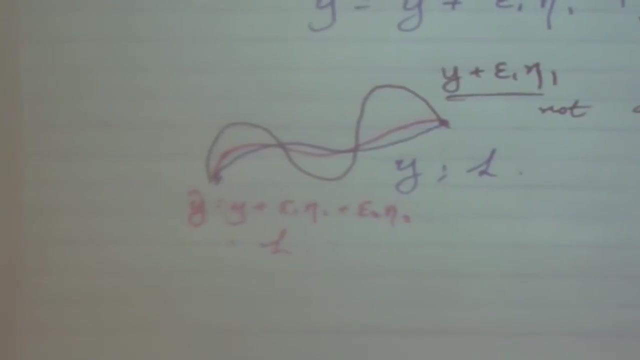 Okay, it still has some resemblance, of course, But here we have y, hat equals to y, plus epsilon1, eta1, eta2, eta2.. That will give you l. So what's really going on is: imagine that eta1 and eta2 are having a conversation. 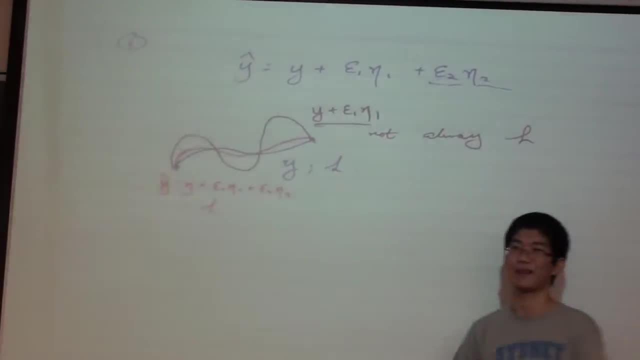 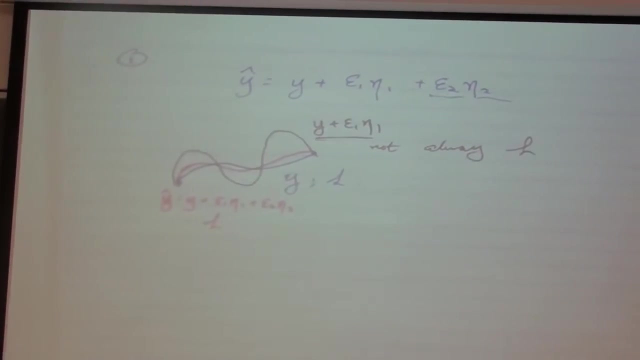 And eta2 says system eta1, just be whatever you want, Whatever. What a mess You overshoot. You overshoot Whatever. right, I'm going to clean up your mess. I'm going to make sure, overall, we're going to satisfy the constraint. 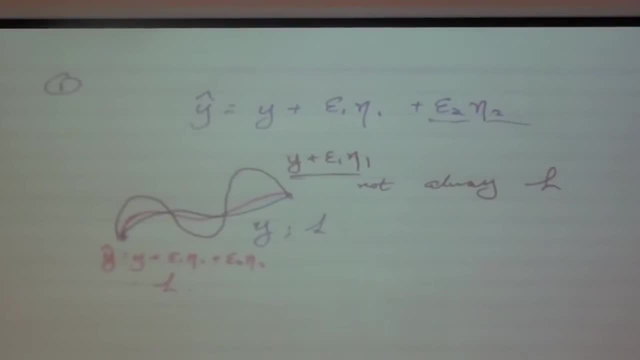 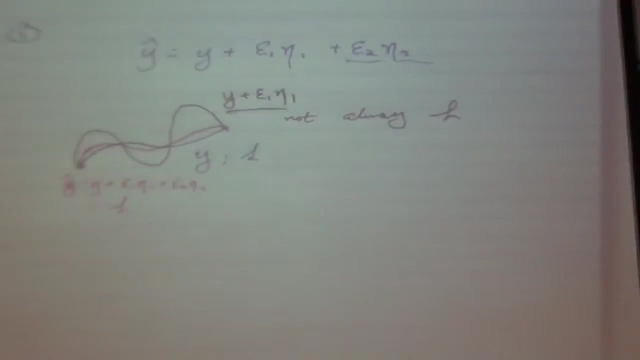 Overall, we're going to satisfy this l. So you can think of eta2 as being a correct return. It corrects the l-word estimate or underestimate of eta1.. So eta1 retains its arbitrary nature. Let's switch back. 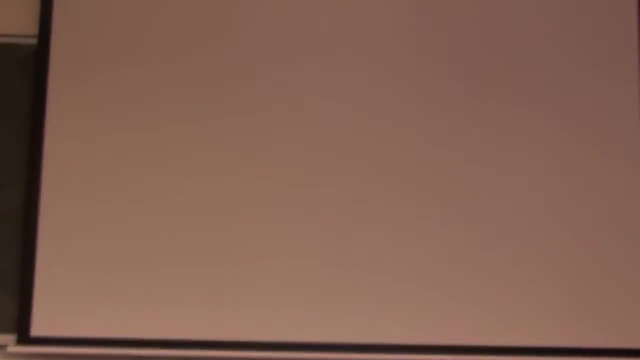 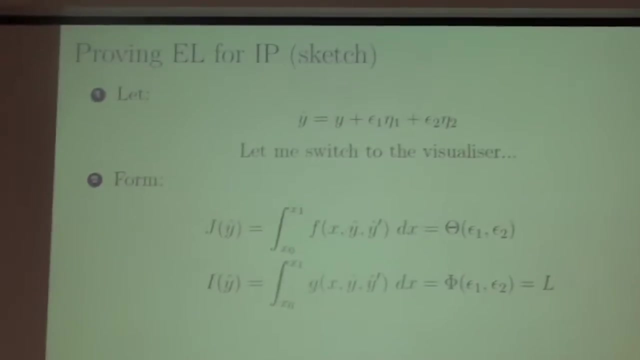 I look like my mom because she always clean up after me. Okay, so once you have that, of course, you can substitute y hat into j and i. Now, once you have those two, you have this horrible integral, But don't worry. 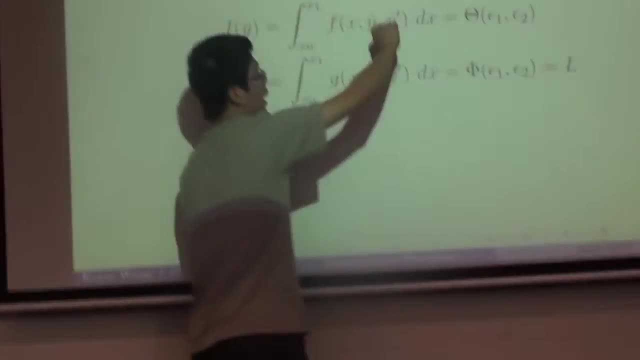 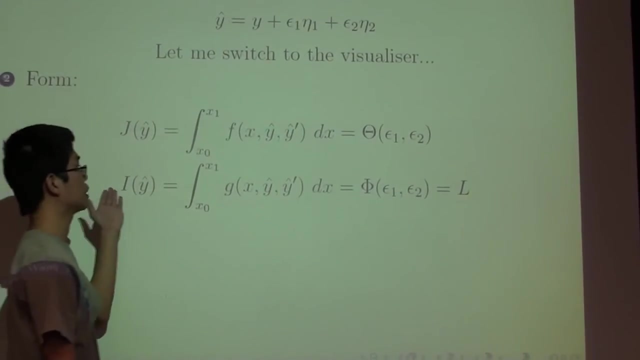 We don't care about that, Because we can consider the whole integral as a function, taking epsilon1, epsilon2 as parameters, And the same thing happens for i of y hat. That equals some function, capital phi, taking epsilon1, epsilon2.. 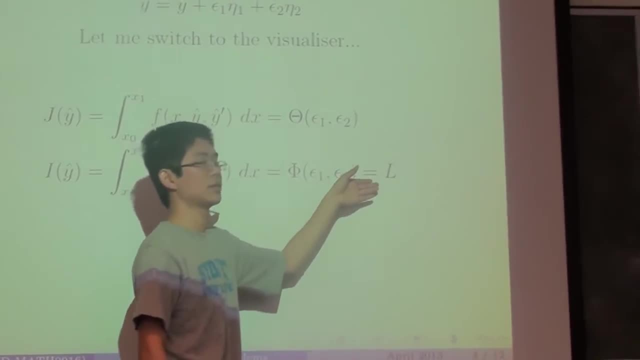 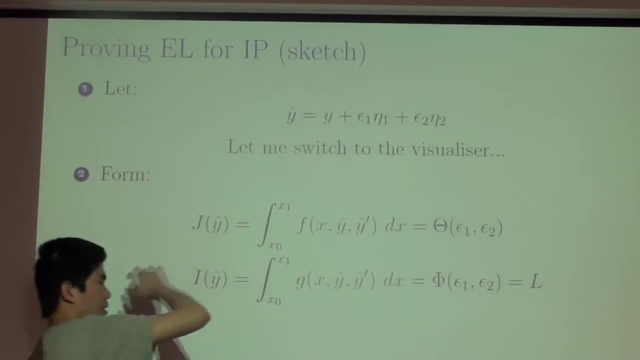 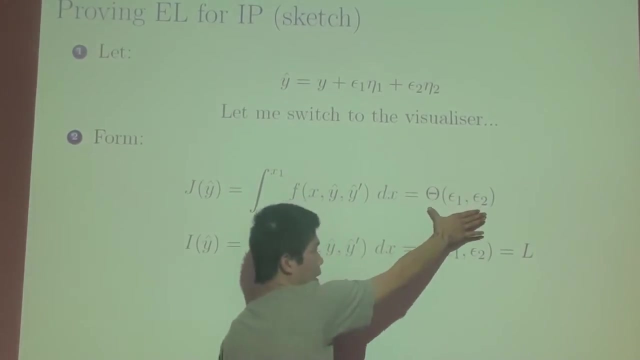 So let's take a moment and think. Our problem of optimizing a functional under the constraint of another functional is now reduced to optimization of this function under the constraint of this function. So we happen to have just done the watchable test class before. 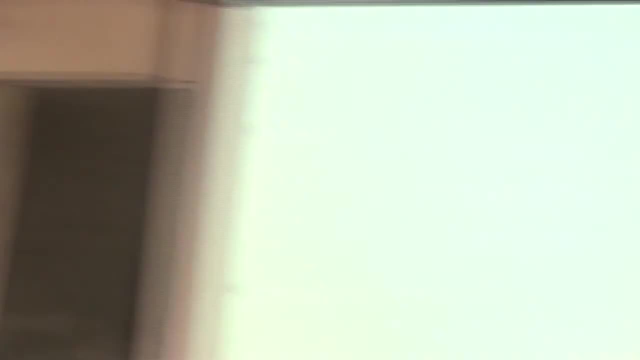 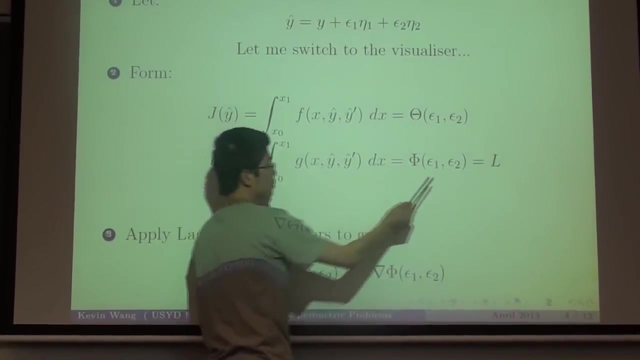 So our equation is applied simply like that. We want to optimize this, So we take a graph. So we take a graph of this Times, some constant lambda, The graph of all of that. Of course, we need to apply the graph operator or del operator. sorry, 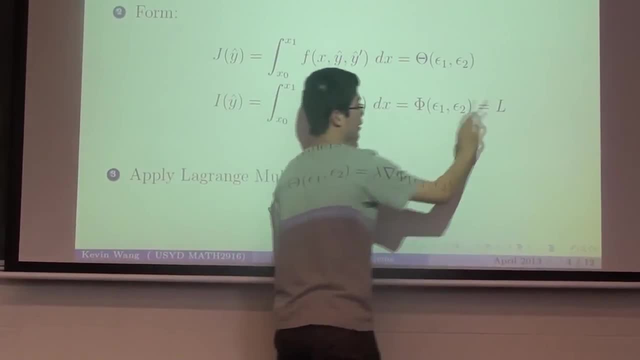 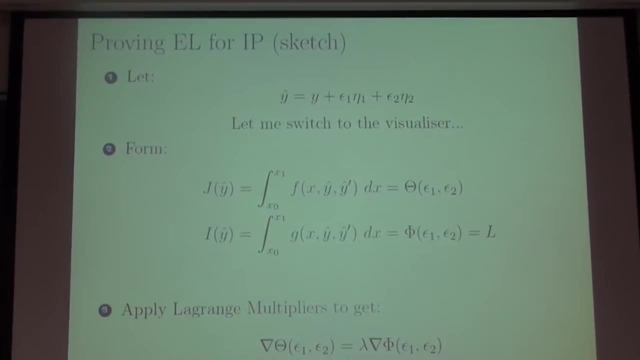 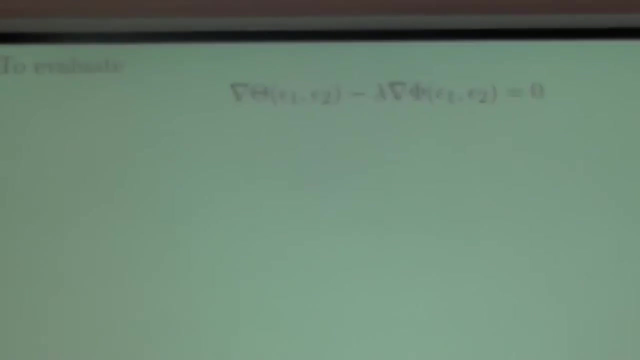 The del operator on capital phi minus l, Of course l goes to 0.. So you essentially have this formulation. So that's great, Because now we're going to evaluate this thing. That's a terrifically wonderful and difficult to evaluate. 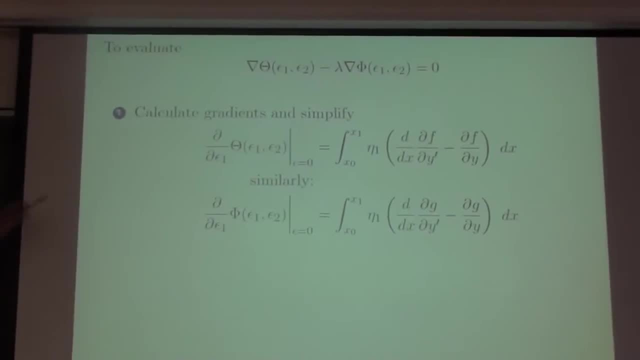 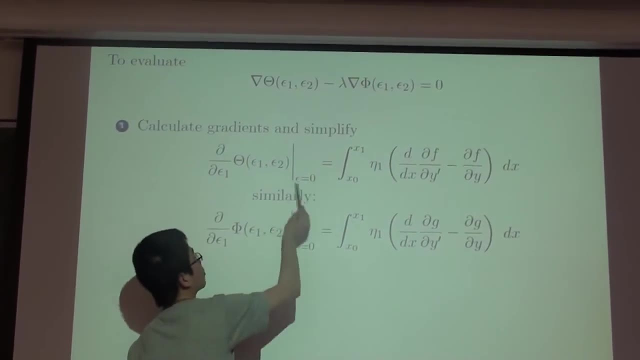 That Kevin did that last week. So I'm going to probe this result And the result simply goes like this: That this is the result from last week. You evaluate the partial, Evaluate at the point epsilon equals 0. Which means epsilon y equals 0. 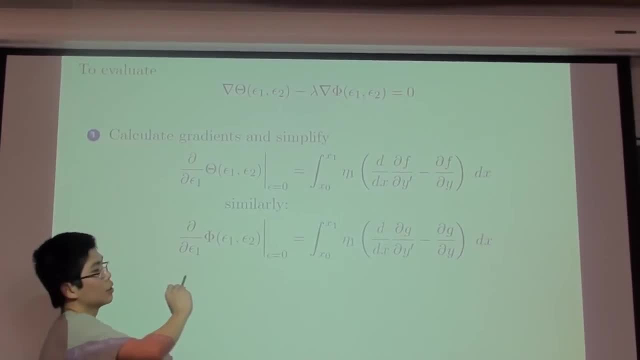 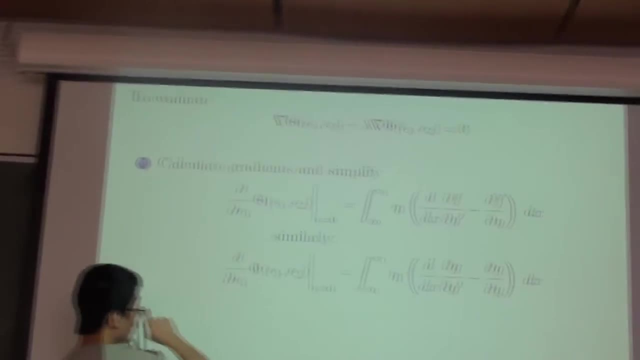 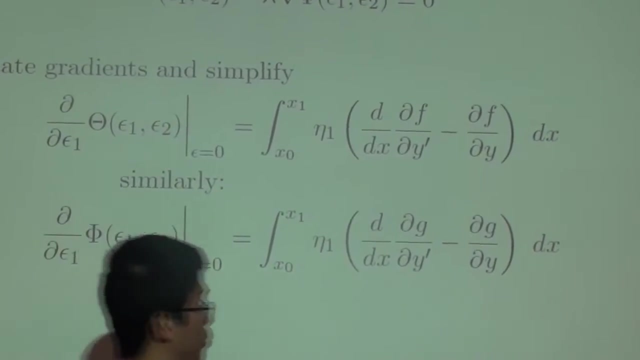 Epsilon 2 equals 0. Because when you have that, you actually get the extremal. Now that increases that equation there, And if you do the same thing with the function capital phi, you get this integral. Now notice that last week we stopped here. 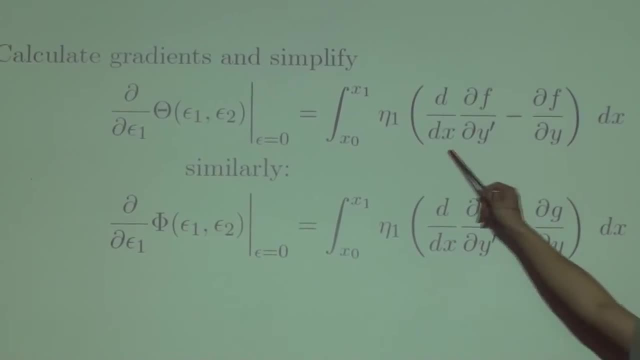 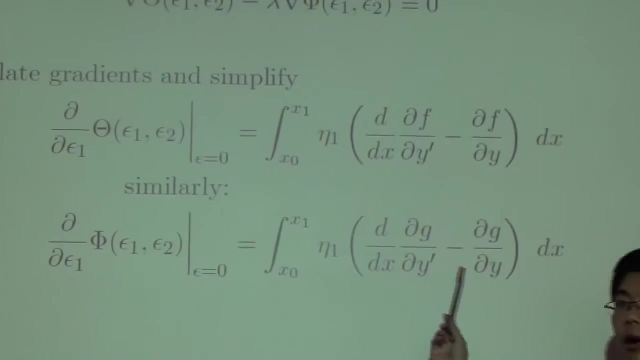 After this one, we stopped here and claimed this equals 0.. And you can probably see that already, That this is the Weiler-Lagrange equation for this function f. And here we have the Weiler-Lagrange equation for function g. 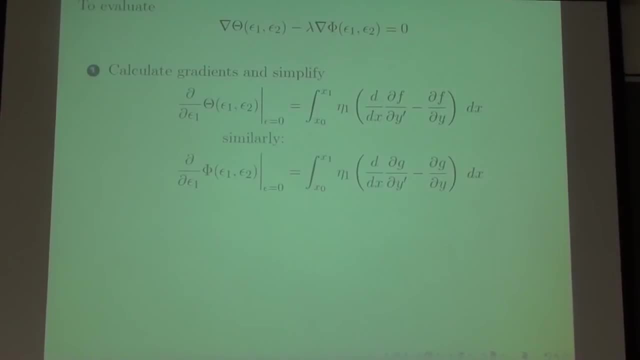 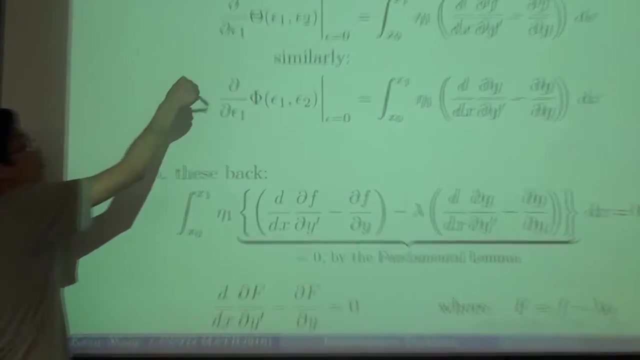 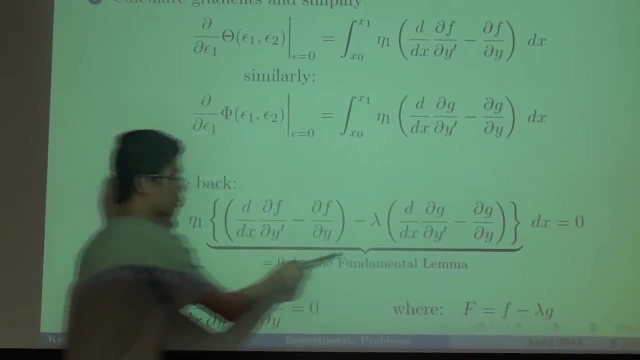 But this is the last week, So we actually go a little bit further this time. What we have now is that we're going to substitute these two results into our original Lagrange multipliers equation And you get this horrible expression. But the good thing is that we can apply the fundamental lemma now. 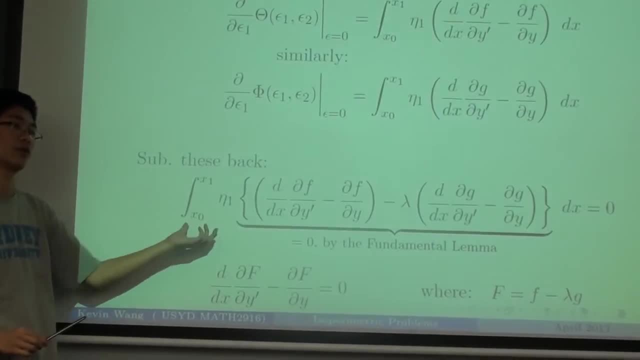 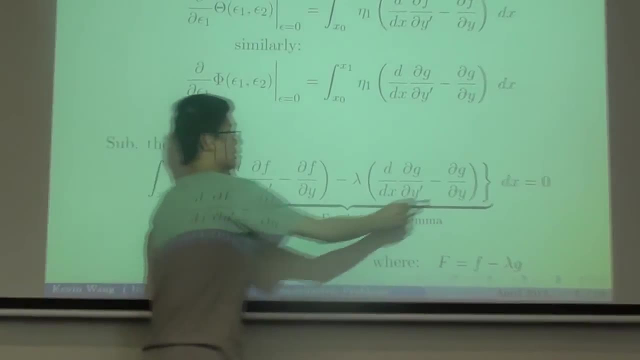 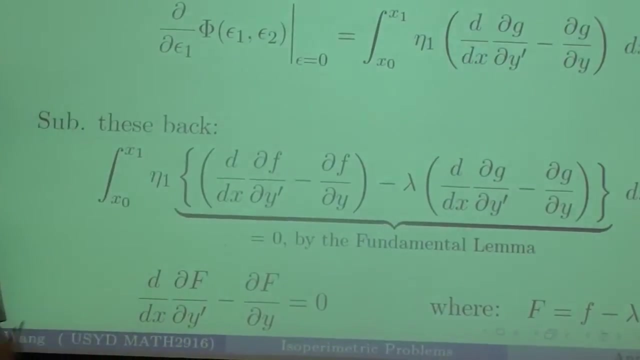 Because this eta1 that went out is now an arbitrary function, So applying the lemma is perfectly fine And, of course, when you apply the lemma, what's inside the braces goes to 0.. Okay, it becomes 0. And yes, that's a horrible expression to write out again. 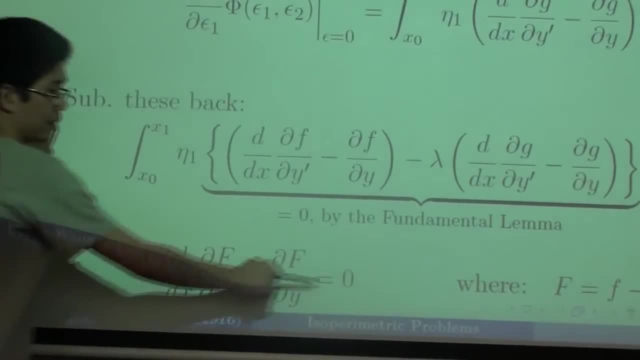 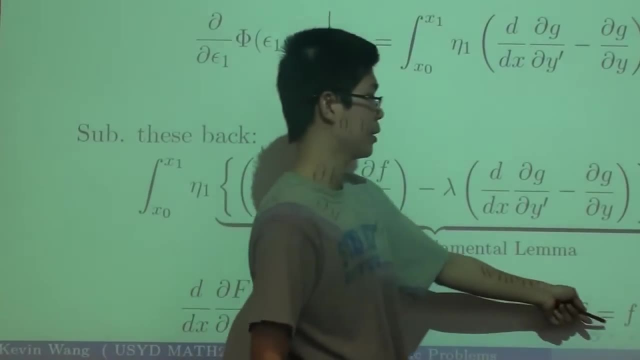 But we can succinctly write that in this form: Okay, so that's essentially the Weiler-Lagrange equation applied on some function, capital F, Where capital F is simply little f minus lambda g. So this is actually the second theorem I have today. 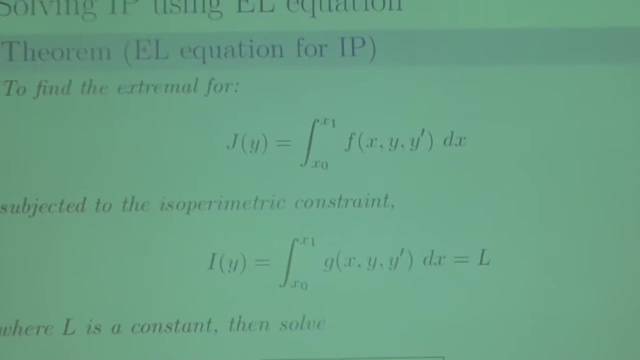 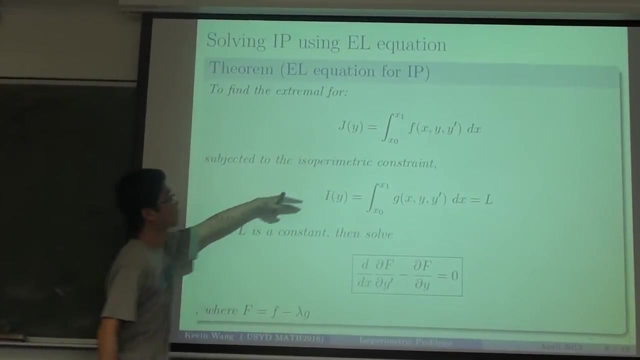 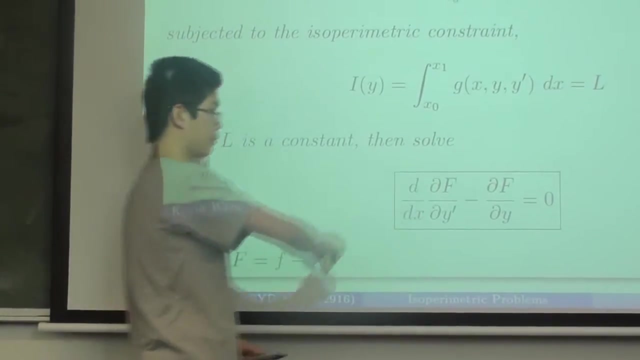 And this summarizes what we've done And the sum of. Yeah, there you go. It says that if you want to optimize j of i under the constraint of i, y, it was L, And then the Weiler-Lagrange equation applies on some function, capital F. 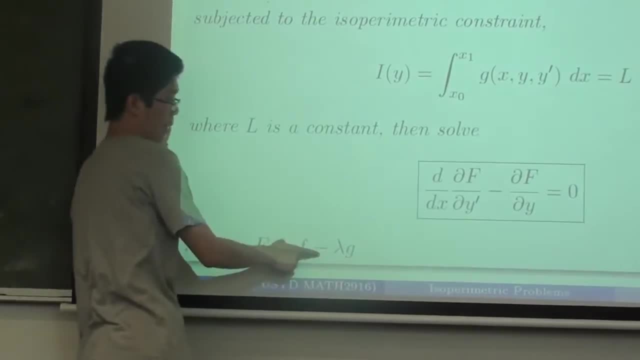 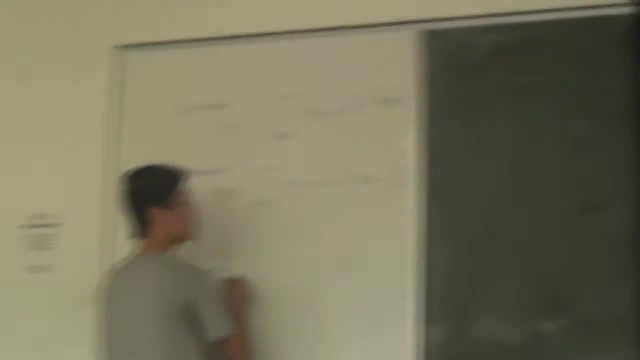 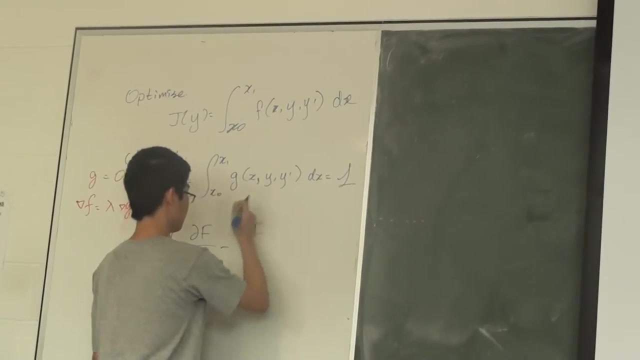 Where capital F is simply the integrand of j, minus some constant lambda times- g, which is the integrand of i y. So let's put that up: It's partial f, partial y, hat minus partial f, partial y, which is 0.. 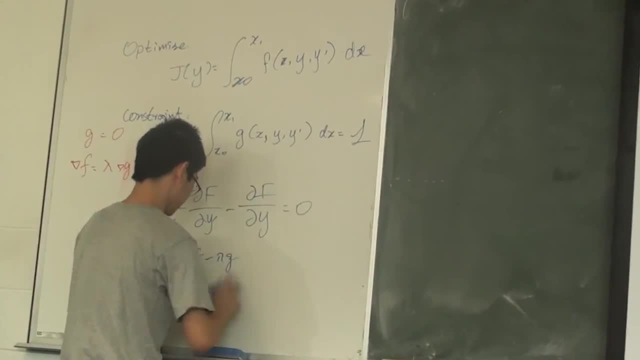 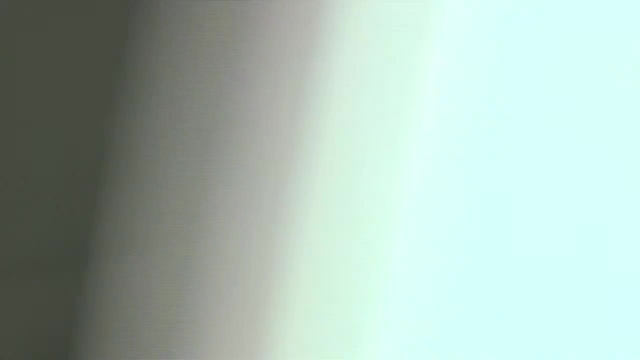 And where the function capital F is little f minus lambda g. So this is why I didn't do a rigorous proof at this point, I only sketched the proof. It's because here is the Weiler-Lagrange equation, applied on both f and g. 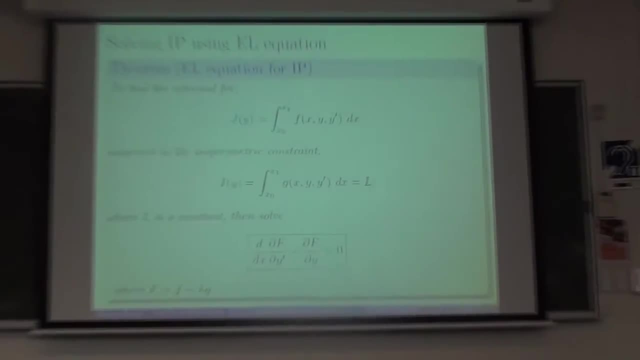 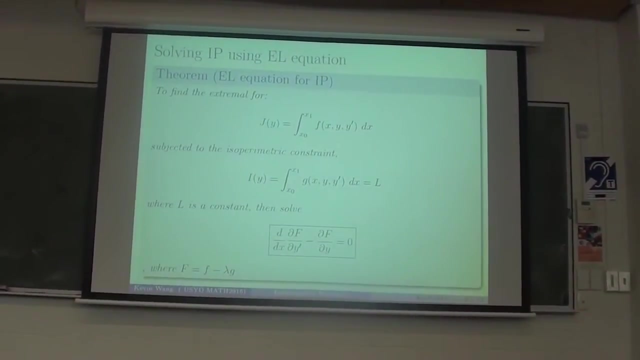 So essentially I'll go write this out. It'll take a long time, but essentially I'll be doing the same proof that Kevin did last week twice. So there's not much insight of what's going on, But this is good enough for us, because now we can use this to solve a problem. 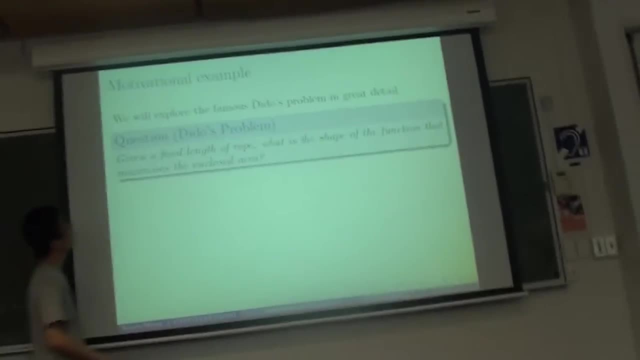 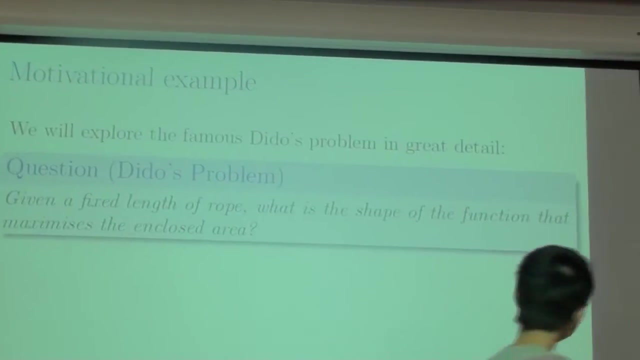 So here's where the audience participates. How are you guys? So I know I have a diode problem And the thing is that people have a fixed length of rope. What is the shape of the function that maximizes this enclosed area? 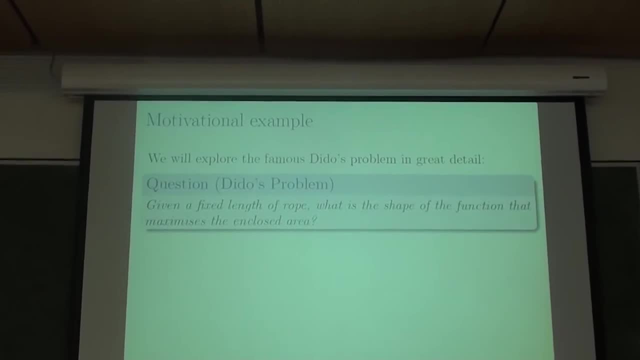 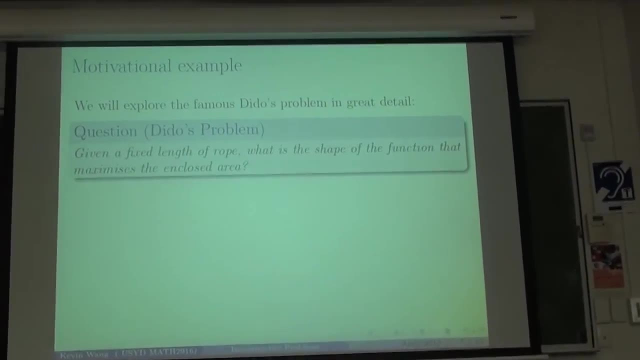 Anybody have a guess? Circle, Yeah, I ask a lot of people about that question during the week. All of them say circle, but none of them actually tell me or justify their claim. So now you know, I'm going to prove this now. 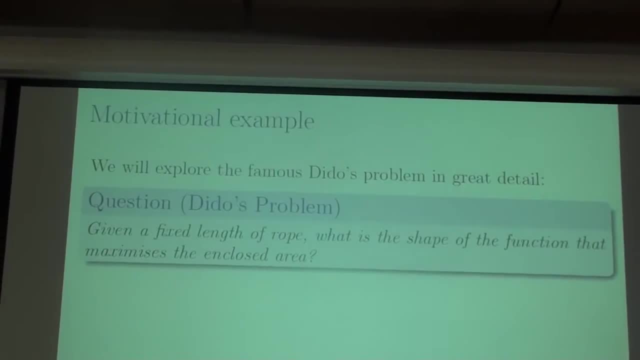 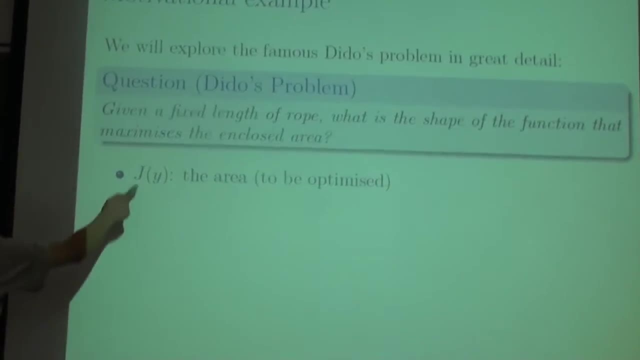 And you can probably show this to someone in your party. Maybe that's what you should do. So just by looking at the equation, we know that j y is the thing we want to optimize. So just by looking at the equation, you know everything. 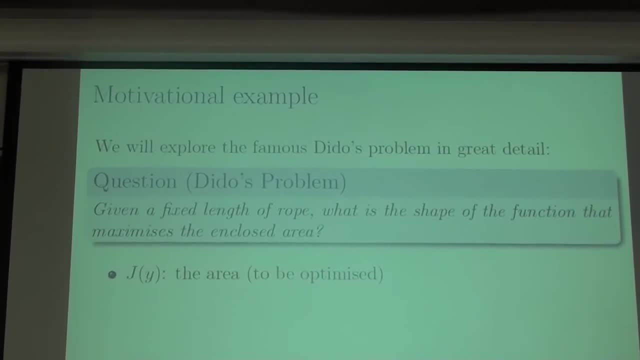 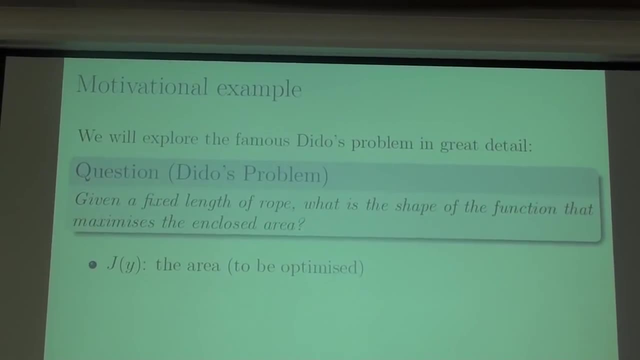 So just a question: Are you looking at the closed row- Enclosed curve. It's an enclosed curve. In this case it's going to be two-dimension. I should mention that It's two-dimension, because, Two-dimension, I don't know what's going on. 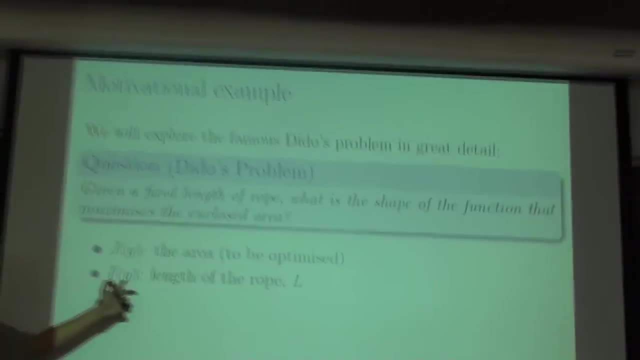 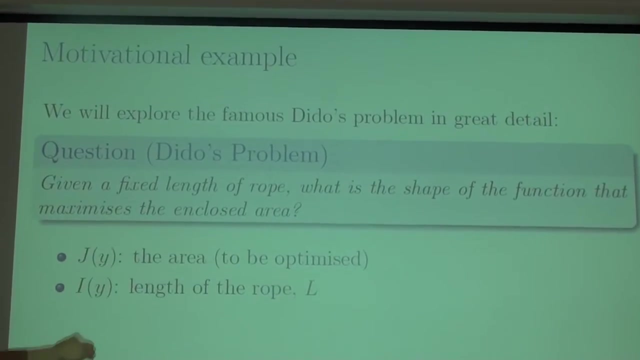 No, okay, don't see that. Okay, sorry. So I have y, which is our isoprimitary constraint, which is the rope of fixed length, Fixed iso length, perimeter. So you see the resemblance here already. 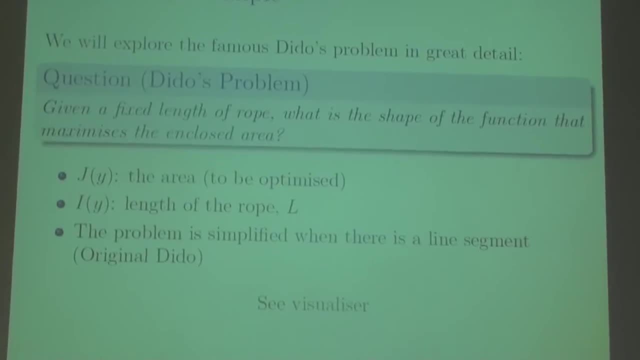 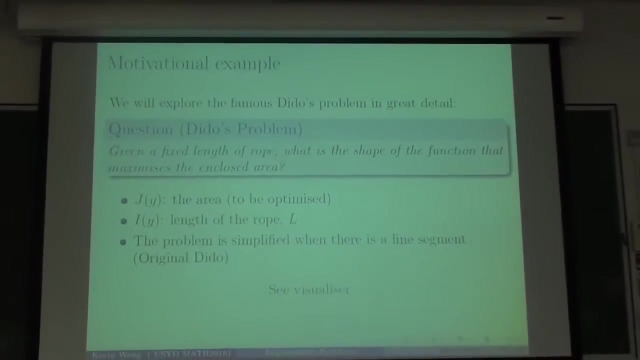 This is the isoprimitary problem And of course we can actually simplify the problem a little bit. And this is actually the original Dinos problem in I don't know how many years ago. So here we're going to have to switch back to Visualizer and do this. one more problem. 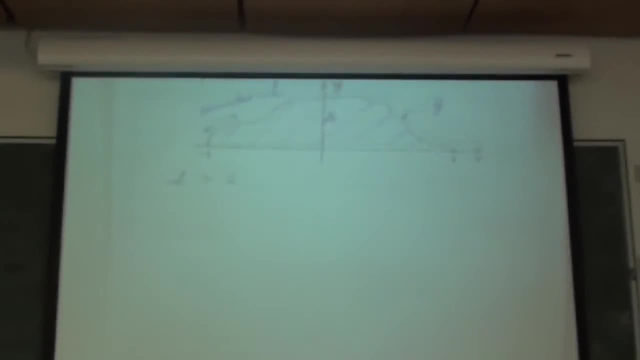 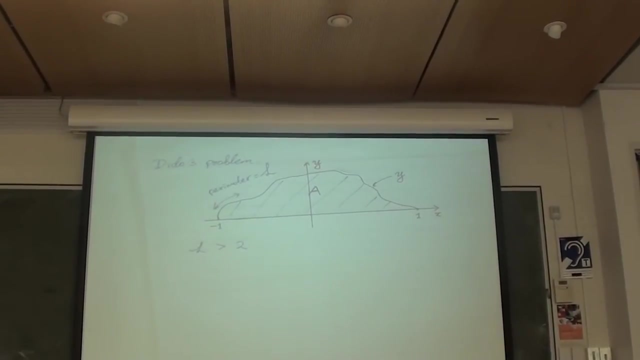 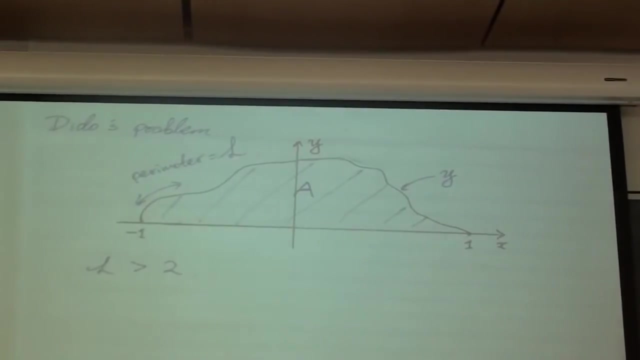 So here is the diagram I prepared earlier. because I can't draw, Let me just remove that. Okay, that is the problem, And what I've done here is to simplify the problem a little bit. What I have here is that, well, whatever length of rope you have, you give me. 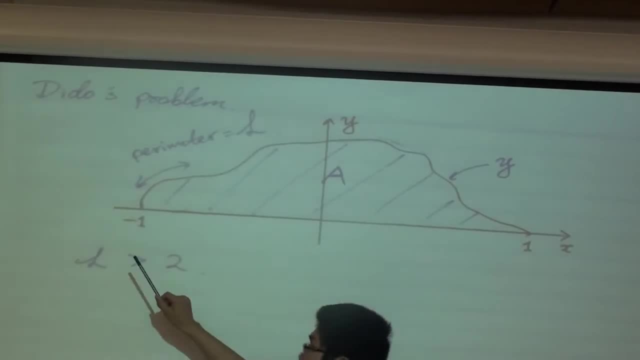 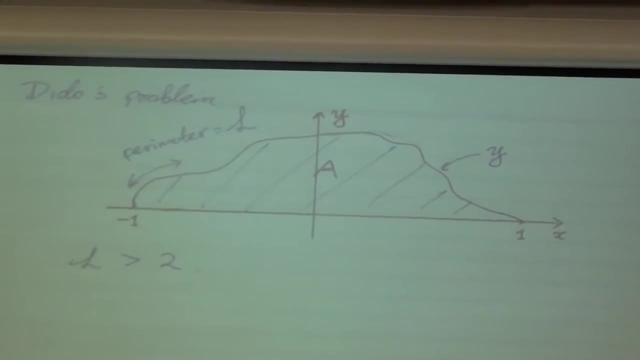 I can rescale that. I can rescale that between the unit, I mean between minus one and one, And I can properly carve my curve into half and I would only consider the top half, And this function is called our y. 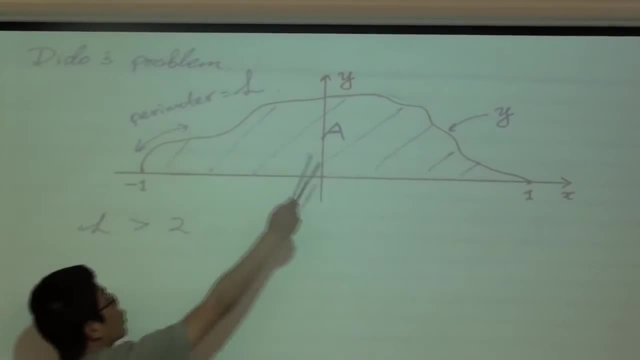 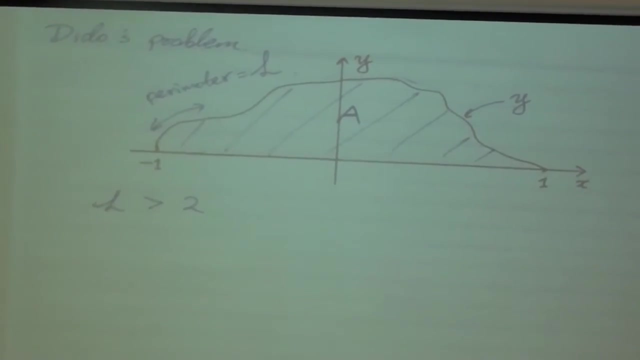 As an enclosed area between the function and the non-second, between minus one and one And the perimeter. if you give me that, that's going to be L. Now, one thing I should mention really quickly is that L should be greater than zero. 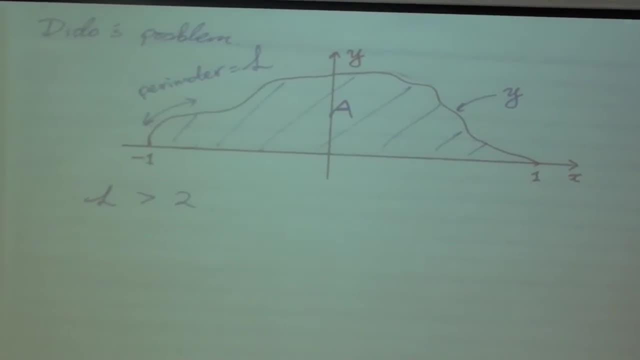 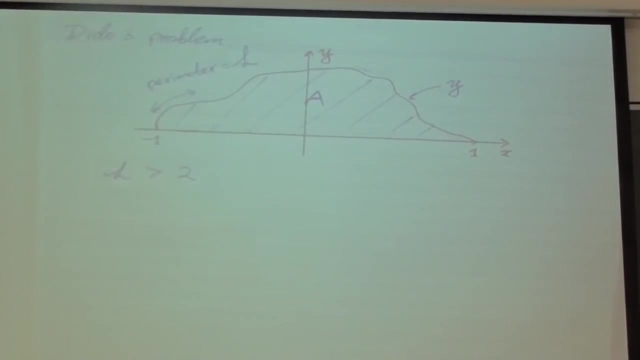 Okay, So greater than two, For the reason that if it's actually equal to two, then minus one and one, you know that's just a geodetic. There's nothing really funny going on. And if it's actually less than two, I'm sorry. if it's actually less than two, then what happens is that you don't even have a geodetic. 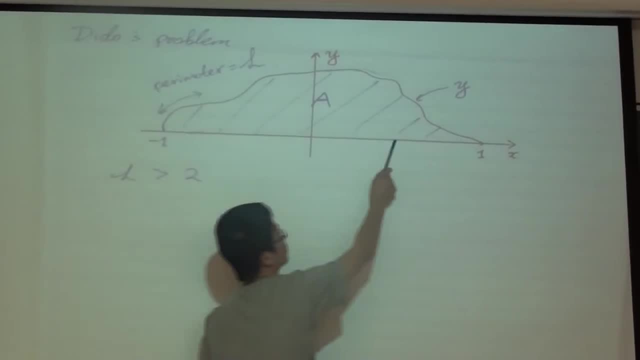 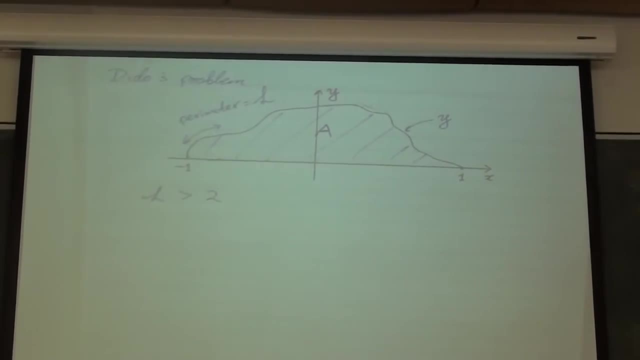 You know, you just go and go for minus one here and stop and never reach that point. So that's no interesting problem. Okay, so it's up to this point. Let's do something fun Now. we established that j of y, what we're trying to maximize is the area. 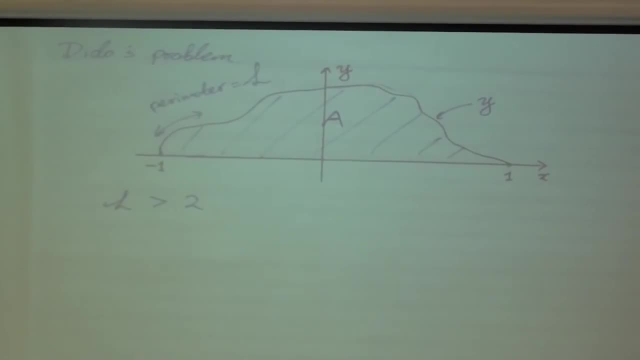 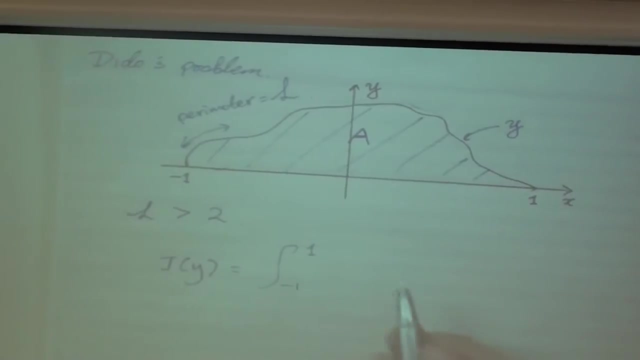 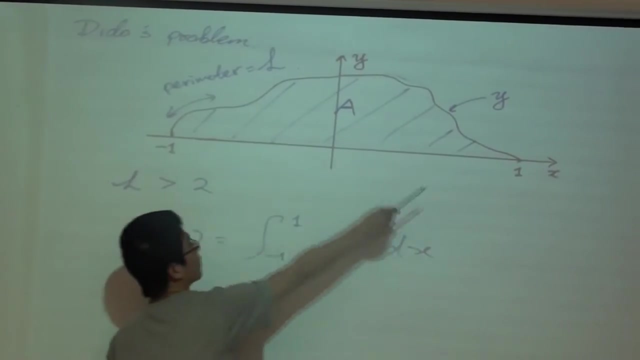 So let's write down the area for this curve here. Audio participation: anyone, No one. Oh nice, It's going to be the area under the curve, because we only have that y Of course again, I should really quickly mention the perimeter. 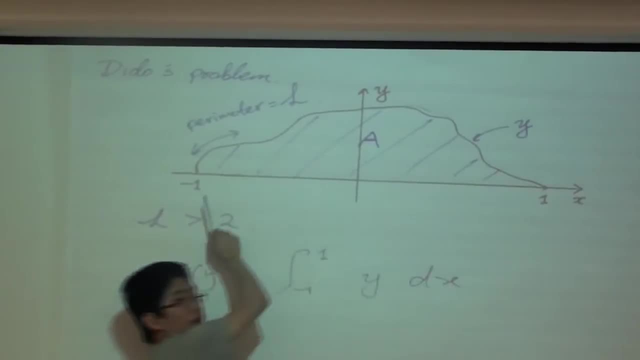 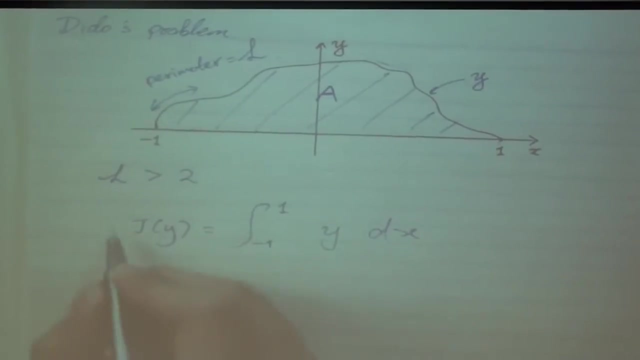 That's no count. Okay, It's minus one to one line segment. We don't consider that. So this is our area, And now we have the constraint y of y, which is between minus one and one. Now, this is our perimeter. 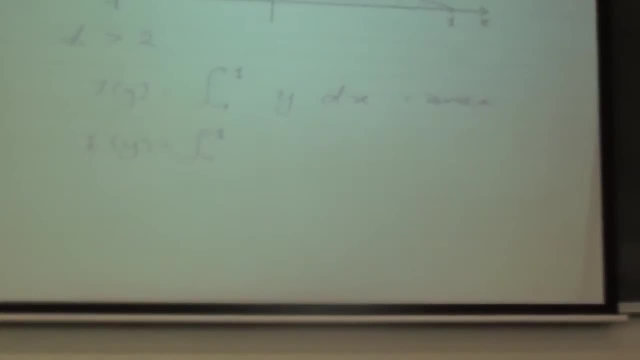 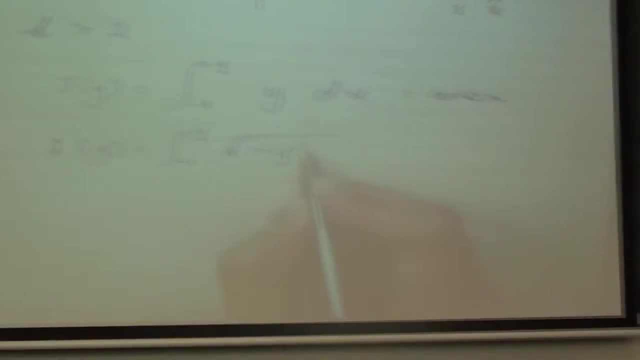 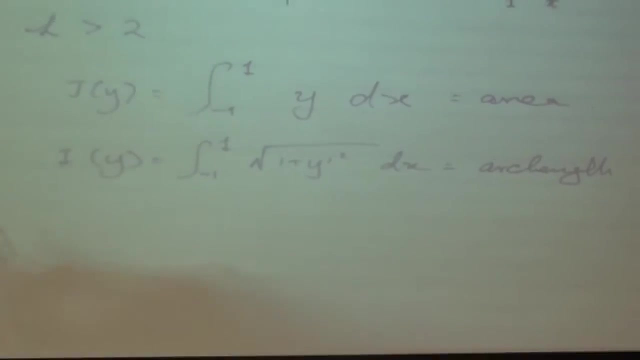 And perimeter. essentially that could be considered as arc length. So here is why I'm going to call my arc length formula: And that is just minus square x, x equals arc length. Oh, that's great. We have formulated j and i. 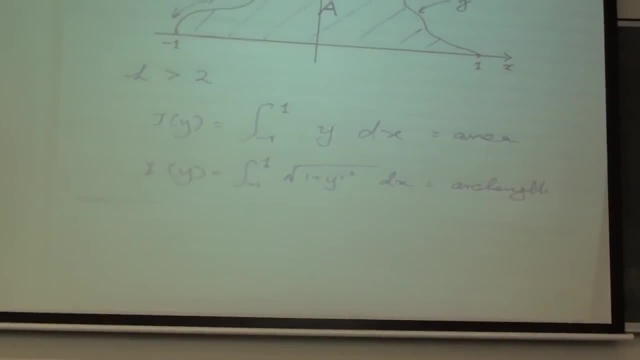 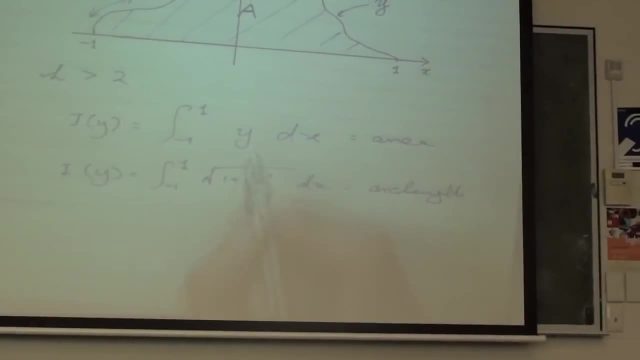 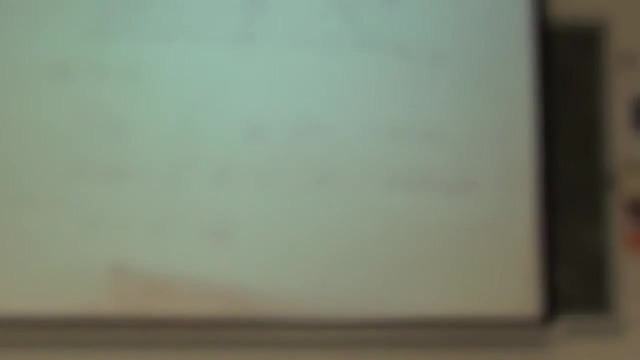 Okay. So now we actually want to apply our theorem, And our theorem says: the capital F that we're going to be applying on is little f minus little g. Now, little f is that and little g is that. So capital F equals to little f minus lambda g. 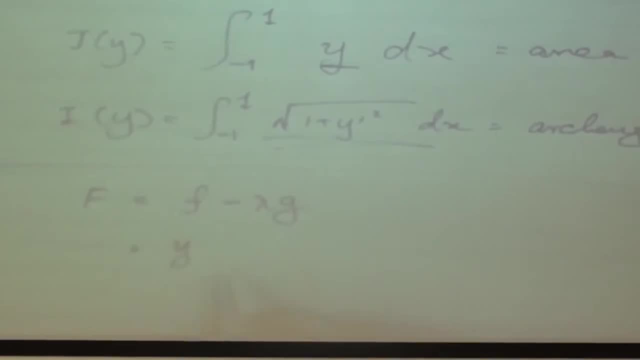 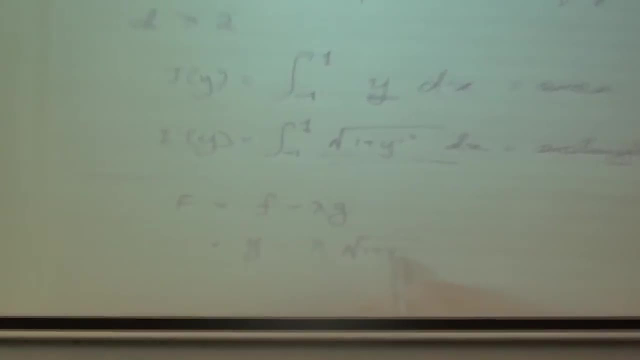 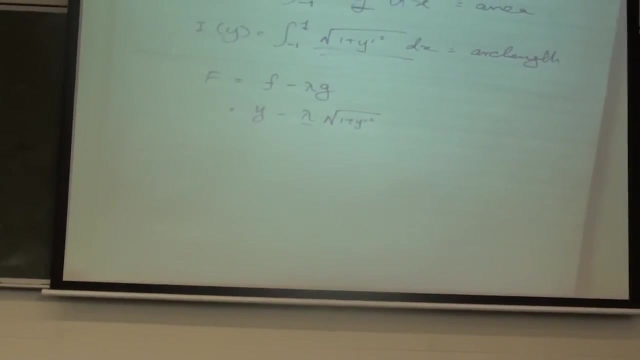 We would get y. Okay, That's that Minus lambda. It's a constant And g is simply the integral of five. So this is what I have And here, Oops. Here's why I would like to apply the Lagrange. 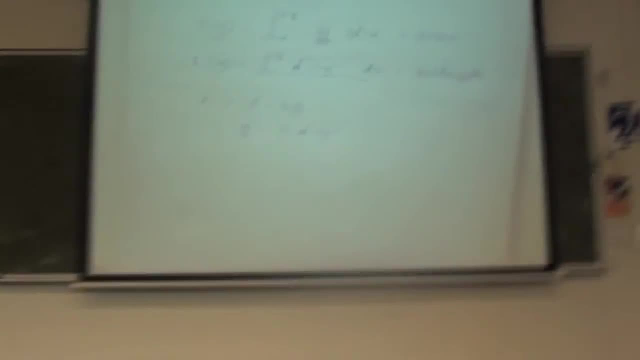 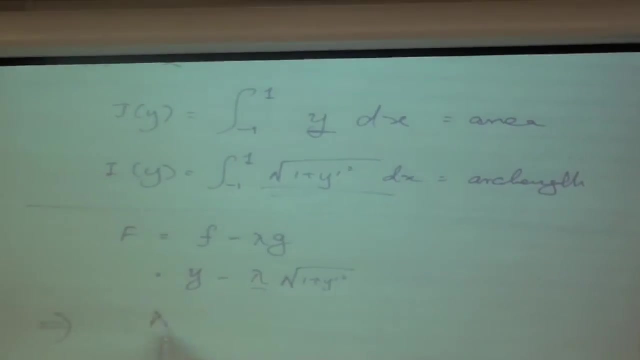 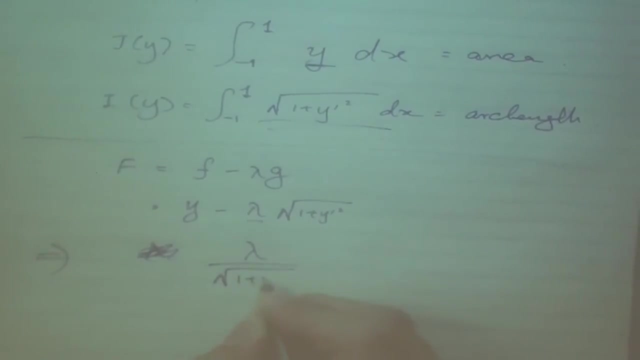 The Euler-Lagrange equation onto capital F. If I apply that, this is the result you should get. This should be lambda, Sorry, Lambda over square root of one plus y. y. dash squared plus y plus c1.. Where c1 is some constant. 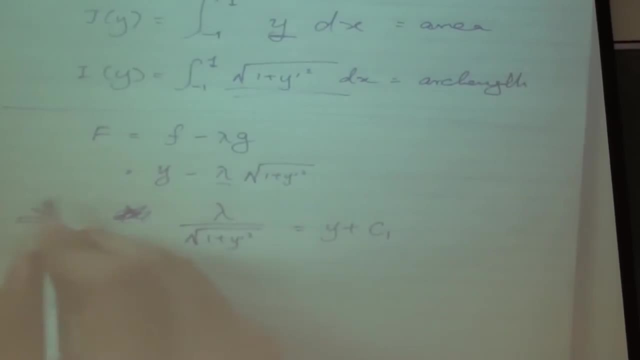 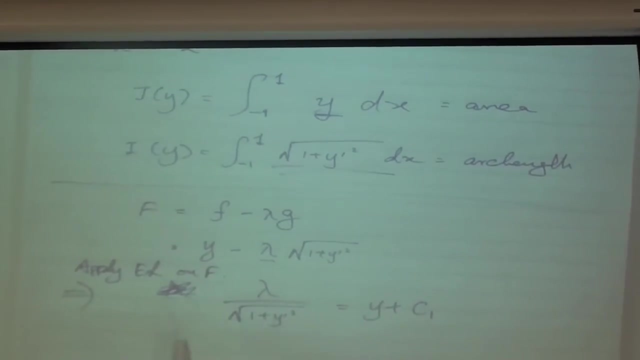 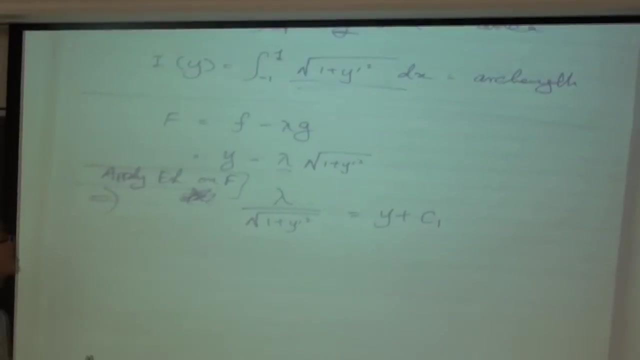 Integration constant with f. So this is about applying the Euler equation on the function f. This is what I did. Now this equation is a differential equation. Great Dana still asked how to do that. Anyone have a guess of how to solve this equation? 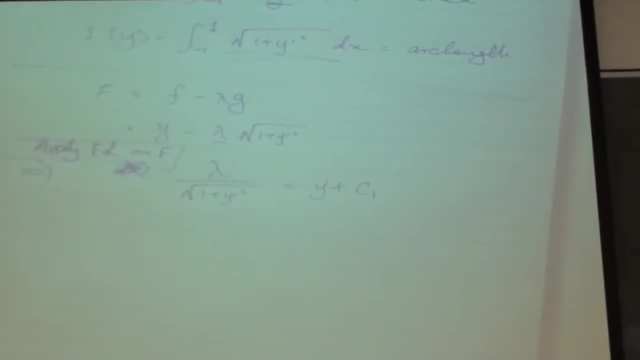 I was expecting participation, right? So we know that y dash, We can actually separate this And one do this. you will see y, I can separate this. Well, I will do d, y plus c1, squared divided by y plus c1.. 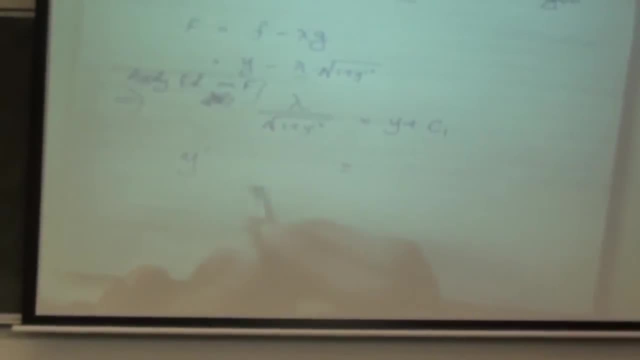 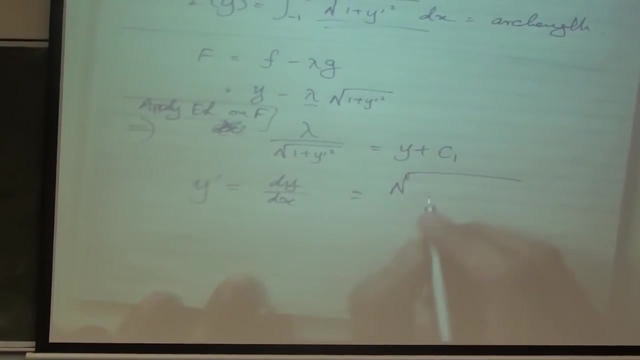 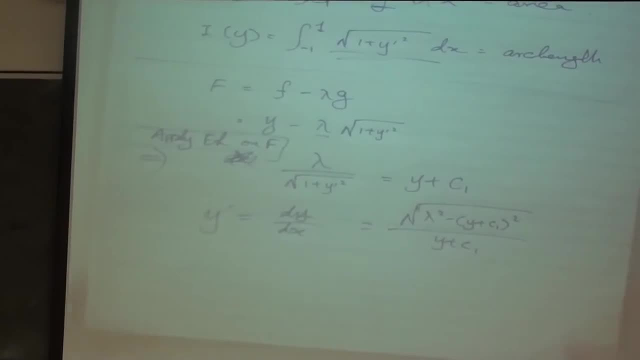 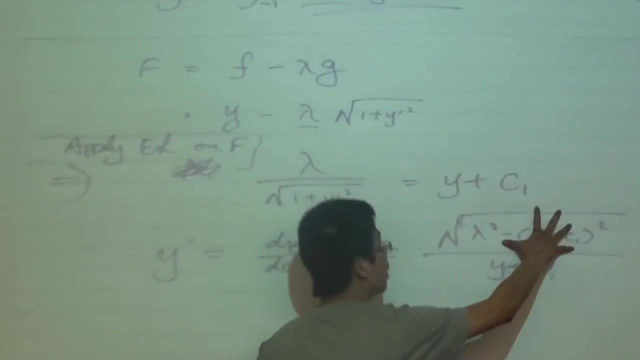 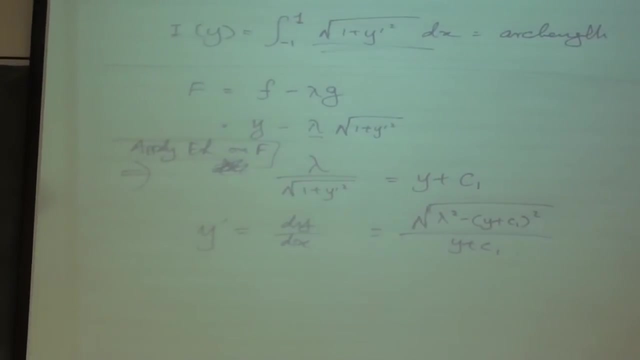 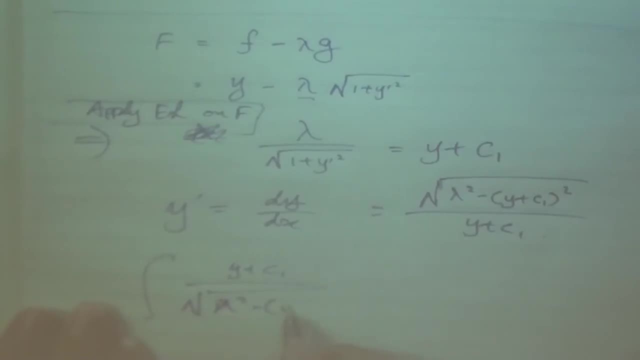 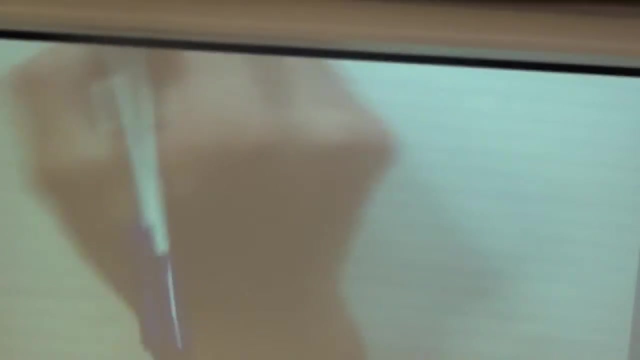 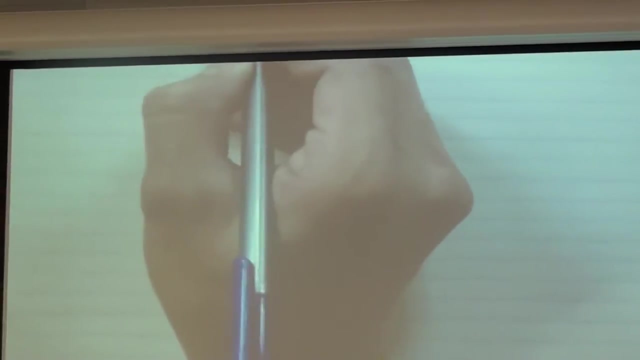 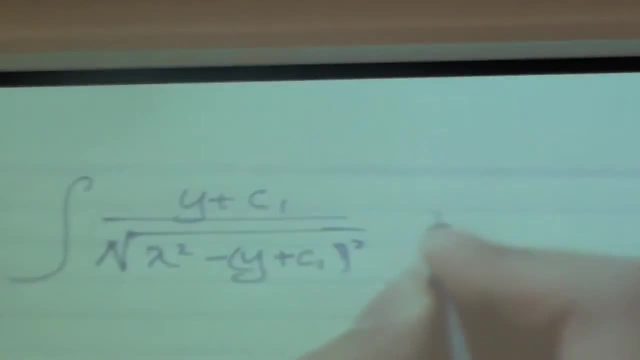 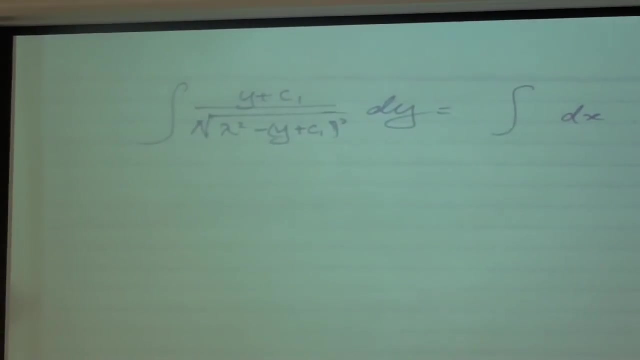 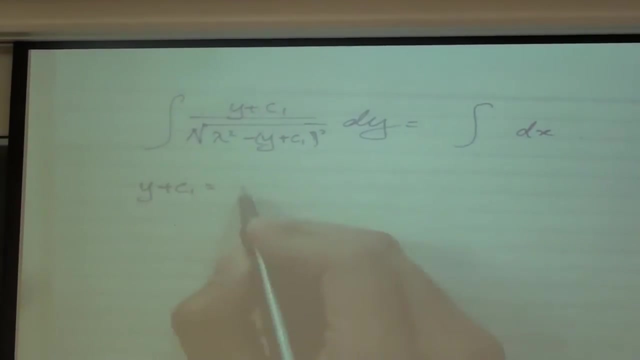 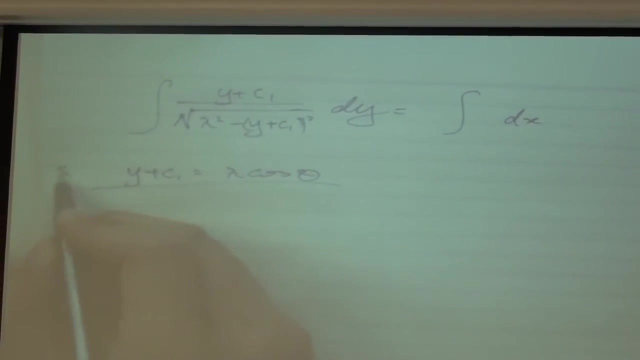 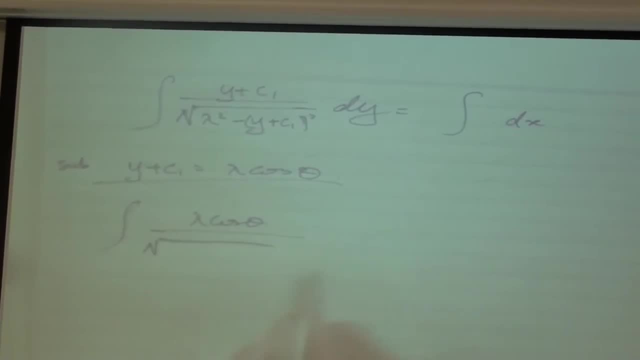 lambda cos theta divided by the bottom line is lambda square minus lambda square cos square theta. So by the trigonometric identity we have a basis for the square root: Lambda square sin square theta minus lambda sin theta v theta. 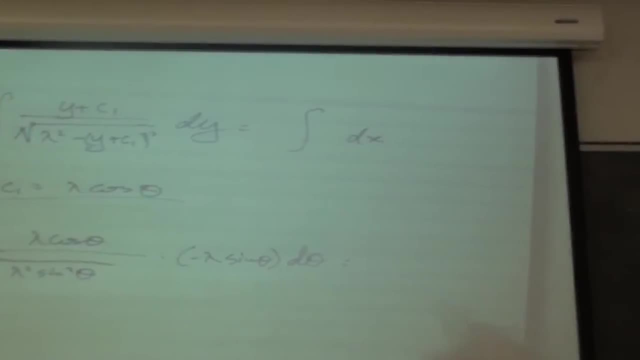 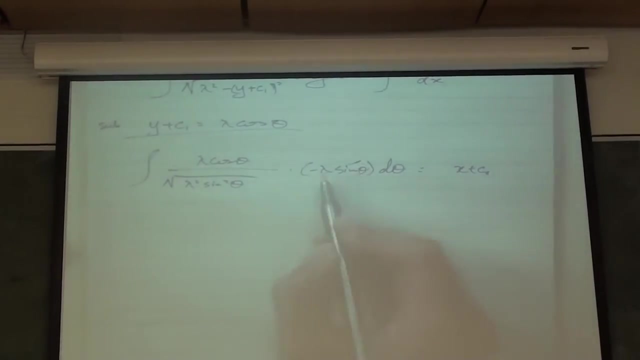 The right-hand side is really simple. right, Of course, that's x plus c2.. Okay, so of course you can see that there's a cancellation going on here- Lambda sin, theta, as I was denominated there, and you simply put the minus lambda out. 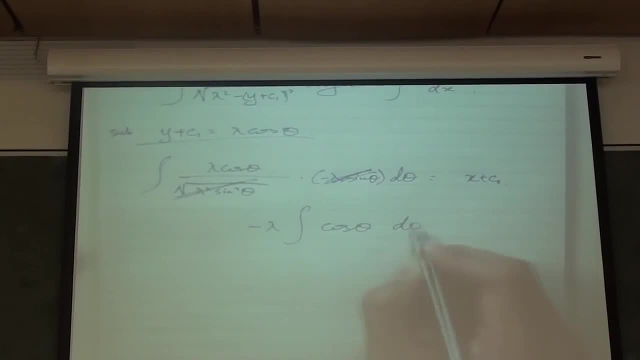 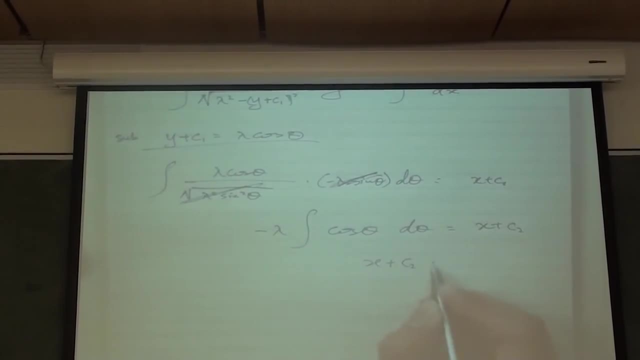 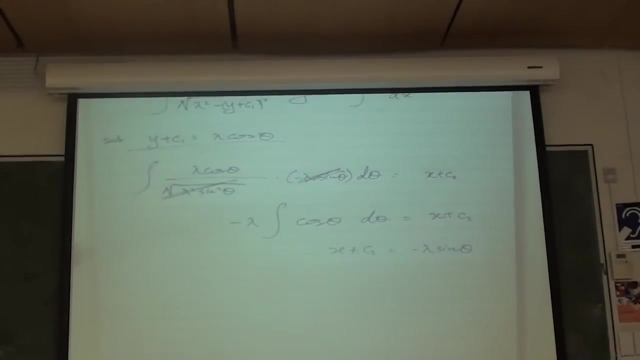 the left-hand side becomes integral cos: theta v, theta x plus c2.. So of course, we all know how to do this right, Minus lambda sin theta. Now here's an interesting point: It's that the author actually did this wrong. 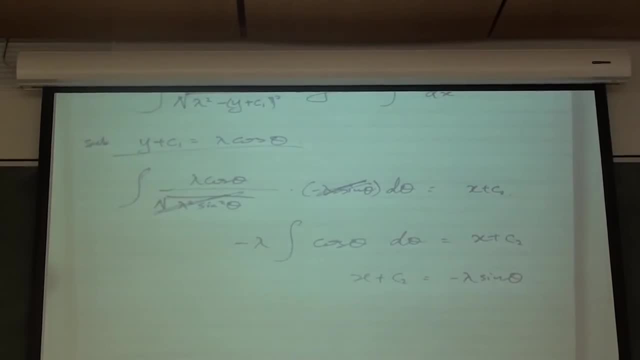 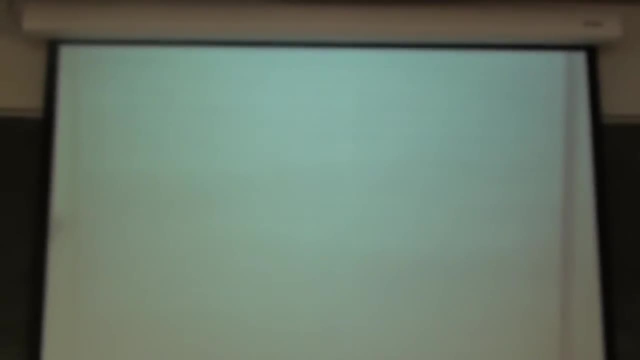 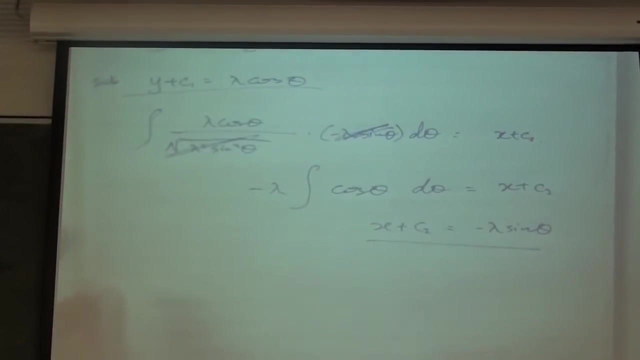 I don't know what happened, but that's what actually bugged me for a whole week. He actually did this wrong. Anyway, once I have that, we can actually write this two-parameterized equation again onto the next page, Because we'll actually be doing something really cool now. 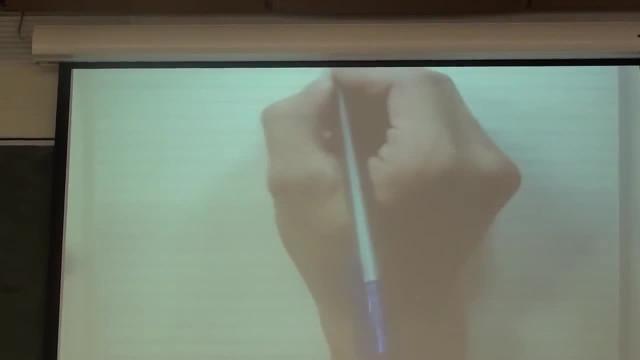 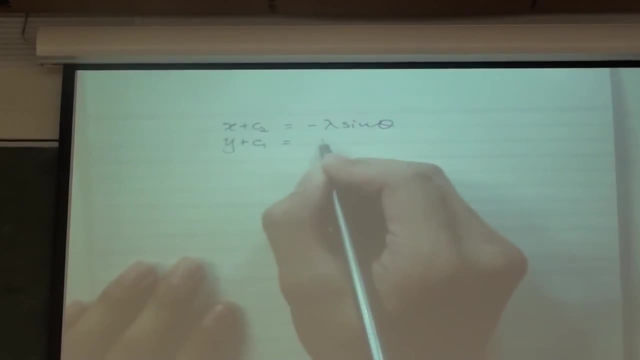 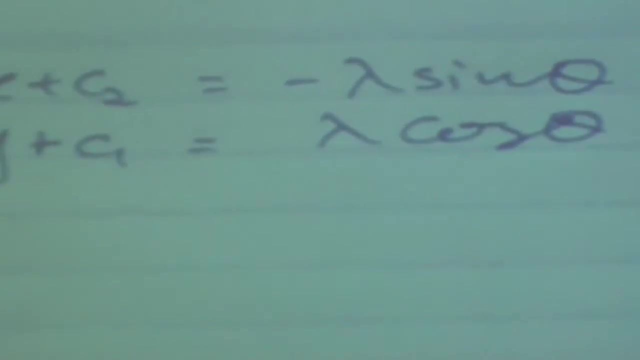 x plus c2 equals to minus lambda sin theta. Sorry, yeah, y plus c1 equals to lambda cos theta. So now what we want to do is to eliminate theta of these two equations, And the most natural way to do that is this: 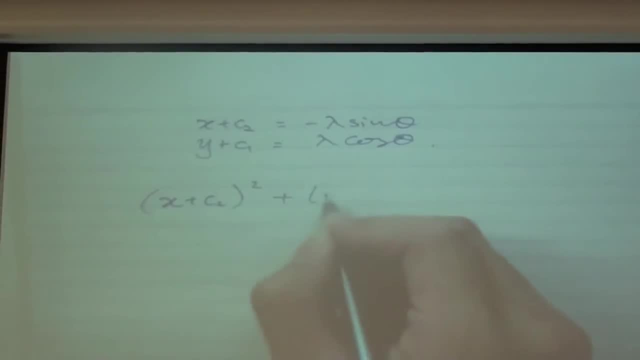 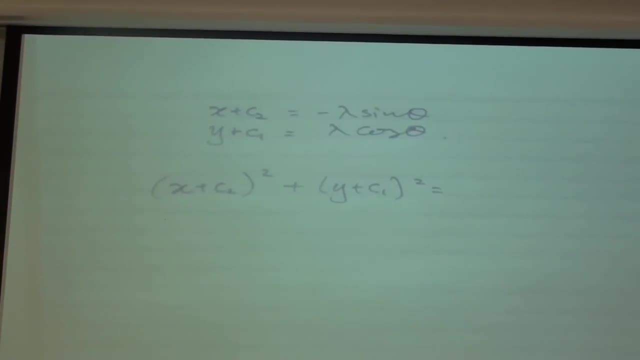 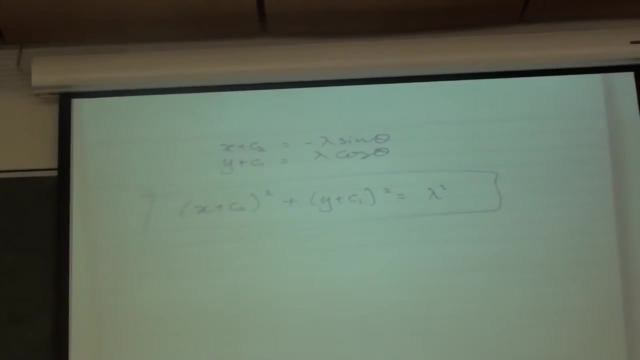 x plus c2.. Square plus y plus c1 squared Equals to lambda squared. But it's times by cos squared theta, sin squared theta. So that goes to zero. So it's minus theta minus squared theta. So lo and behold, we have an equation for a circle. 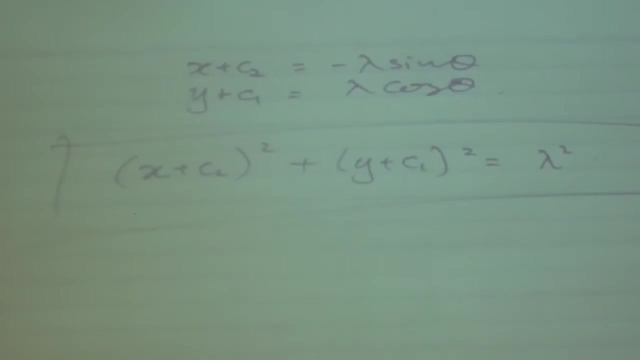 So now, essentially, you proved that you have this diagram: Between minus 1 and 1, the maximum area is going to be the arc of a circle. It's of a circle, but what circle? I mean, we're mathematicians. 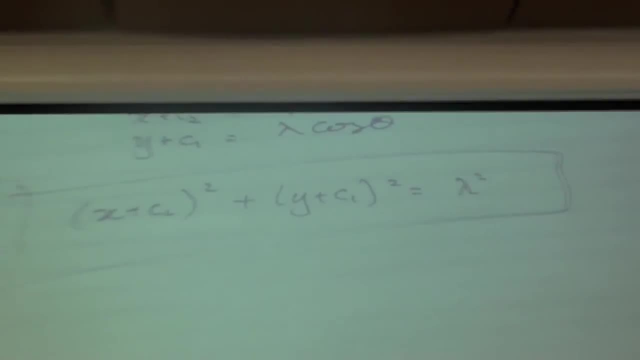 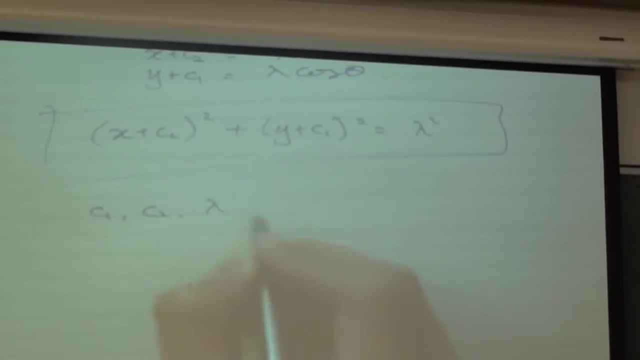 We're not satisfied with the answer of a circle. We want to actually find out exactly what is that circle. So to actually do that, we have to solve the constant c1,, c2, and lambda And to actually do that, or at least get an idea of how to do that, 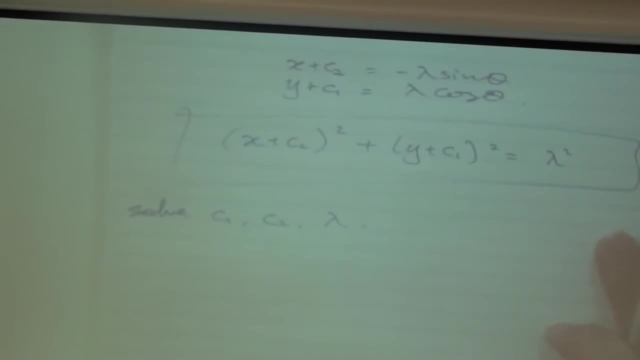 wait, let me just- it's a little bit hard to position this- We'll substitute these two, these two equations, into our isoparametric Mark-Lenz equation that we had before, And if I do that substitution, I claim L. 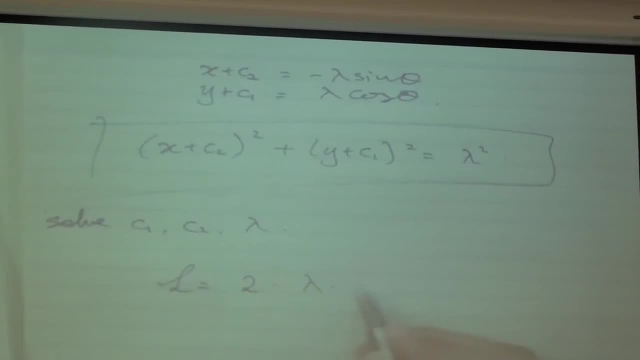 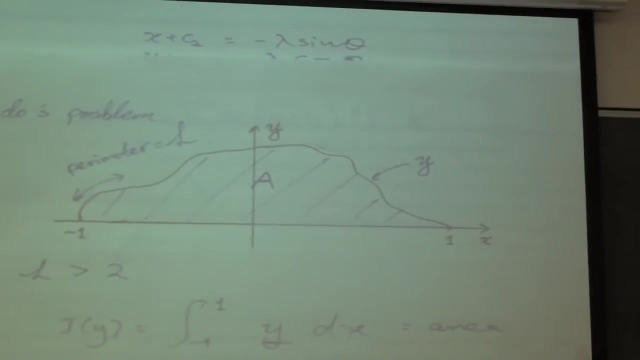 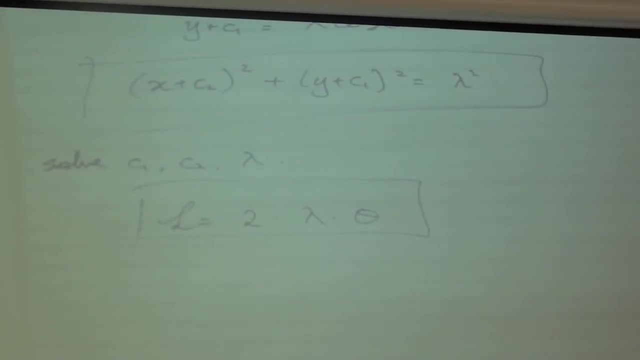 because of 2 times lambda, times theta. Now that's just a really straightforward integration that, if you're interested, of course you can try to do it at home. And now let's see what else we have Now. what we need now is the boundary condition. 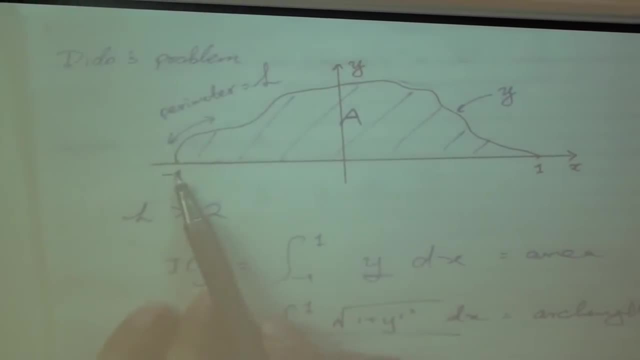 What I mean by boundary condition is that at x equals minus 1 and 1, y has a value of 0. So that's my boundary condition. So it's bound condition is: y minus 1 equals to y1 equal to 0.. 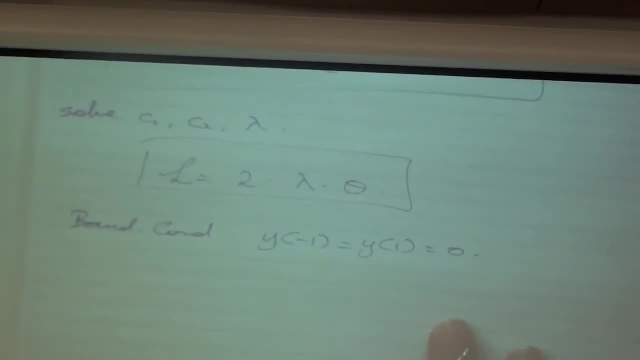 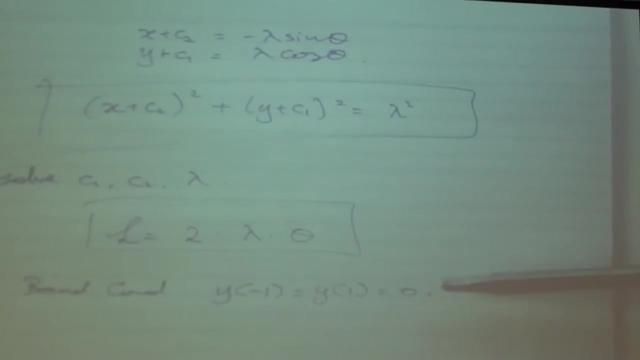 Now, once we have this boundary condition, what we could do is do a substitution, a substitute to these boundary conditions into the equation of the circle. And if you do that substitution, you see that c2 equals 0, and, in particular, 1 plus c1 squared. 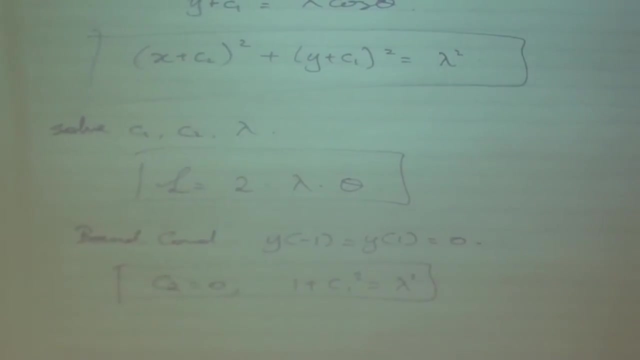 which is lambda squared. Now, of course that fits with our picture here, because if it's a circle it's symmetric and it must be centered around the y-axis, And that's why c2 equals 0.. That tells you it's the x-axis. 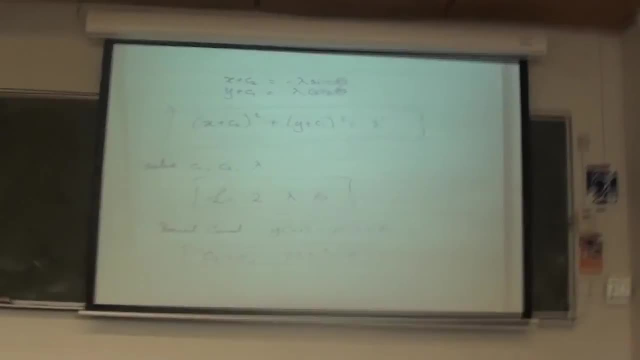 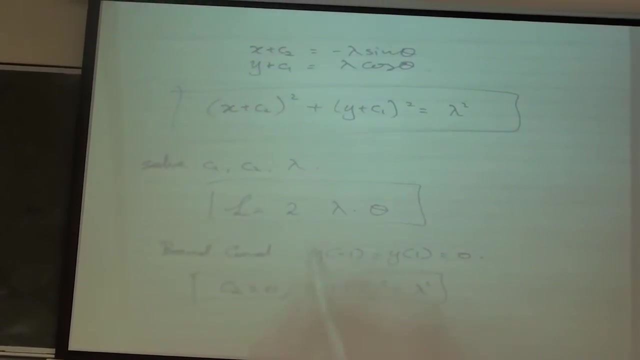 Oh, sorry, the y-axis. Well, once we have that, we can substitute the boundary condition into these two point-to-right equations. If we do that- and in particular I'm going to use this one- it's going to be minus 1 plus c2 equals to minus lambda. 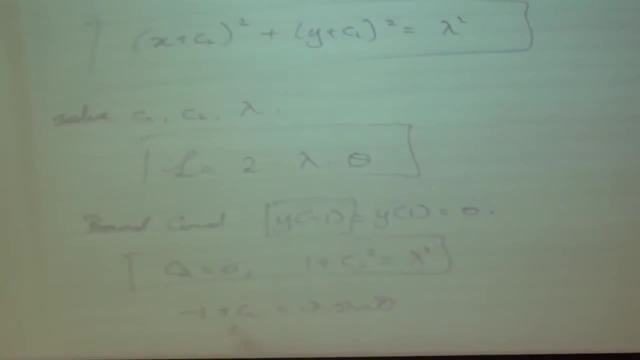 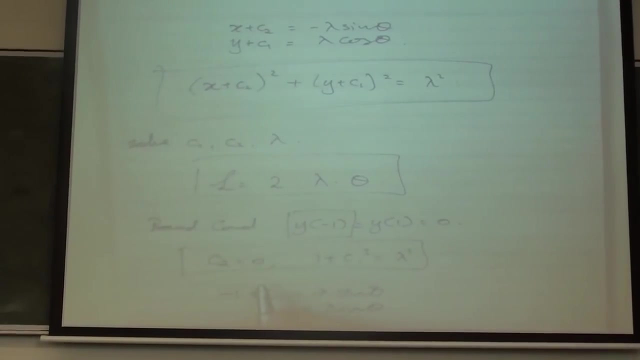 sine theta and y equals 0 plus c1 equals to lambda, equals theta. Now, of course, c2 is 0, as we calculated here. so that's 0. And if we do the division of these two lines, you can see that 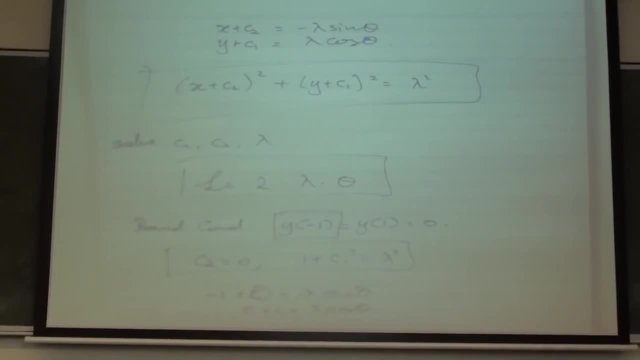 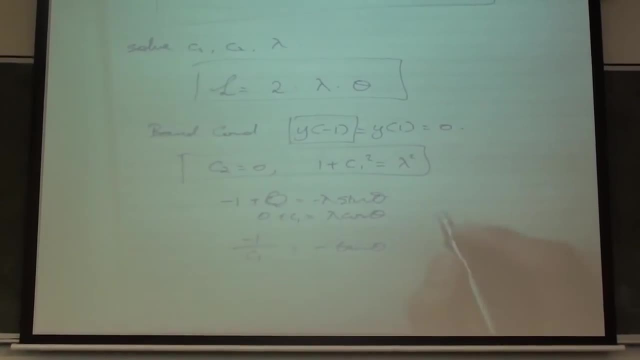 minus 1 over c1 equals to lambda. cancel out. so that's going to be 10 theta. Oh sorry, Yeah, it's a little bit hard to see. yeah, Okay, so once we have these, of course the negative sign, cancel each other out. 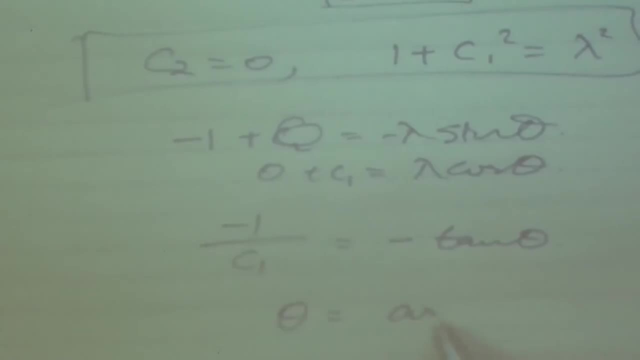 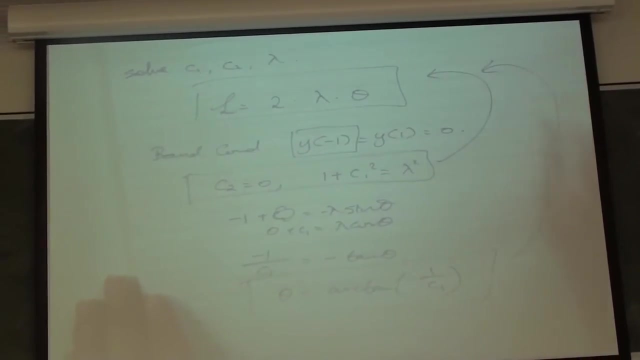 so we're just simply left with: theta equals to the arc 10 of 1 over c1.. So here we have to go to theta and this equals. we have this equation here, and what we do now is to substitute this back. 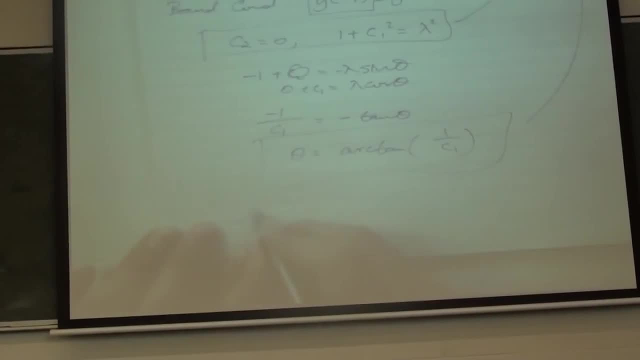 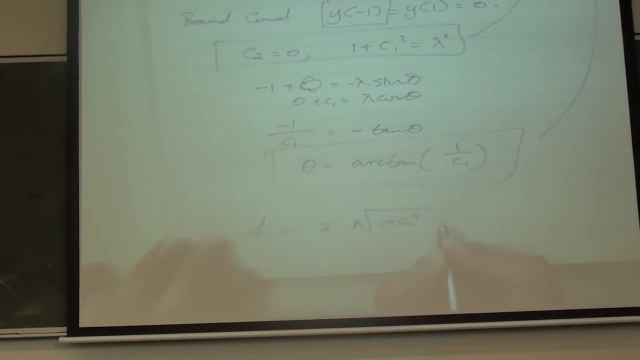 If we do that substitution, I claim that. well, not claim. you can see that 2 times lambda, but lambda is the square root. Okay, take the square root of both sides times the arc 10 of 1 over c1.. 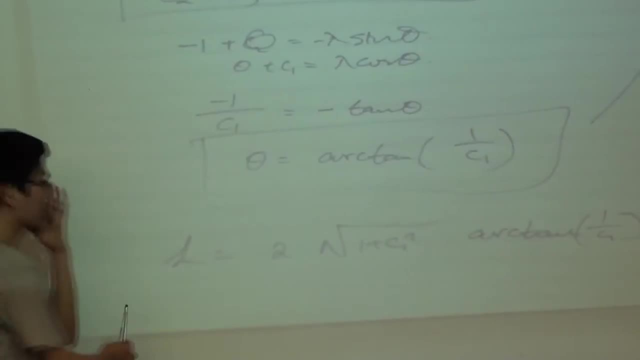 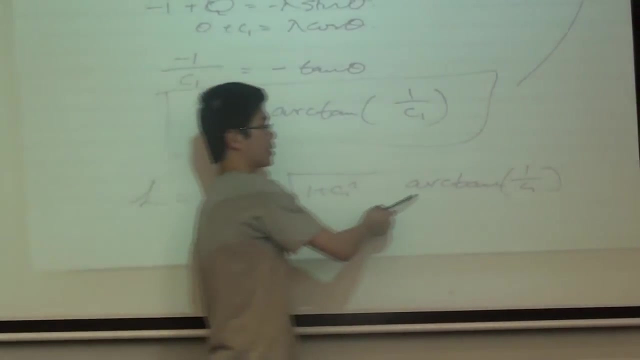 And here's why I would like to take a moment and think about this, right, Because now, once I have this equation, if you actually give me an L now, I can substitute L into this and it will help me with c1 numerically. 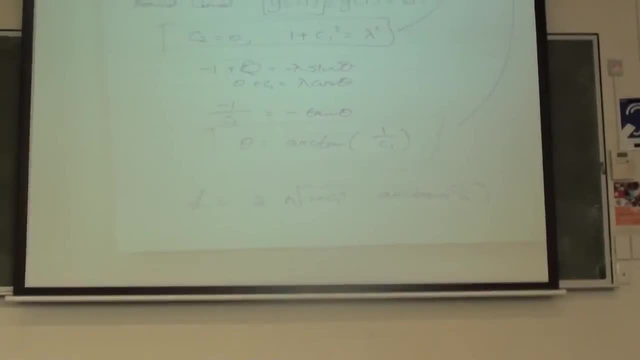 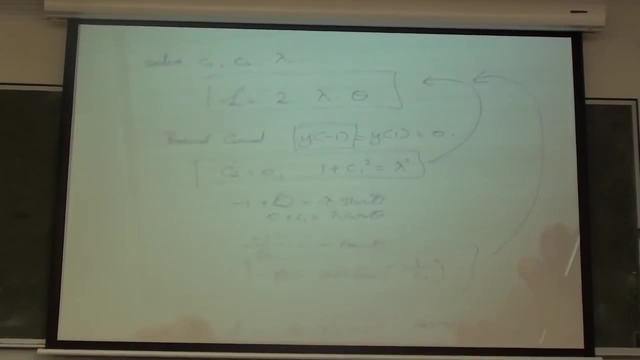 And of course I have to use a numerical method because there's no easy formula for arc 10.. So once I have that right, what happens? is this The equation of the circle, if you just substitute those conditions back, especially that c2 equals 0,? 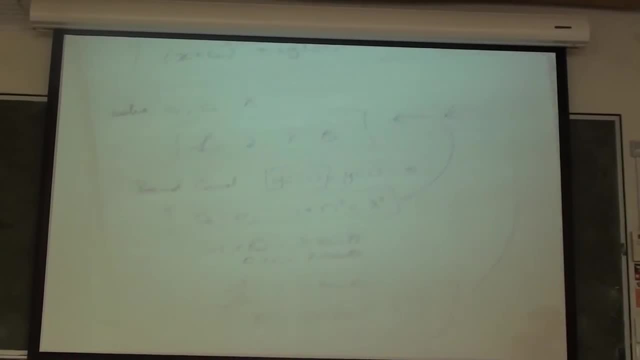 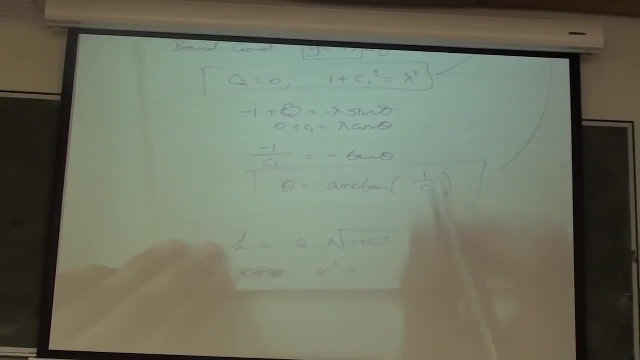 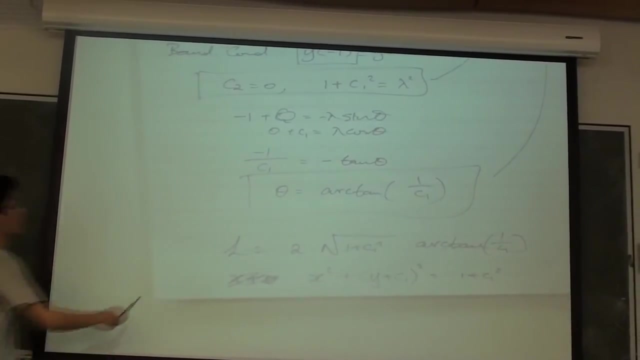 and I'll rewrite lambda. this way, you will actually get x plus 0.. Let me write it again: x squared plus 1 plus c1 squared equals 1 plus c1 squared. So, as I mentioned before, if you give me an L now, 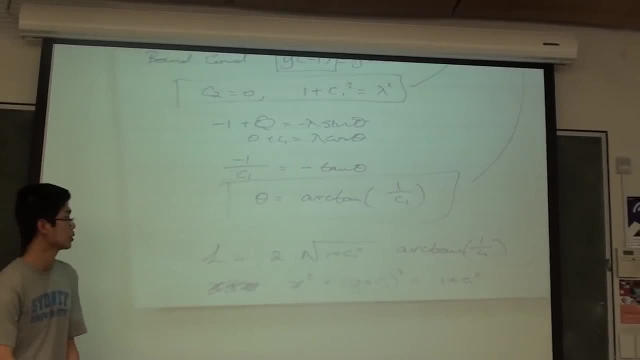 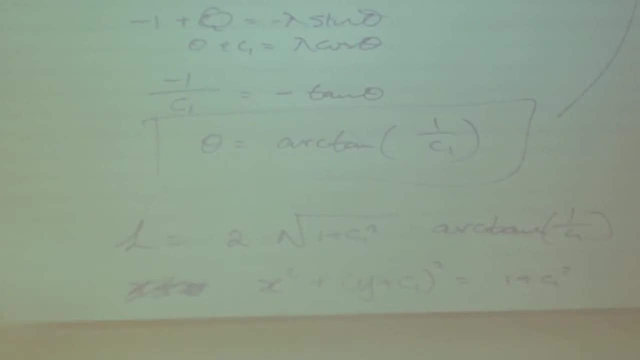 I can solve c1 numerically And once I have the numerical solution, I can carry precisely where is that circle, And that's actually finished my whole problem. well, almost, Because in actual fact this is a really nice diagram. It actually shows you that you can. 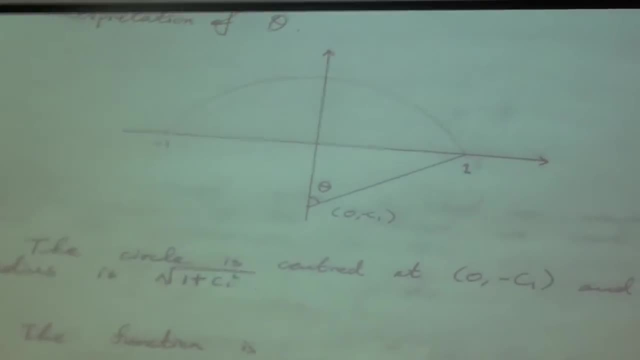 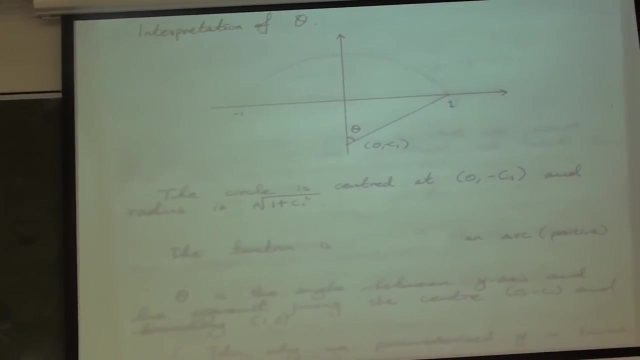 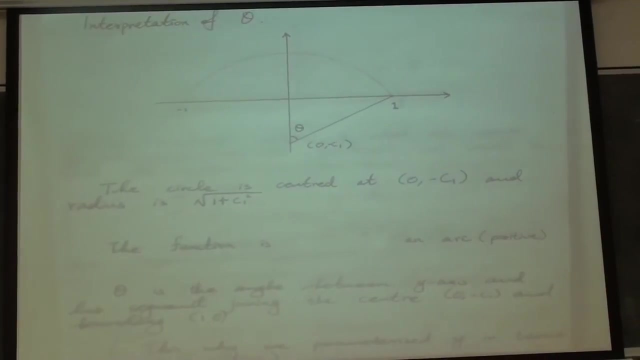 Why is this intuitive? You have this. What You fix a lamp, don't you? Okay, okay, I understand you. You can imagine that I can move this arc up and down And if c1 actually coincides with the origin, 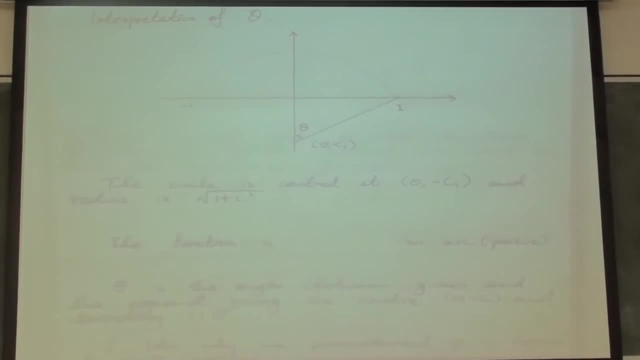 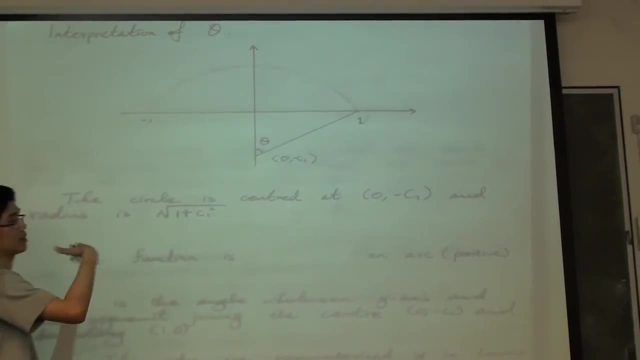 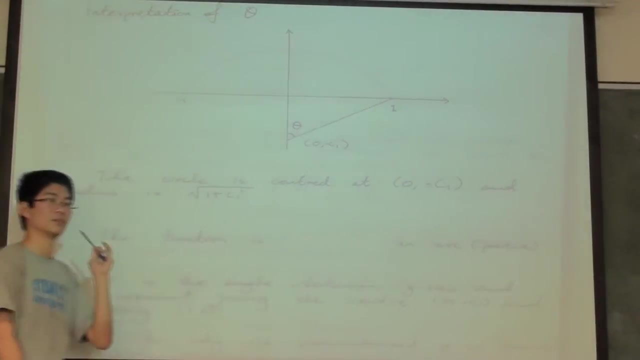 then we'll actually get the semi-unit circle. And once we get c1, if c1 equals to 0, and you get a semi-unit circle, then you can perhaps make a symmetry argument and say, well, what's above, that is a maximum. 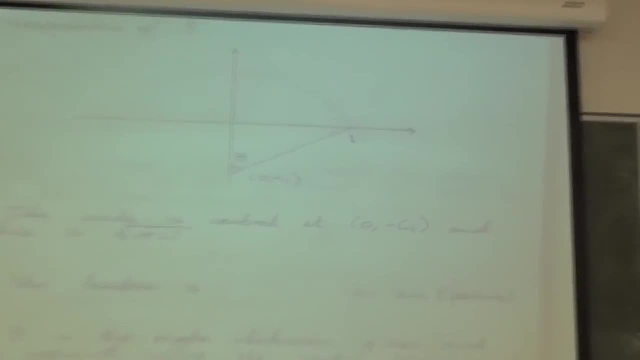 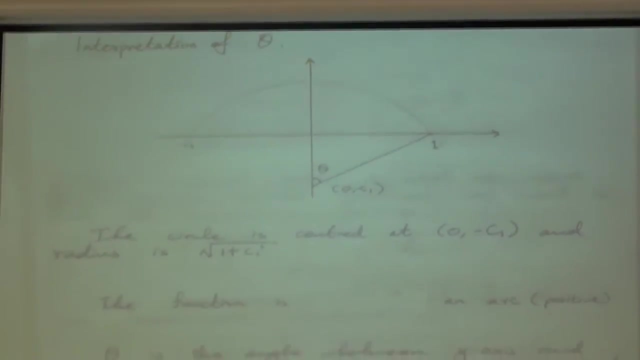 because I've just shown that What's below that? because it's symmetric, you can actually make that same claim that that's going to be maximum if it's reflected. So overall you can sort of make that symmetry argument that this is going to be the maximum area. 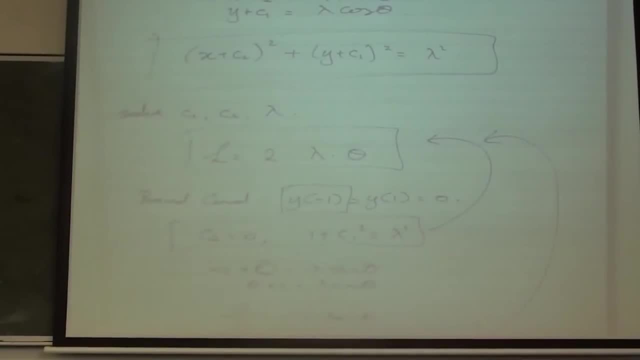 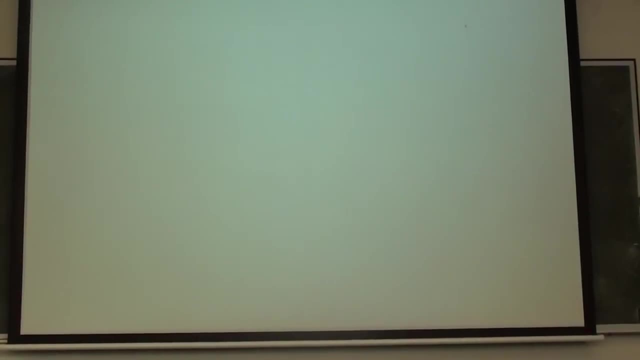 Now, of course that's a little bit dodgy, because I, Because I don't know if my solution is a maximum or minimum, But let's just summarize that. Summarize, Ah, show and tell, right, Sorry, show it here. 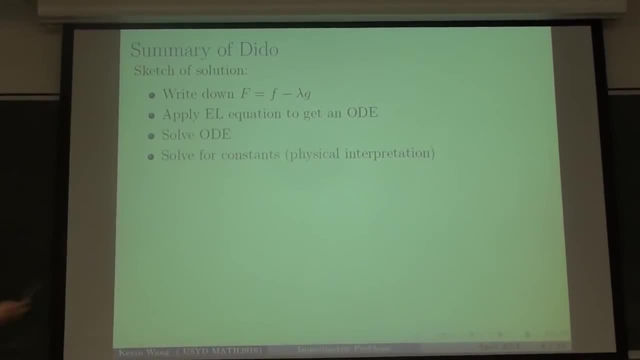 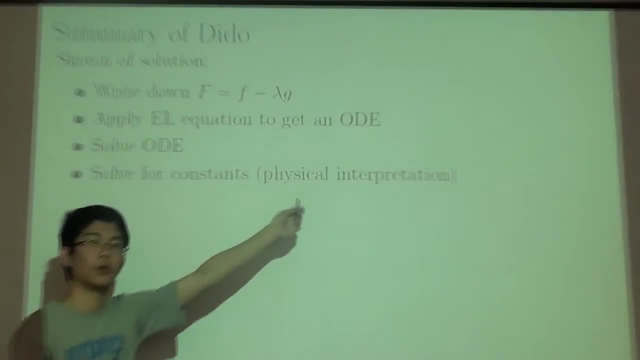 So let's summarize what we did first, and then we'll look at the maximum problem. So here's our solution. We'll actually write down our function capital at first, and then we'll apply it to all of the large equations to get an ordinary differential equation. 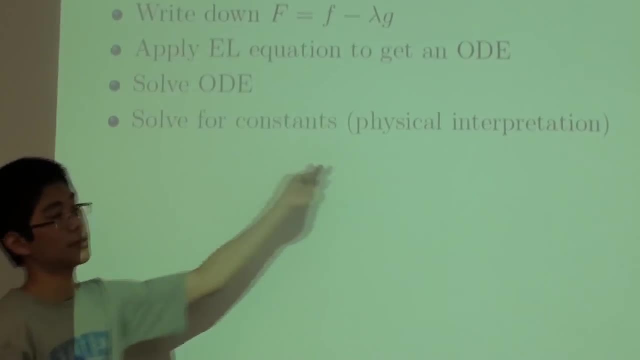 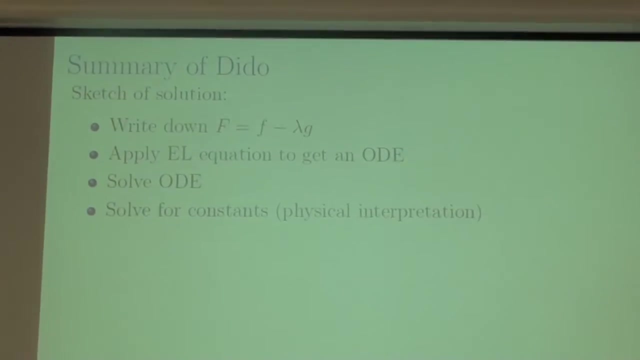 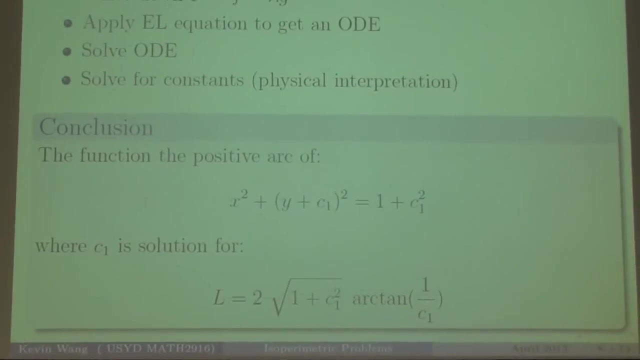 And then we'll solve that differential equation and then we'll solve the constants. So this is the four steps, That's all. our solution is about doing these four steps and then understanding what is the constant. And here's our conclusion, written out nicely in LaTeX: 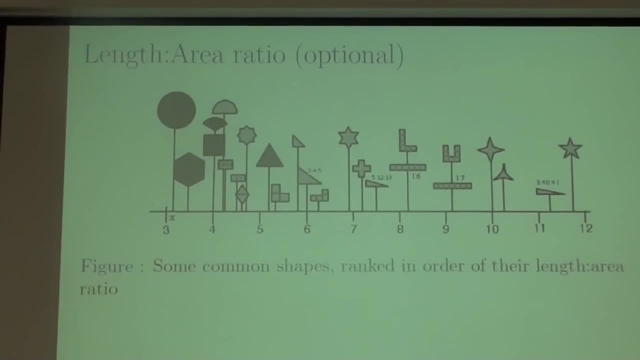 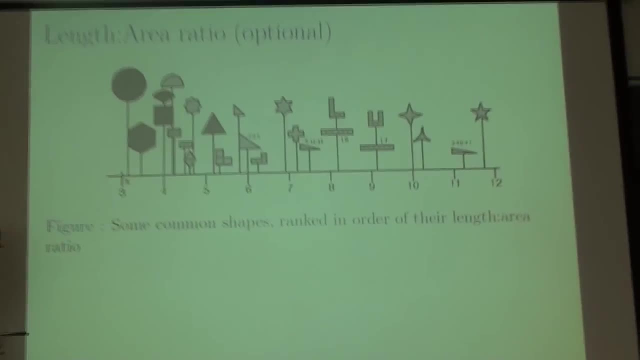 Not LaTeX. So here I mentioned before that I don't know if my circle is a maximum or minimum or some other critical points, but hopefully I can convince you with this rank of diagrams. Now, all of these diagrams, all of those shapes. 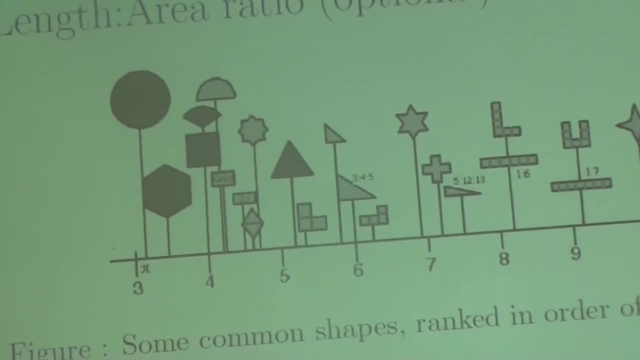 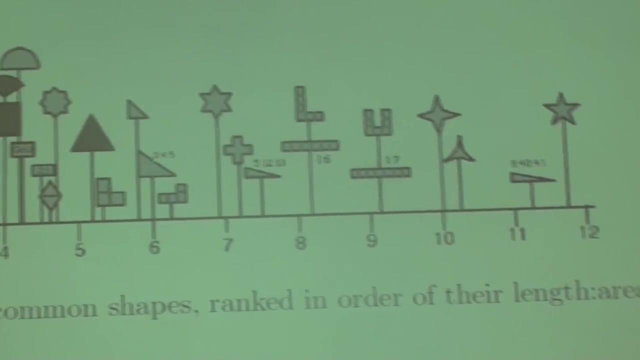 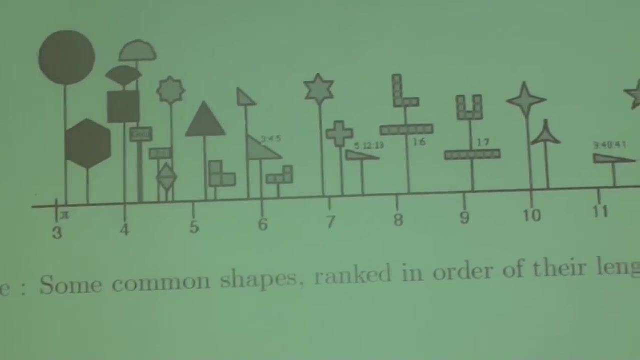 they are right in the length-area ratio, But that I mean circle has the maximum among all of those shapes, most common shapes you have in real life Common, Ah, that's a little bit of lollipop, isn't it? 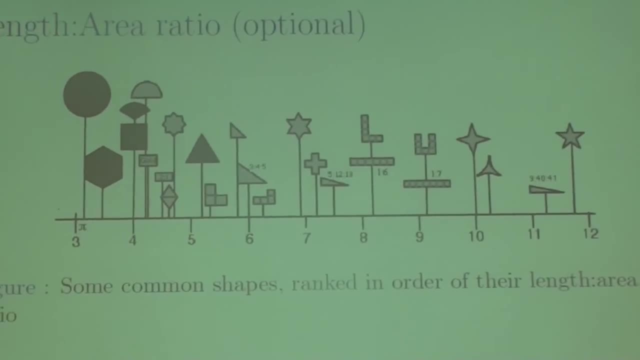 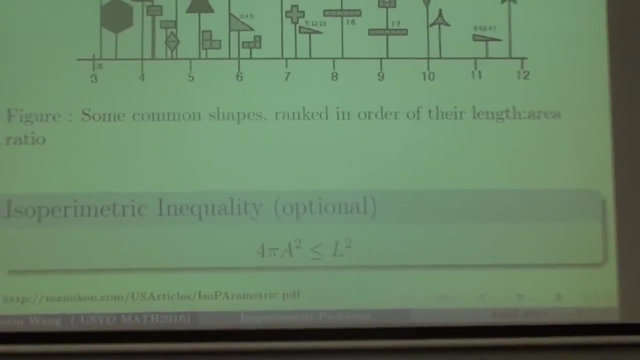 So hopefully I can at least convince you that circle is not a minimum among all of our common shapes in life. But of course, to address that, to address that more precisely, perhaps this is where stick and variations come from. Now, the iso-parametric inequality. 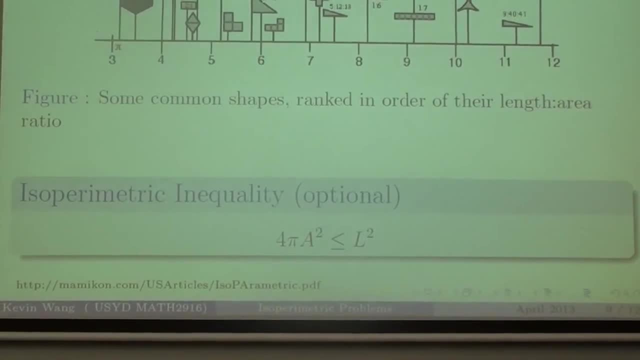 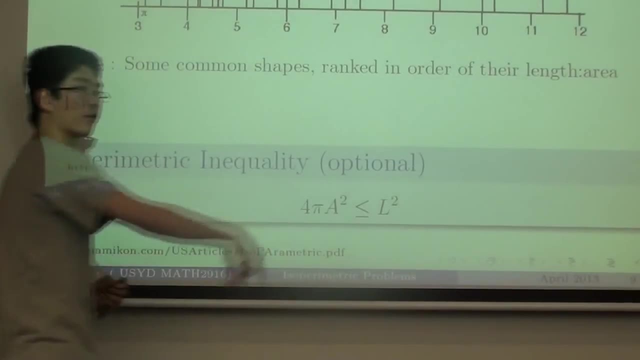 which is definitely known in your book- I mean in the von Braun group- is that you have this intron equation that if L is the parameter of your curve and A is the area of that, this equation always holds in two dimensions. 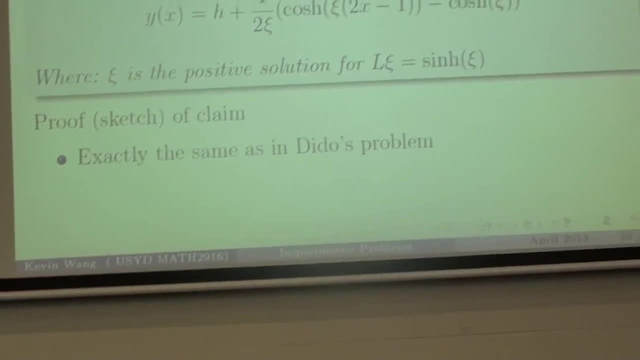 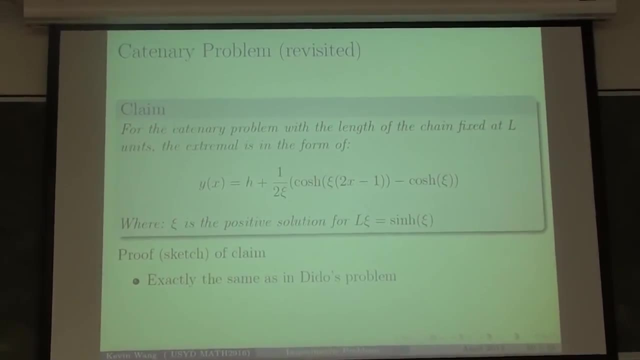 And that's quite cool. And this is just for Daniel, because he was asking about the ordinary problem last week and I just put it here and showed it. This is actually the solution. Of course that's really messy, but the idea of actually proving the claims- 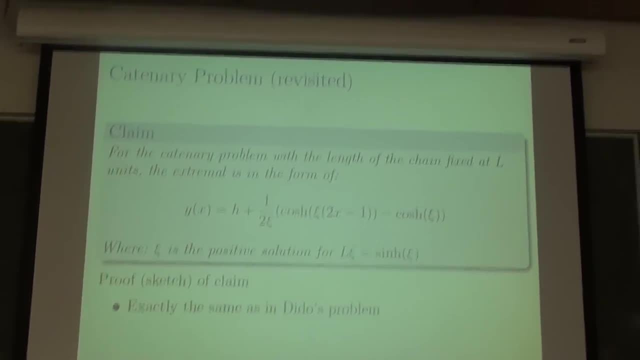 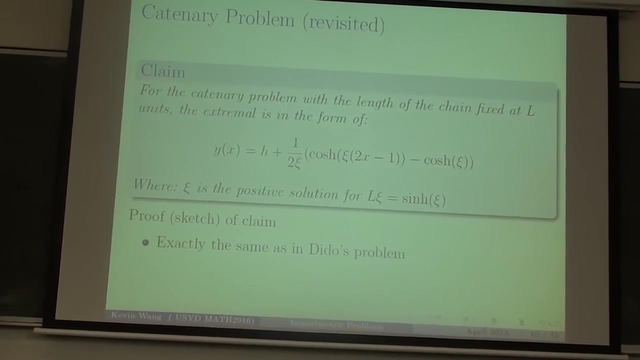 is exactly the same as in the Dino's problem. It formed with the capital-N function and then you apply the Euler-Lawrence equation. Once you did that, you solve the ordinary differential equation and you just get a constant at n. 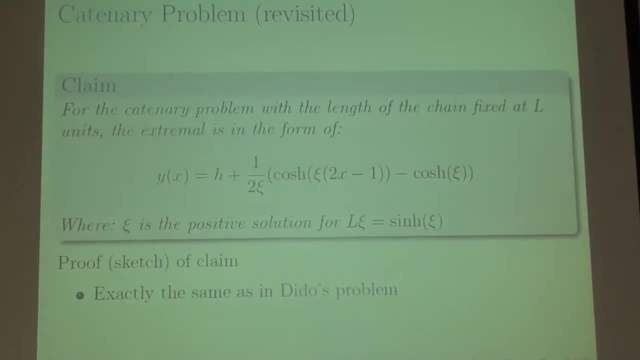 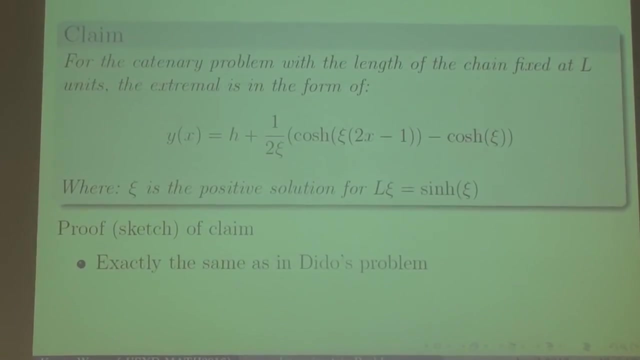 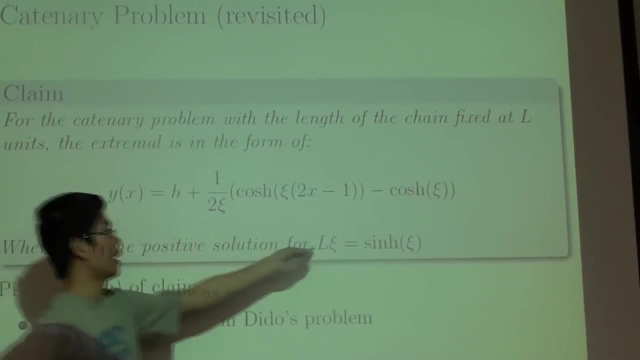 You solve the constant at n And of course this has some solution, but that could be very difficult to calculate. So again, computational solution housing- And you can probably notice that that's exactly what Will had before- is that he cannot make the claim that 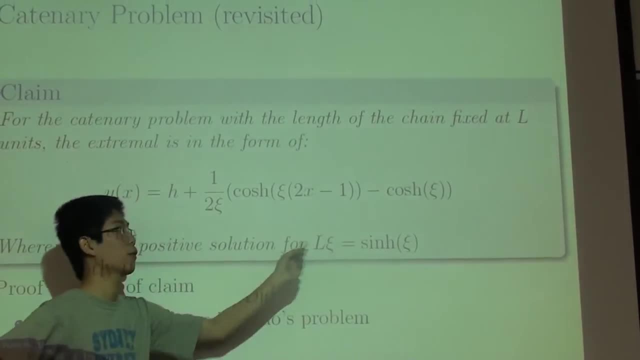 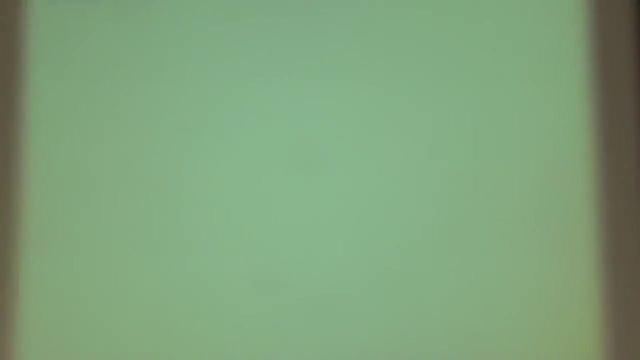 this C, Greek letter C, if that's 0, of course these will hold, but that would be a meaningless problem because L equals 0. So here we'll have this problem here and now. I'm trying to relate this back to the bottom of the map. 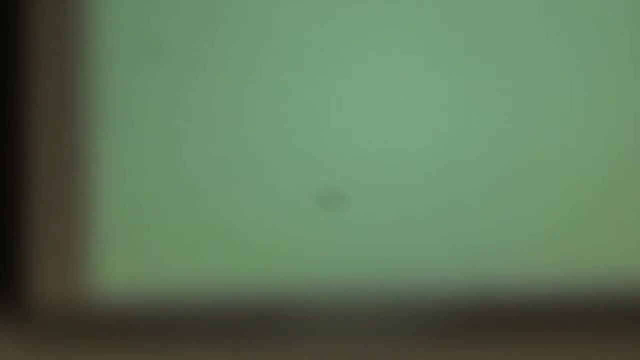 I'm almost finished the slide, sorry With Landau. Now Landau, as I mentioned before, is called the Lavoisier multiplier, is the actual constant itself. Now, if you think about constants- and this is what I struggled with- 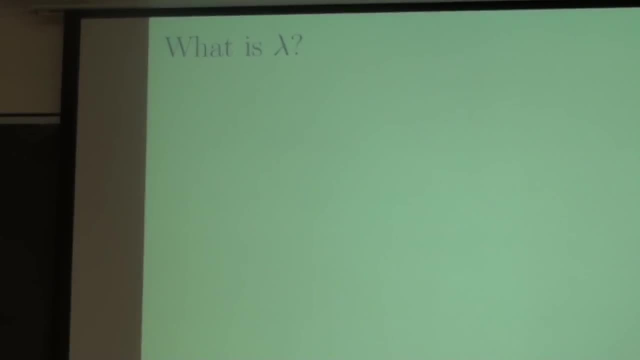 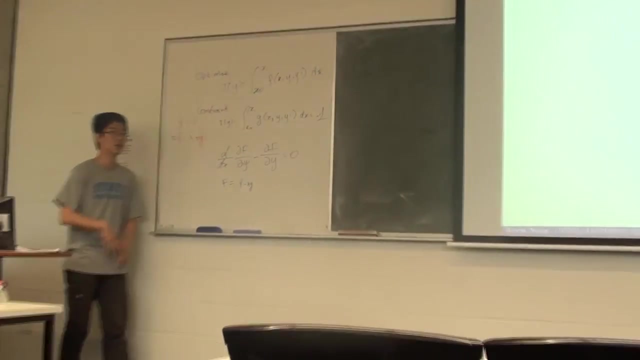 during my research of the topic is that I would think about Landau as some sort of mathematical constant that actually is there to make your equation work, or some sort of physical constant like that we've seen in the Dino's problem. It has a physical meaning. 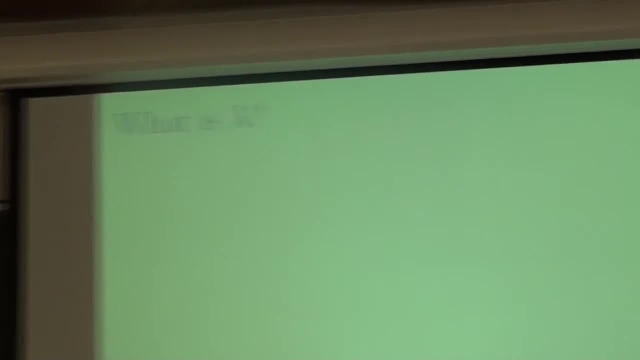 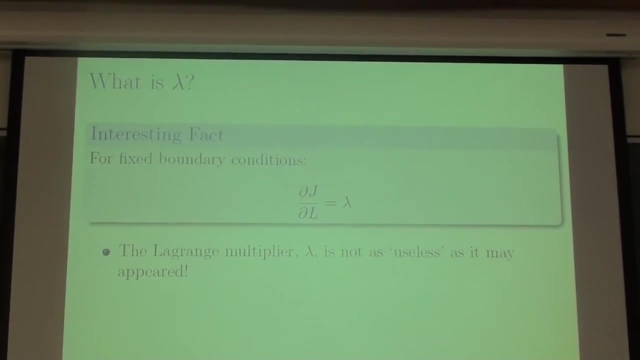 But the Lavoisier multiplier, it was literally deeper than that. Now, if you actually have fixed boundary conditions, this equation always holds. If you take a partial of J with respect to a partial of L, this equation will always hold. 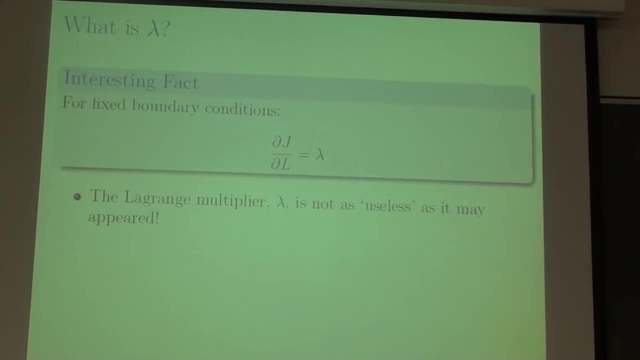 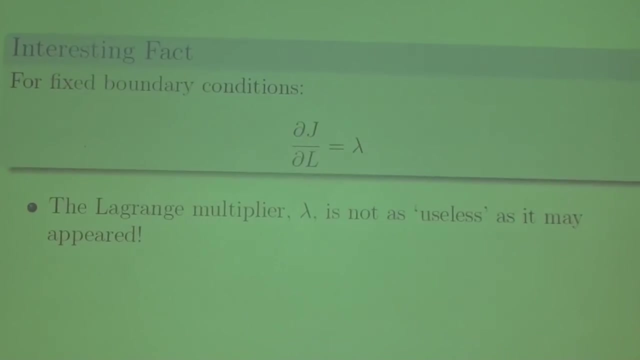 And that equals to the Lavoisier multiplier, And that, I think, is probably surprising for me while I was doing this, because I didn't know that what's the actual meaning of the length of the constant Landau? And, of course, I just want to quickly mention that. 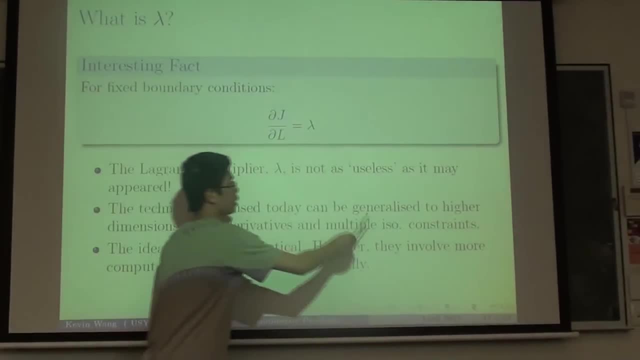 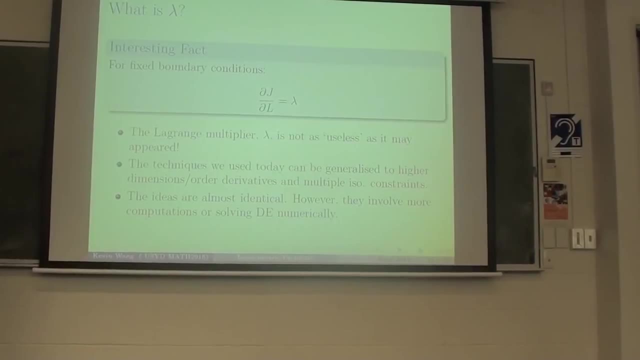 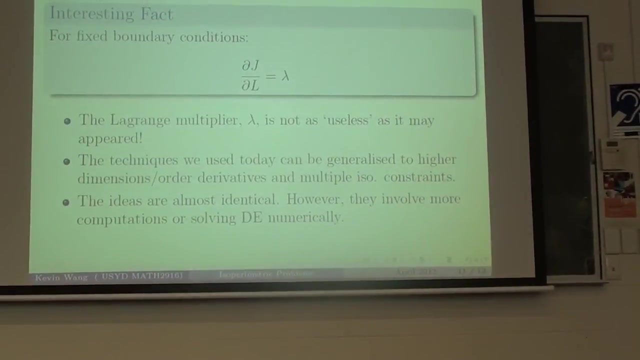 the techniques we use today in the Dino's problem are actually applied and generalized into higher dimensions or higher derivatives or in multiple isometric constraints. Of course, that is what Maggie covered last week about using Lavoisier multipliers in higher dimensions and higher order derivatives. 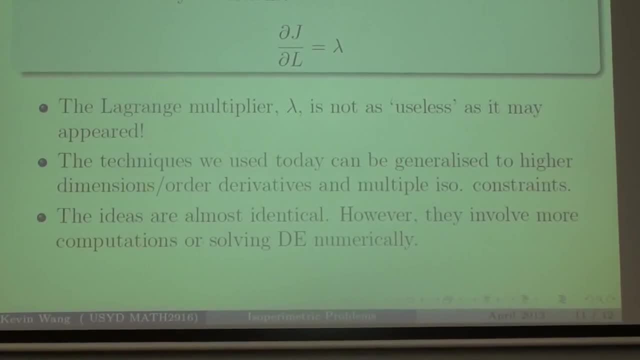 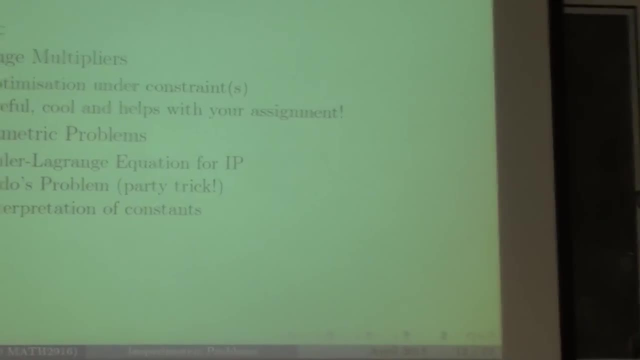 And you do exactly the same thing and the function you're going to apply on is actually this capital F game And of course, there's more computation. So here I actually finished my talk, and the concluding remark is that Lavoisier multipliers optimize each other constraint. 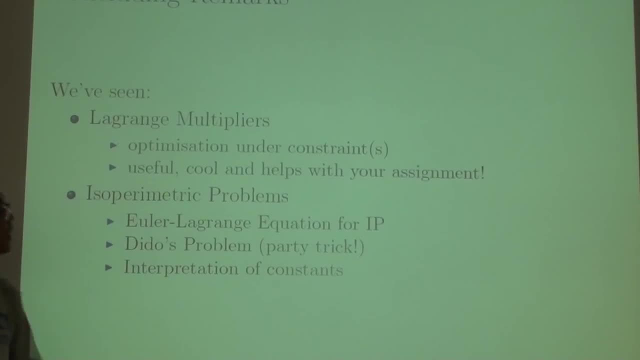 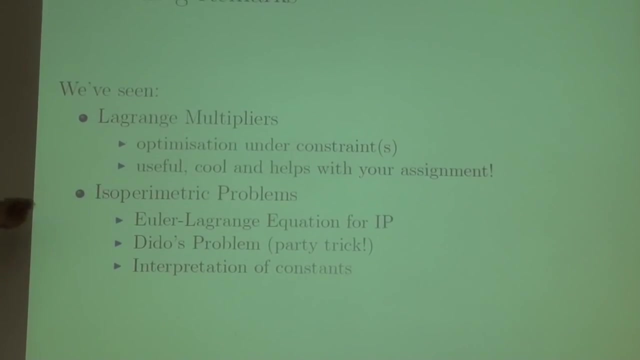 and it's useful, cool and helps with assignment. One thing that I should have probably just probably glossed over is that this is not going to be the last time you're going to see Lavoisier multipliers in your life, in your mathematical career. 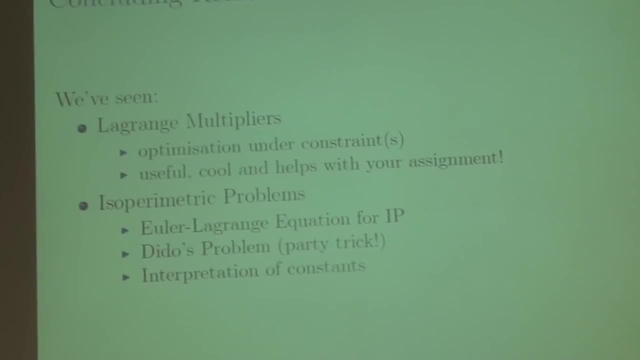 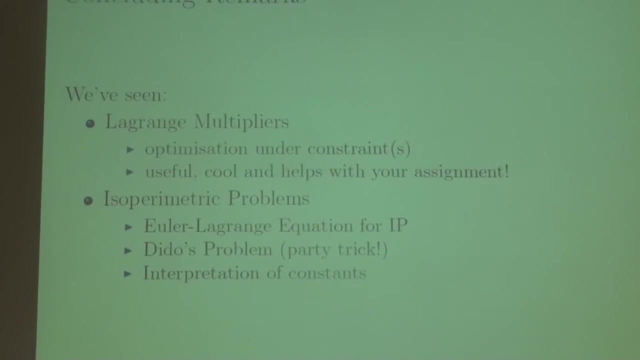 It's probably going to pop up somewhere in your life later. And, of course, you know the Lavoisier equation for IP, which is this: that's a cool equation and the Dino's problem. show that to your friend next time. 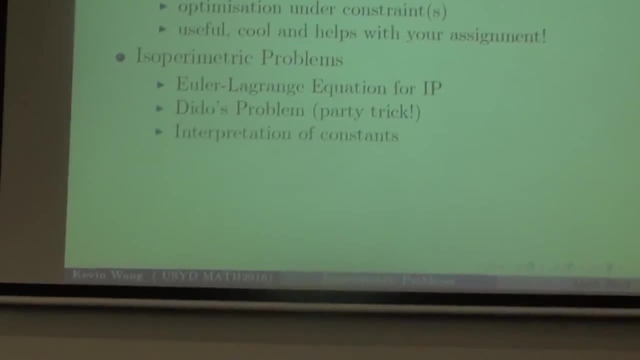 you're partying and you have to deliver the confidence in this. So yeah, here's my talk, Thank you.